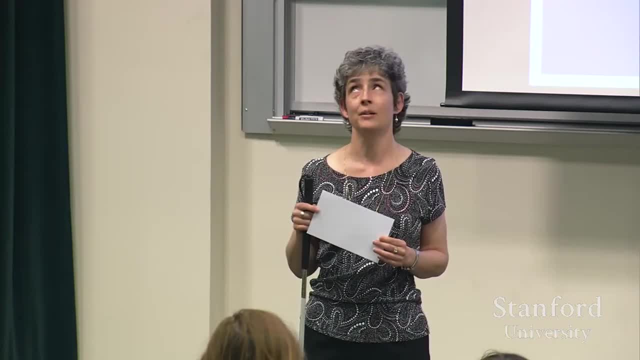 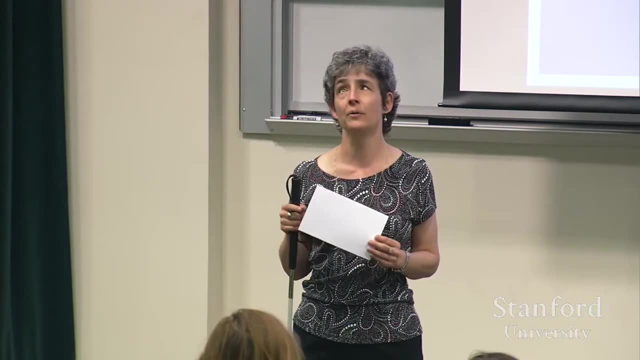 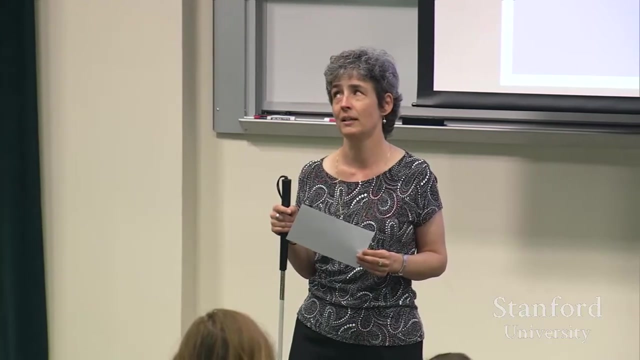 on. it's called WCAG for short. You may hear people pronounce it differently, but WCAG- mostly people know what you mean. WCAG 2.0, and we focus on the AA criteria. I'm not going to launch into any discussion of those criteria, what they mean, but the short version to think. 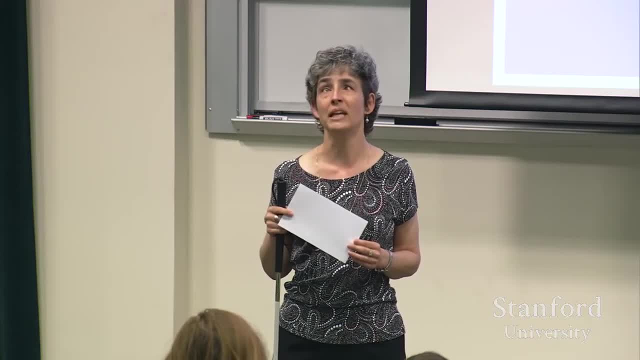 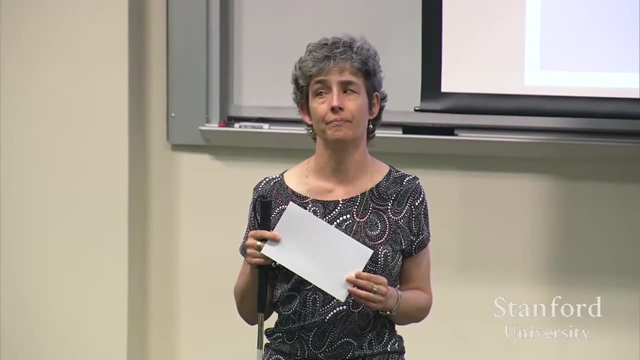 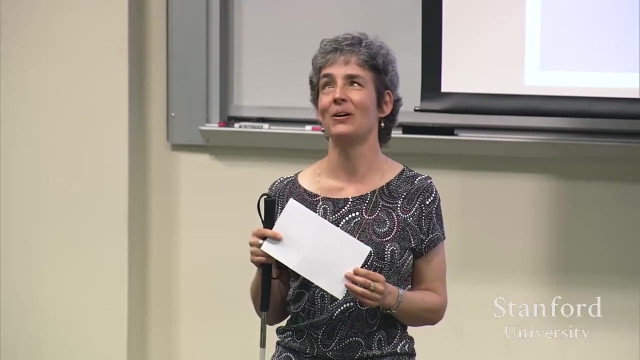 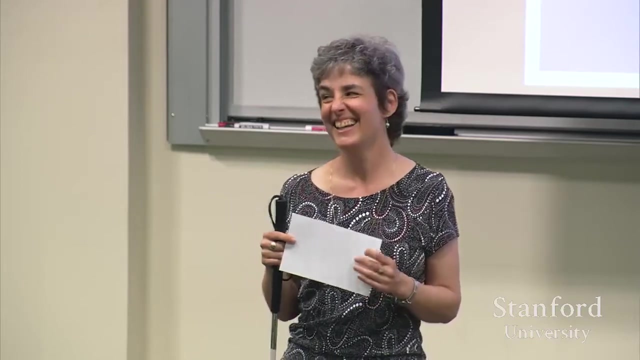 about when you think about WCAG. is POUR, P-O-U-R Perceivable, Perceivable, I'm not going to go into that. Perceivable, Operable, Understandable, Thank you. Understandable and robust. Was that my colleague there, Judy in the back? Yeah hi, So anyway, those are. 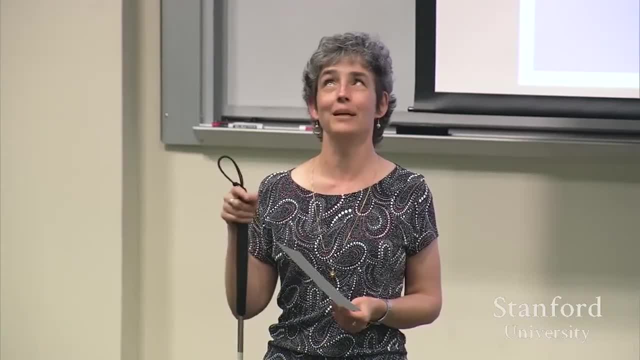 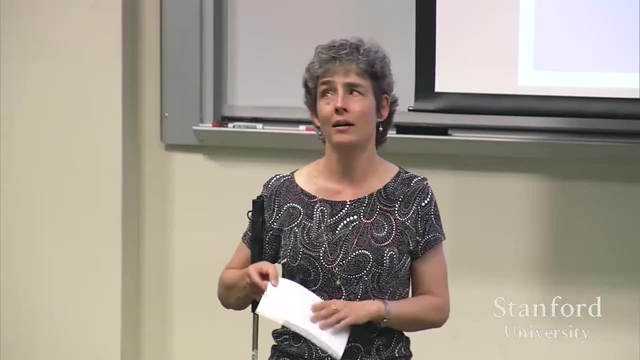 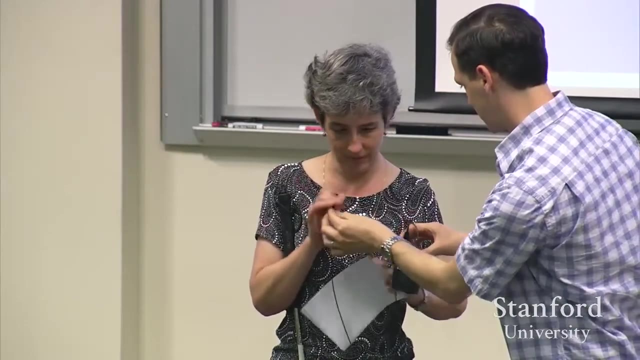 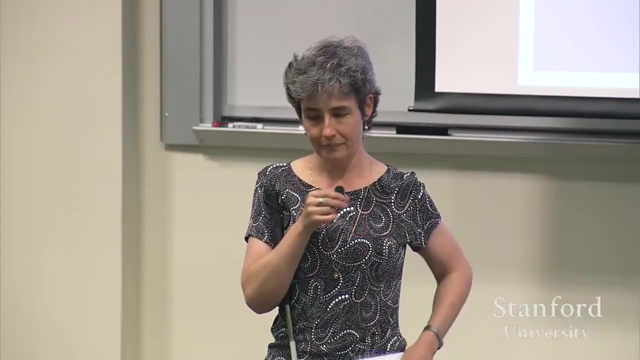 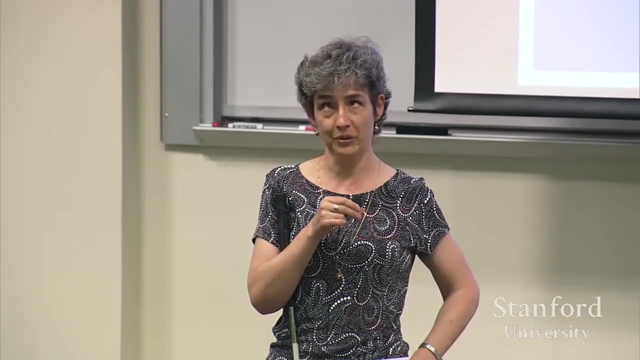 the four criteria. I don't actually think about them that way very often because I kind of know them back and forth, So that's why I'm a little caught short. So I work with on assessing, I work on assessing websites and I also am building, and it is a journey. 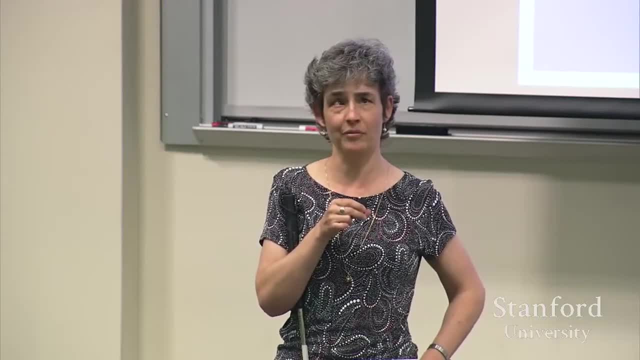 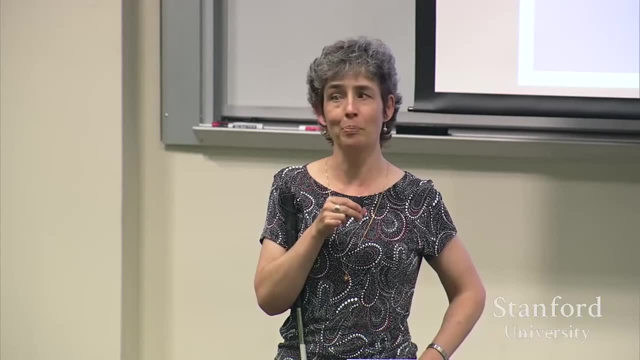 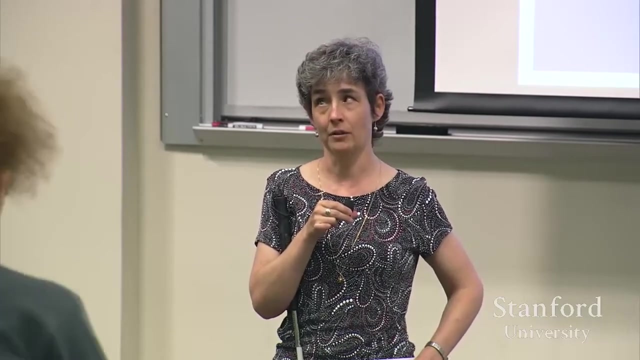 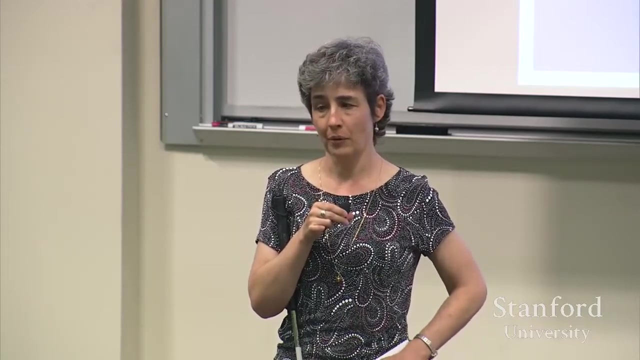 to build a website for the Stanford Online Accessibility Program And we call that here SOAP, So it's soapstanfordedu, And you're welcome to take a look around, and the content will be growing as fast as I can write it and get it posted. So that's pretty much the. 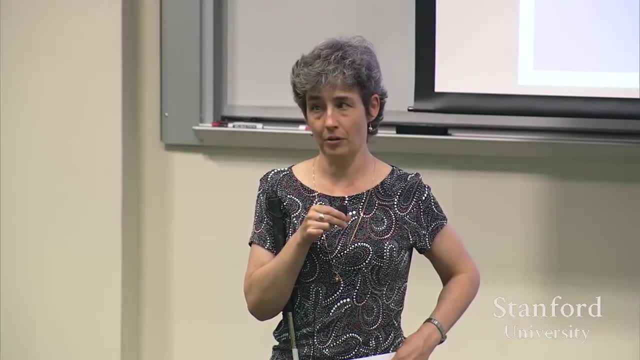 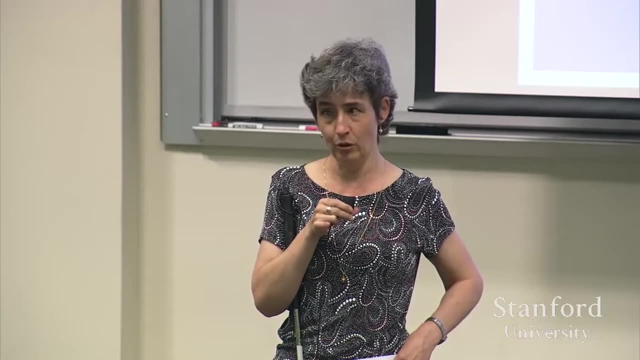 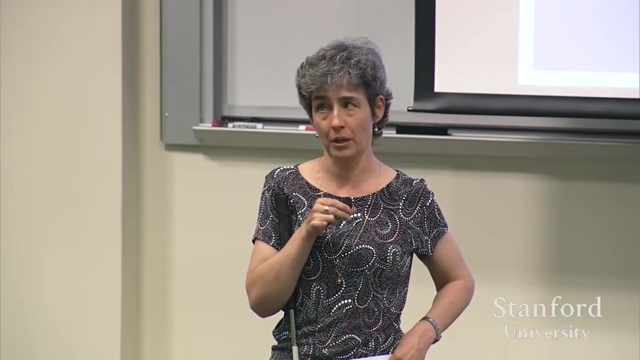 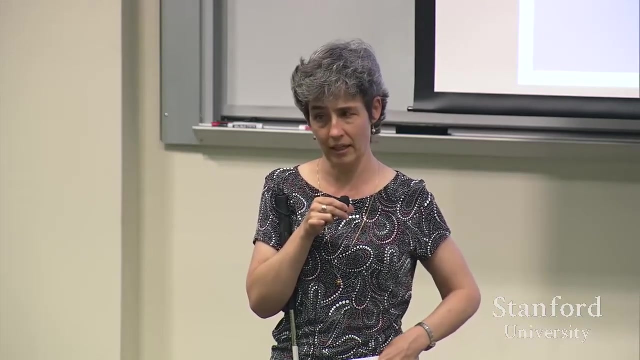 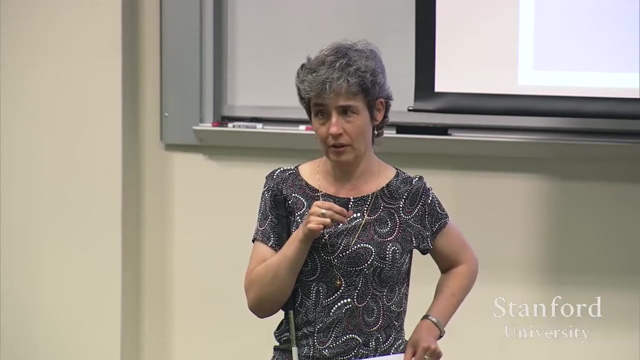 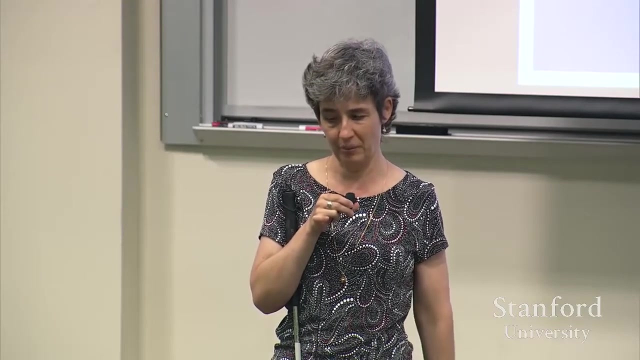 work that I'm doing For those that are students here at Stanford, there's a different office that would be available to help you, So that's the Office of Accessibility Education. So there's sort of the website aspect of it, and then there's more the assistive technology aspect of things. 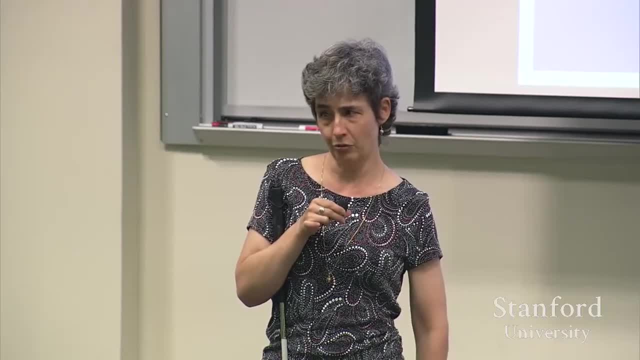 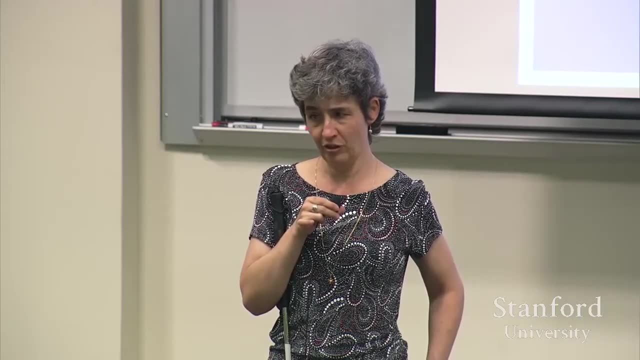 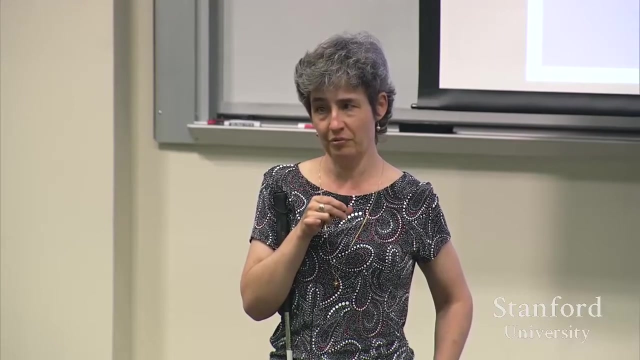 So I just want to give you a bit of a rundown, bit of an orientation of what we're doing here at Stanford. I have just: my job has just expanded. I've become a Stanford staff member as opposed to a contractor, So I'm just getting myself revved up here. That just. 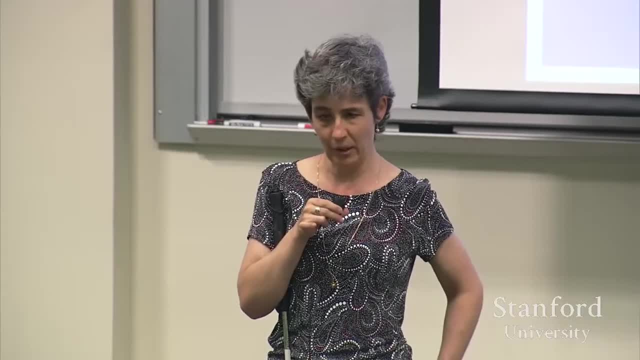 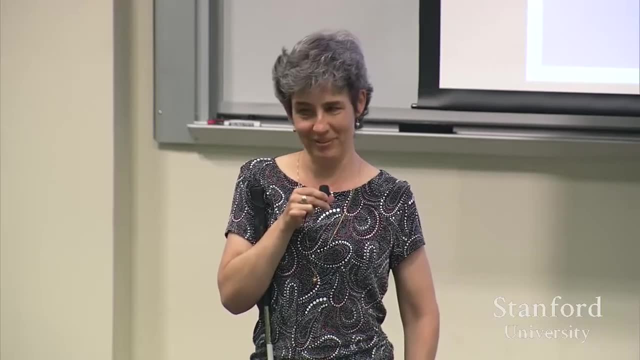 happened in the last two weeks. So I've got my work cut out for me. We've got plenty to do. I have no concern, frankly, about job security. There are lots of work to do. I'm trying to have a better job. I'm trying to keep up with the data that's coming in, which. 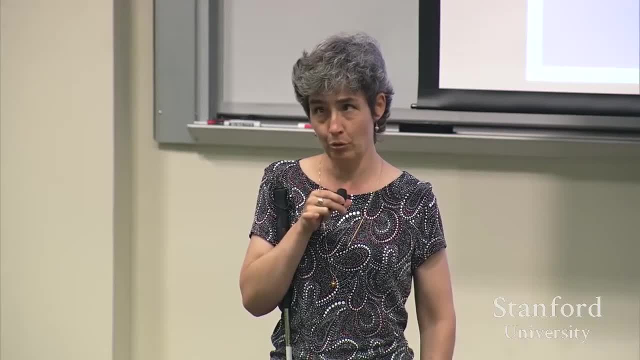 is still pretty good, But my job is probably going to change with a little hand. I'm going to just NOT be very active with the data here. So I have had a lot of experience with on-site work and things like that for a long time, So I'm going to try to do some of my work. 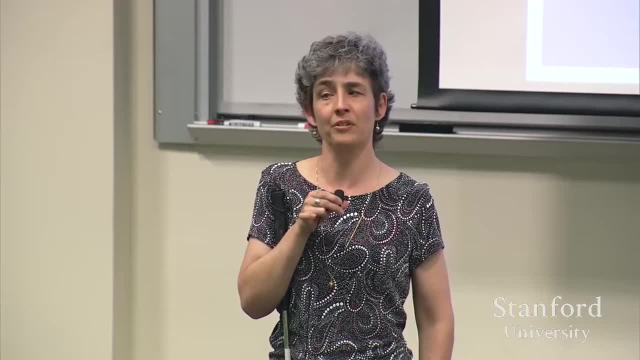 as soon as I can. Dr Allison is going to talk about the state of the art in theGSET for a little while. Good, I'm going to just let someone know that I'm going to hear from Dr Allison. So, again, I'm going to try my best, to do my best and we're going to see what they. 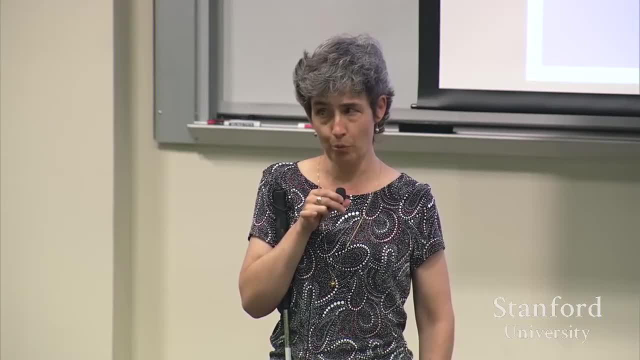 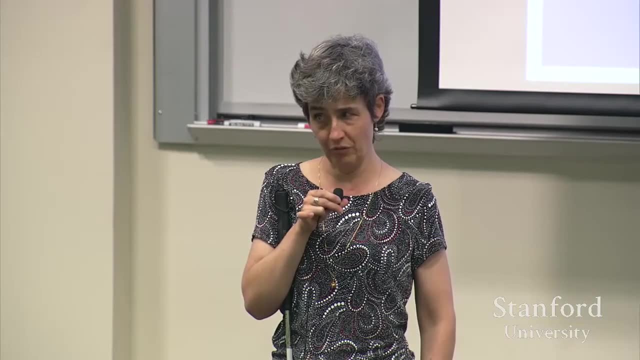 want to hear from each other. Dr Allison, thank you, I would love to hear from you. So this is Dr Allison framework, basically, that Stanford can use, And that framework has a lot of accessibility, features and functionality built in for free. 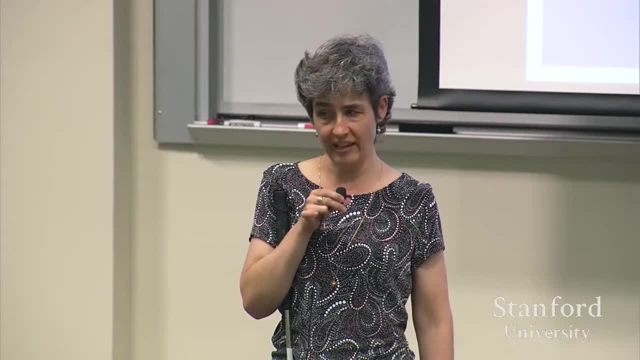 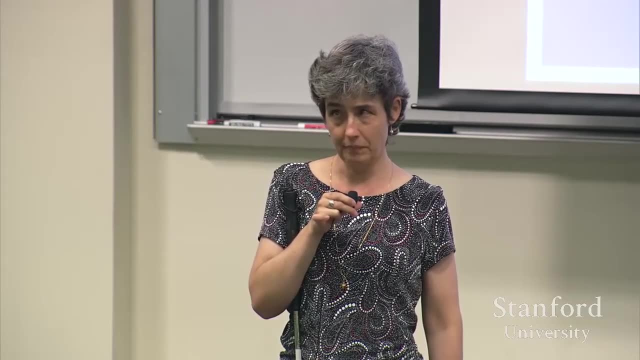 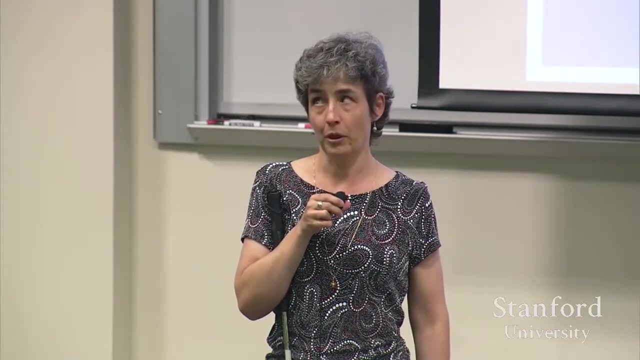 And so if people use Stanford sites, you can get it up and running with a website really quickly And get a lot of accessibility for free. So I'm gonna wrap up, but I want to leave you with two books And then I wanna take a little bit of a quick poll in terms of to find out who you 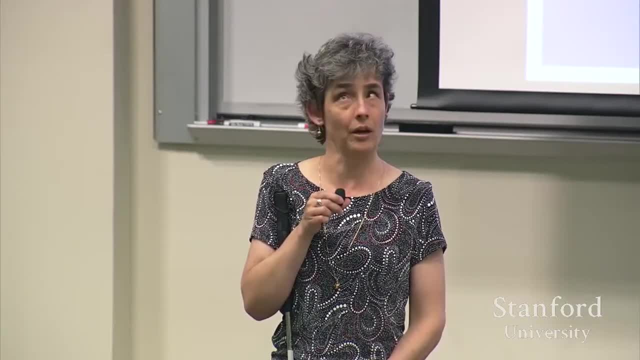 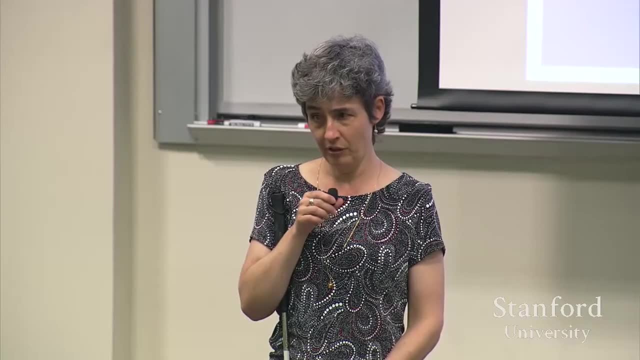 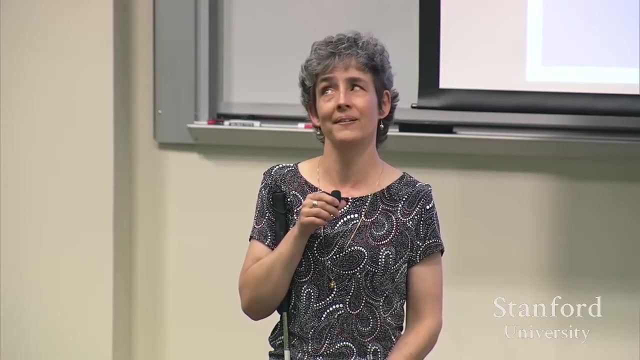 all are, so that folks who come after me will know who they're talking to. So books: I would recommend a recently released book that I know Stanford has. It is a Rosenfeld media book. Have you all heard of Rosenfeld media? 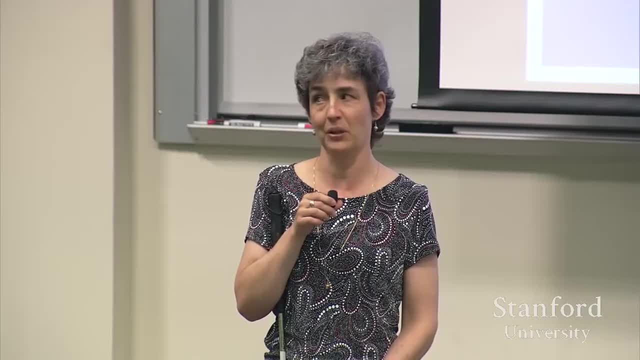 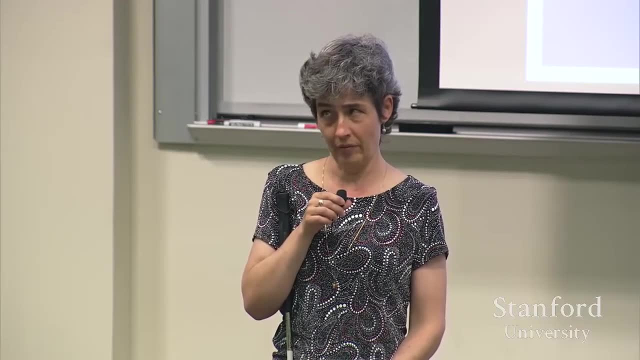 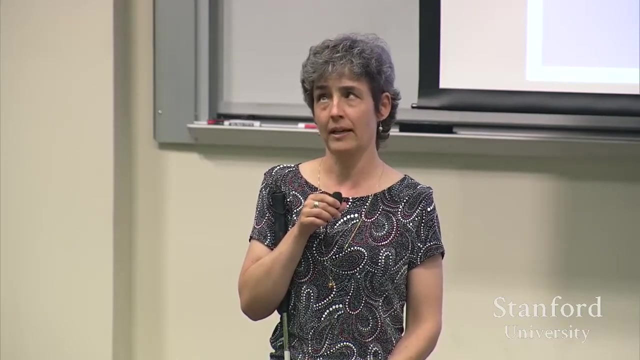 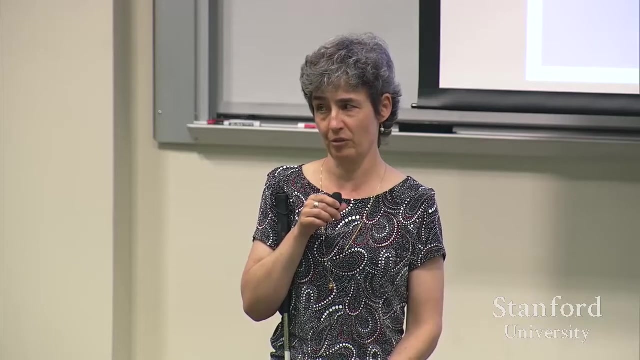 You should, cuz they've got all the great usability books And they also have a great book where we're having sort of crossover and interaction between accessibility and usability, which I believe deeply in, And that book is called A Web for Everyone, So it's available electronically from the Stanford library. 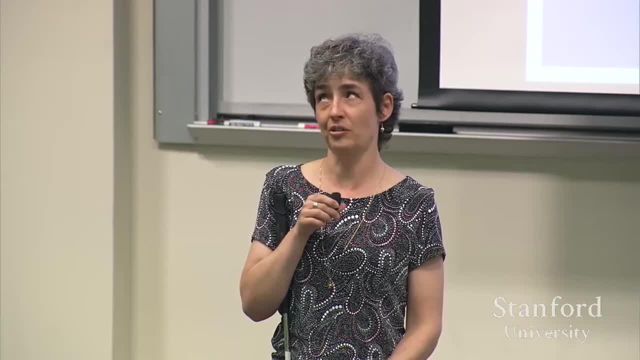 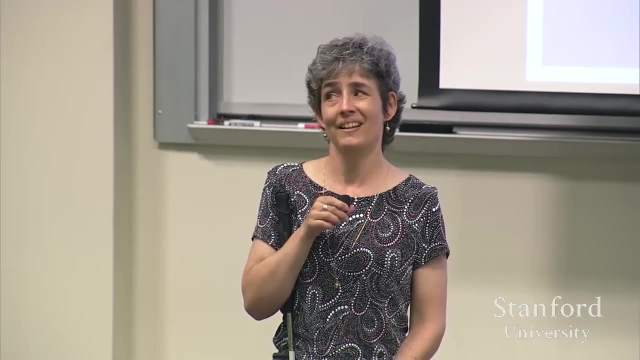 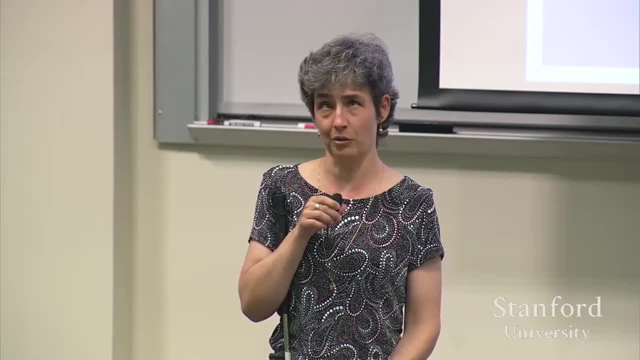 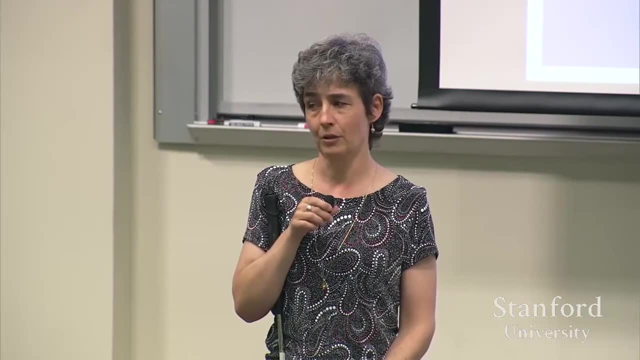 So that's one book, And then the other one was just crossing my mind when Michael was introducing me, So this is a quiz for anybody who can remember. There's this really good user interaction book, not so focused on the web, but 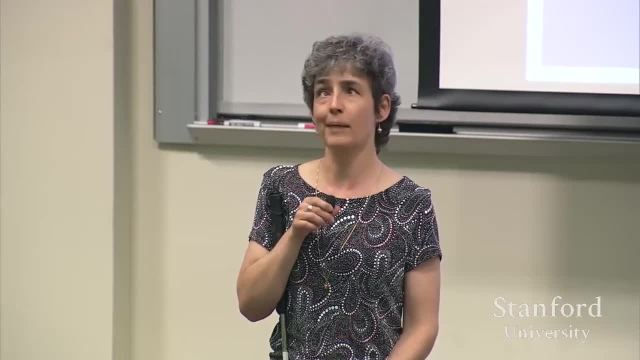 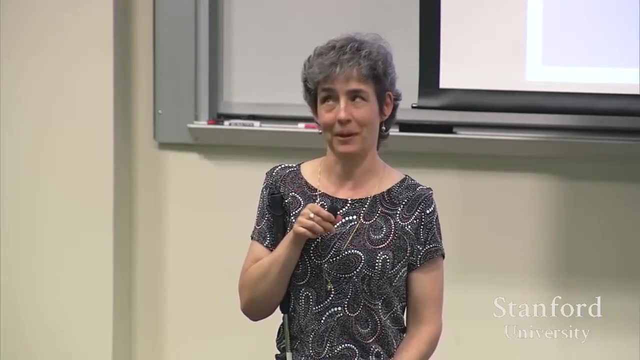 focused more on products and that kind of thing. It's by Graham Pullen. Anybody know this book. Yeah, Can't remember the title: Designing for Disability. That's right, that's right. So that's a really good one. 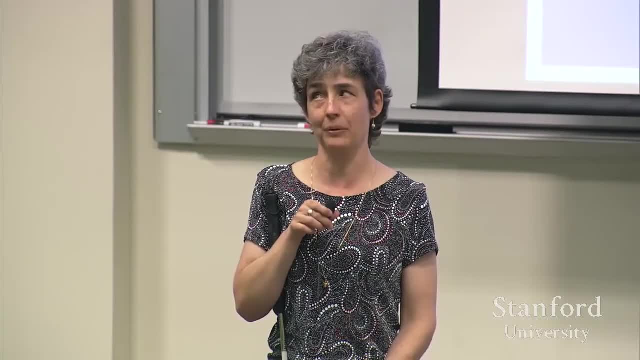 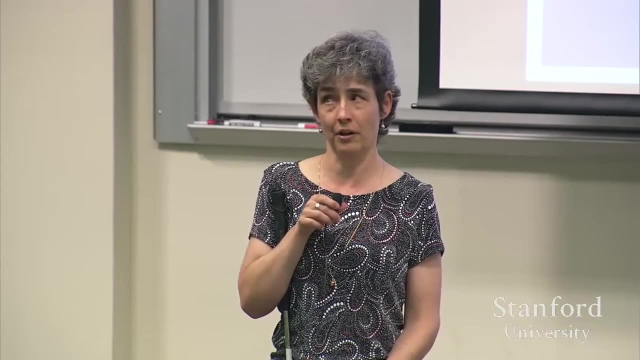 If you haven't taken a look, I would say that it's sort of one of the founding books in the field. So make notes of those and they'll get you off to a good start. A Web for Everyone focuses a lot on personas of people with disabilities and how they use. 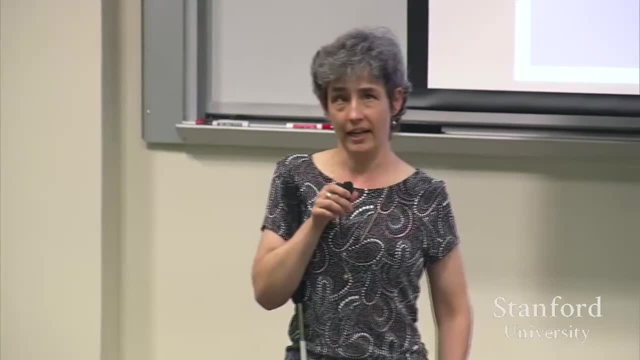 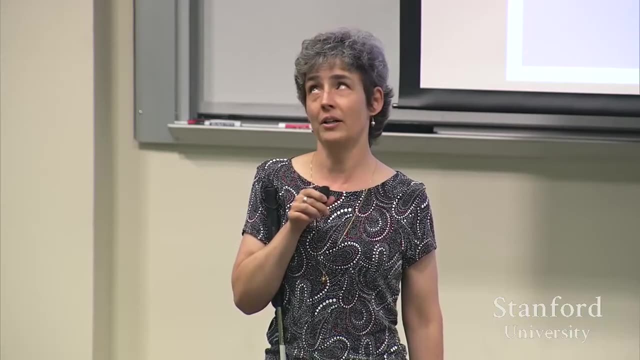 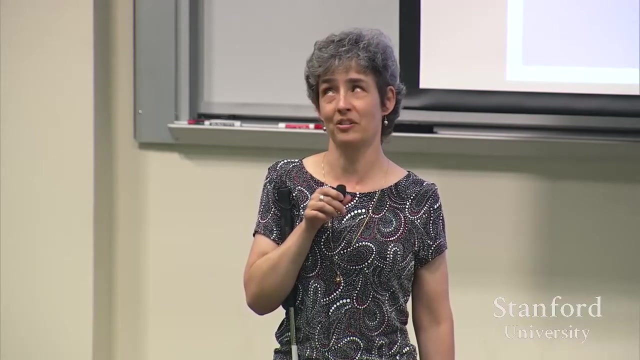 the web. So that's what I got for you today And to wrap up, I'd like to take we're going to do hand raising for sighted folks and audio queuing for blind folks. Okay, Don't shout out, because it's I mean, you know, speak up, but it's not a competition. 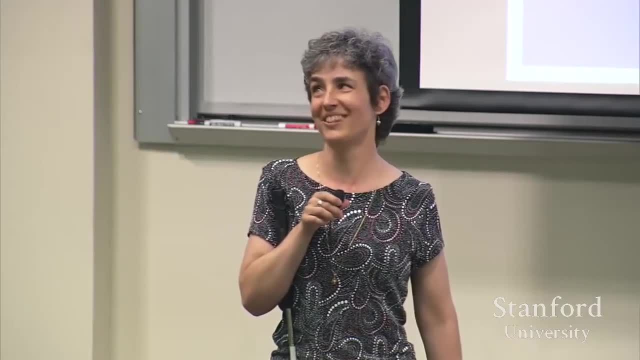 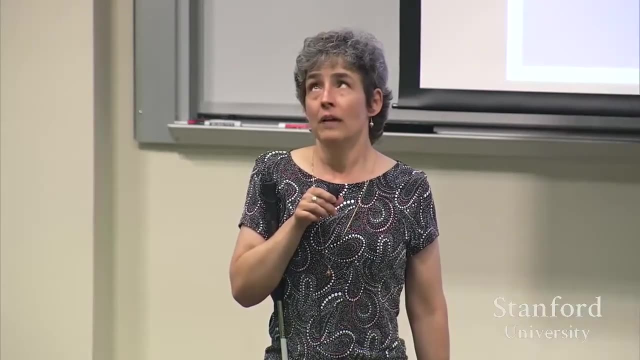 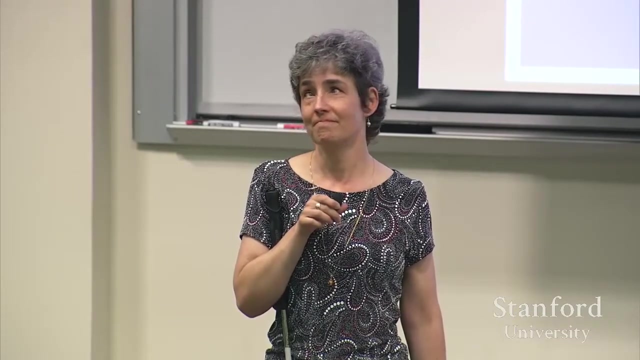 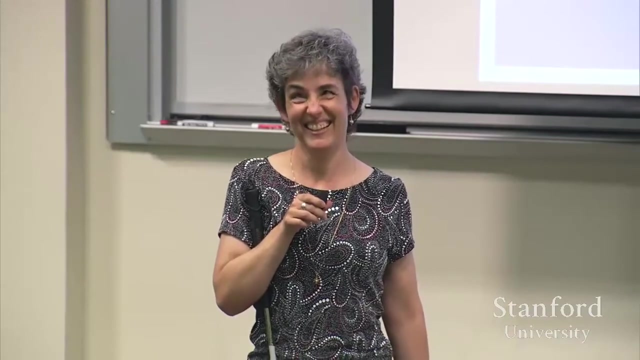 in terms of who wins, So don't skew the results. So how? first general question about how many people in the room- 60,, 60 or so, I was going to say- are we having food coma? I might be soon. 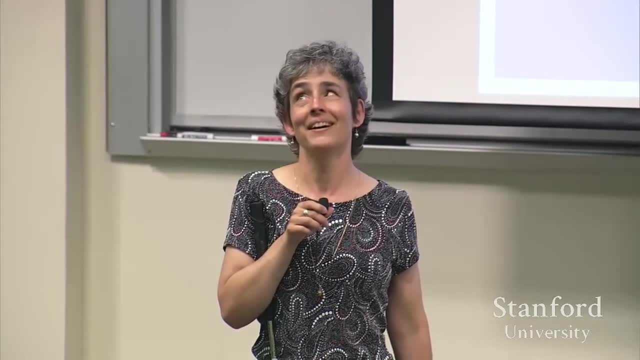 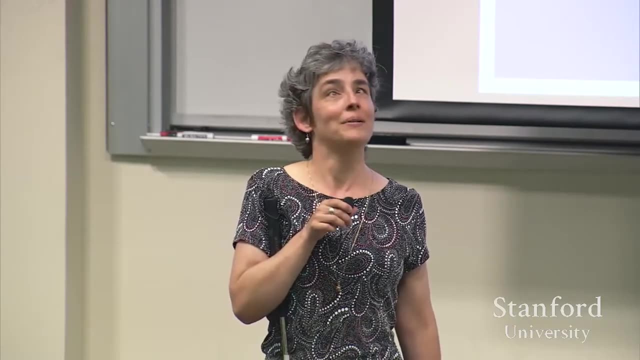 Okay, It's a Friday, Exactly It is a Friday. Okay, 60 or 70.. Okay, Students raise hands and give a little audio cue. Okay, So about half. A little bit more, Okay, Stanford staff. 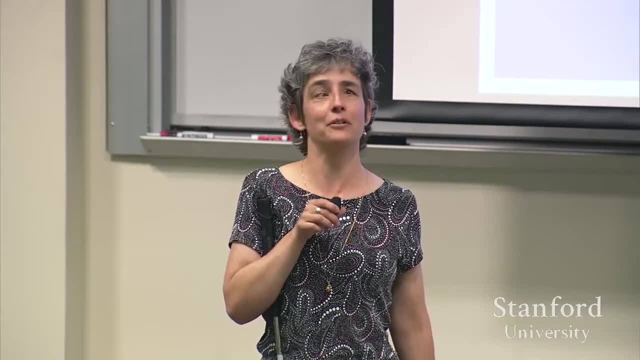 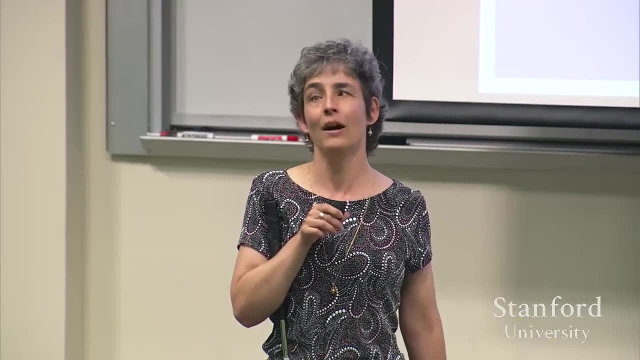 Okay, And that includes faculty as well. Okay, Good, You guys are separate too. Okay, Excellent, Does that pretty much cover everybody? Oh, public, We got some public people that might have come. Yeah, we did, That's us. 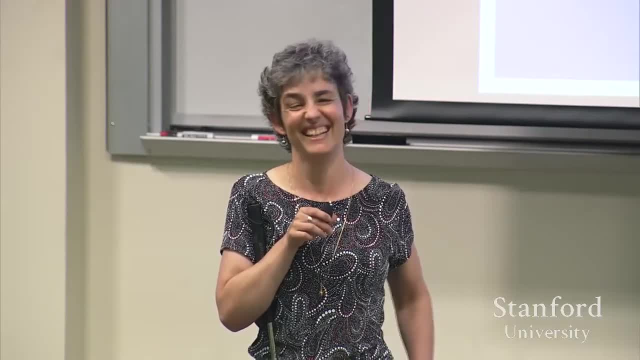 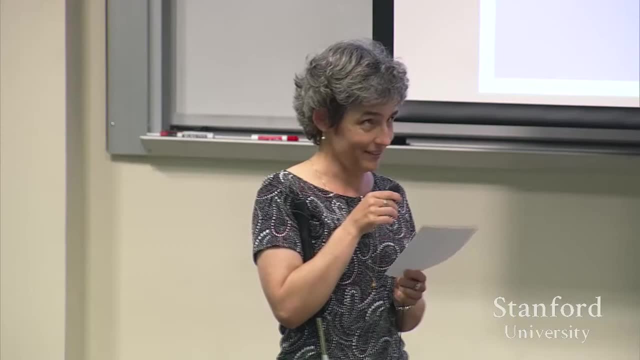 Yes, That's us. Okay, Excellent, Okay, Excellent. Thank you guys for your time And I know I went over, but we're done, I'm done And next person. You're good, You think I hit it? 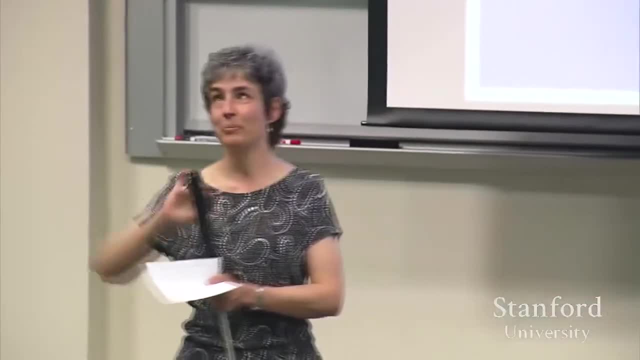 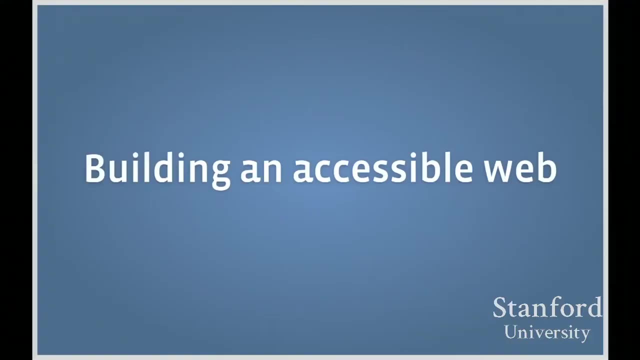 Okay, Excellent, All right, Quiet, Victor, here's your hand. Thanks, Jennifer. Thank you guys. Thanks Michael. Okay, So the title of our topic is building an accessible web- making sure that the web is usable. 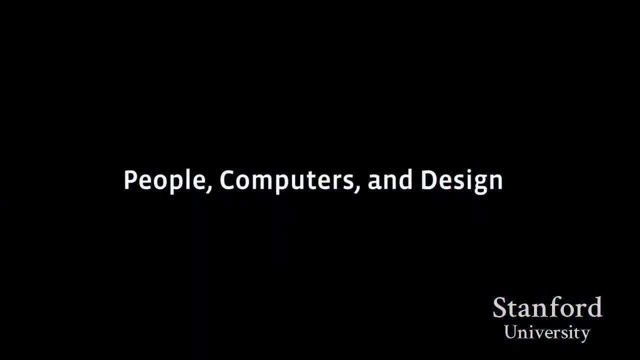 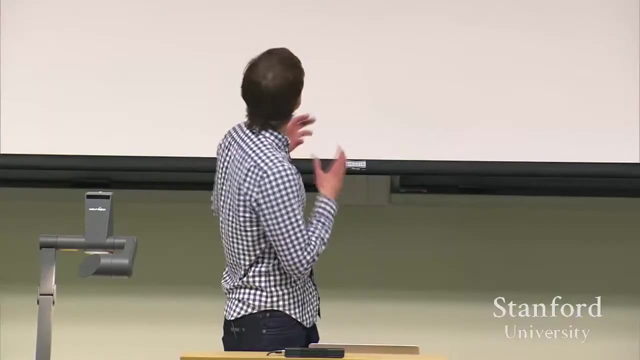 by all people. Now, before I go into that- Okay, Now before I go in and unpack what that means a little bit more tangibly- I wanted to try to root this topic of accessibility within the context of CS547. So, according to CS547's website, this is a seminar about people, computers and design. 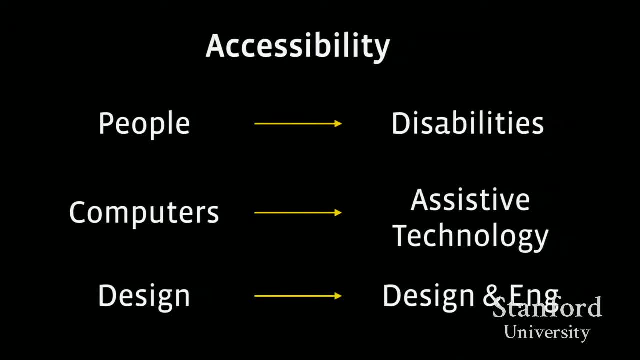 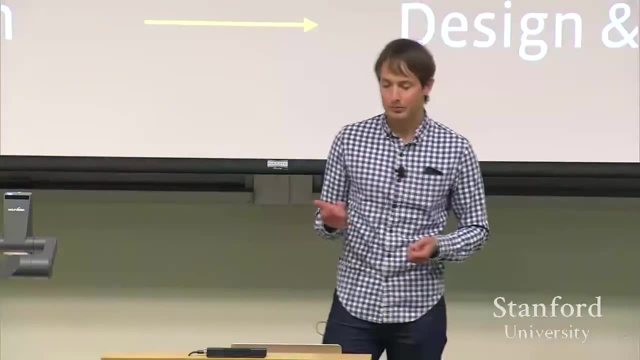 And this is actually a really nice capture of what accessibility is about, because accessibility intimately touches each of these three things. So when we use the term accessibility in the context of technology, We are typically talking about people with disabilities interacting with computers And in order for people with disabilities to interact with computers successfully, 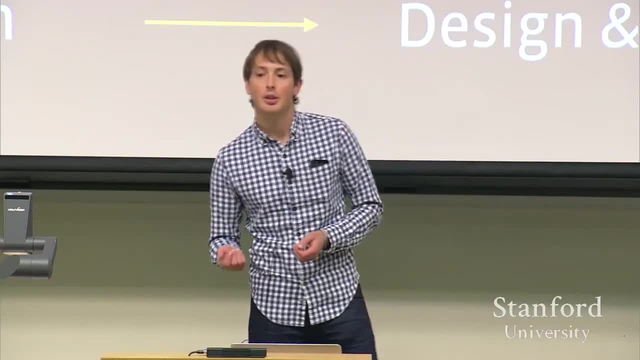 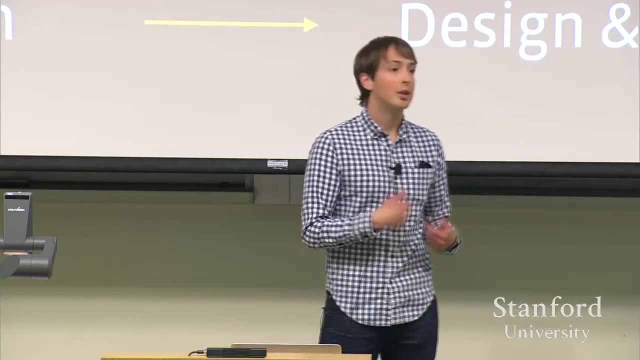 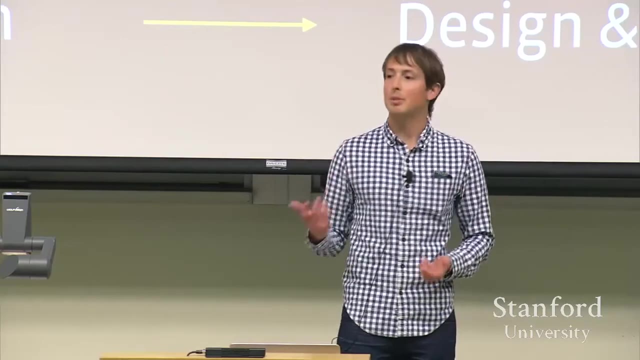 in some cases, they need to use assistive technology. Now, one example of that that we're going to focus on today is screen readers, And that's a piece of assistive technology that blind people use to interact with the web. The place where design comes in is that, in order for your experience, your web experience. 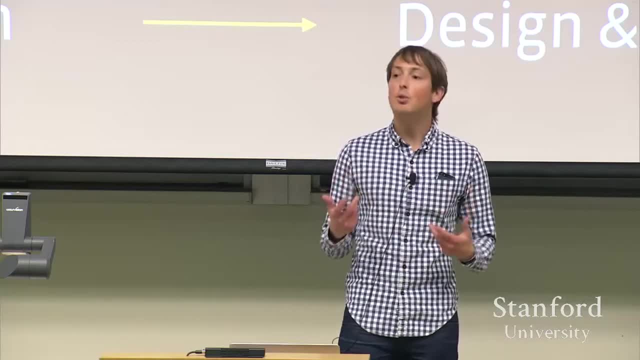 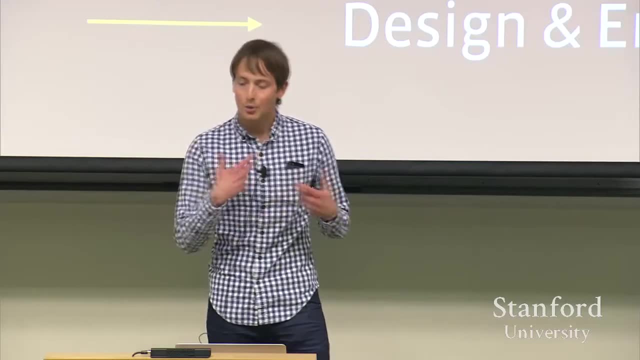 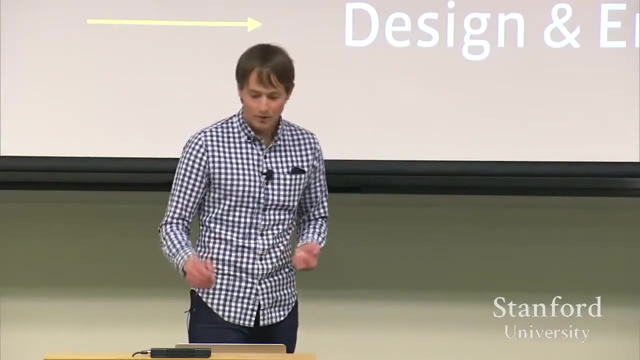 that you're building, the product that you're building, to be usable by somebody, say, who is using a screen reader, you need to make conscious decisions about how you design and engineer that web experience. You don't always just get accessibility for free. 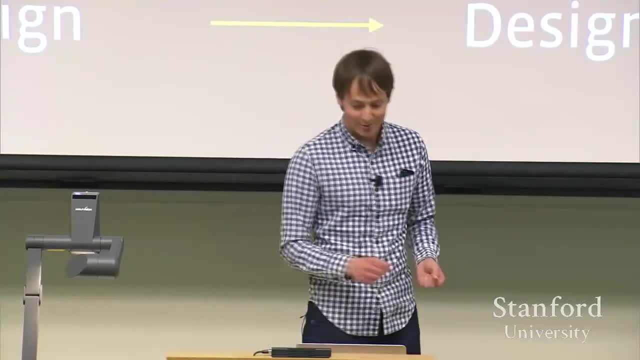 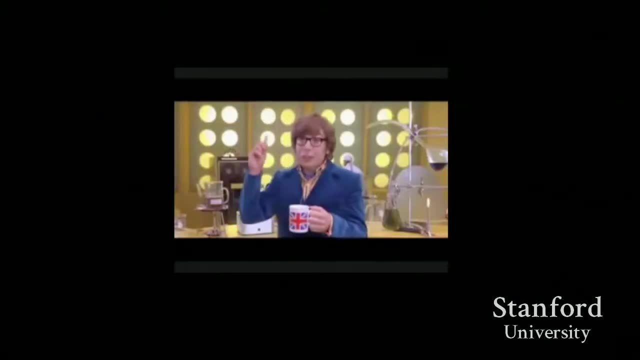 So I've been talking pretty abstractly for the past minute or so And it's not unreasonable that you might feel a little bit like Austin here: Whoop-de-doo. What does it all mean? What does it all mean, Basil? 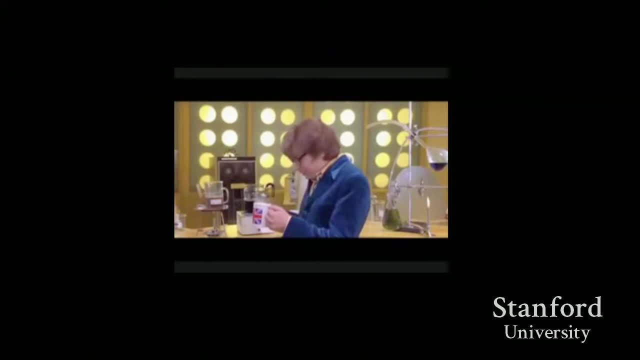 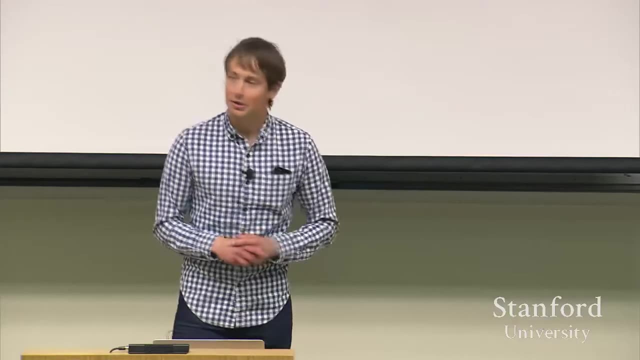 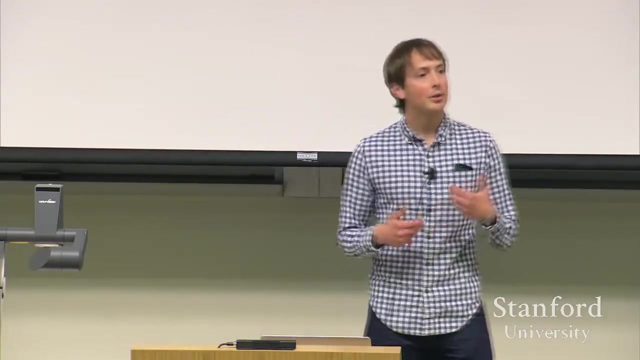 What does this all mean? What does it actually entail in terms of trying to make one's web experience accessible to people with disabilities? So we're hopefully going to explain some of that today over the course of the next 30 minutes. prove to you that you do need to make some conscious decisions, but also empower. 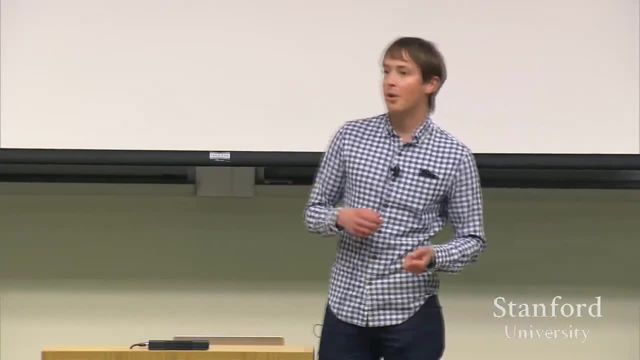 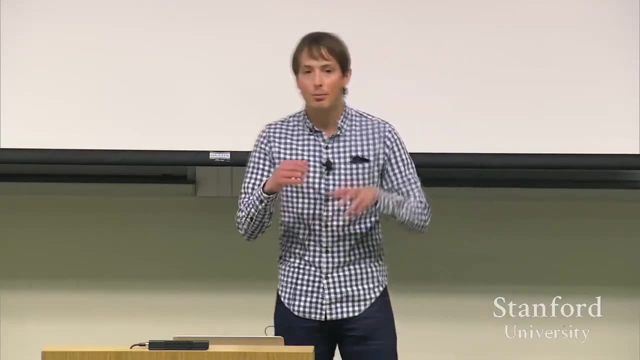 you guys to know what to do. Whether or not you are engineering a website, designing a website, doing research from an online perspective on a website. it's important for each of these people who touch a product to understand a little bit more about what accessibility is and what you need to do to. 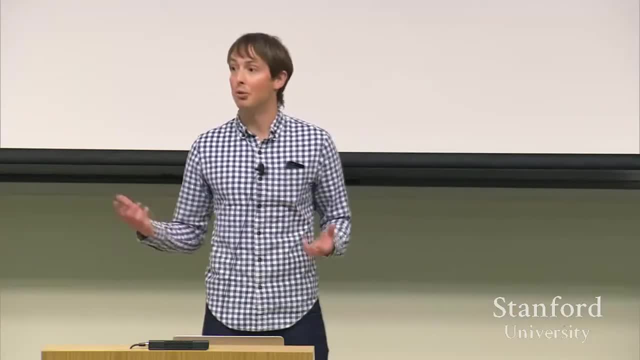 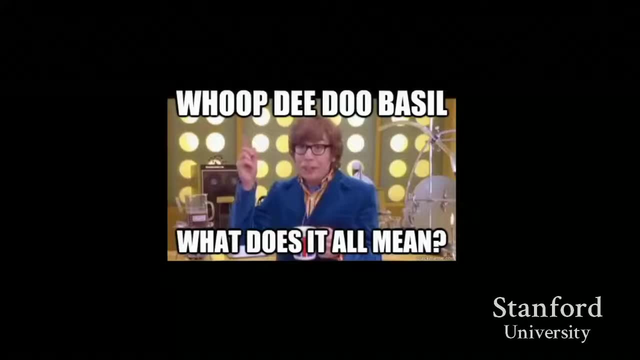 make something accessible in order for the web in general to become more accessible. So, to make this a little bit less abstract and really make this a lot clearer to you guys, I'm going to pass this over to Victor And Victor is going to walk you through what the experience is like for somebody who is. 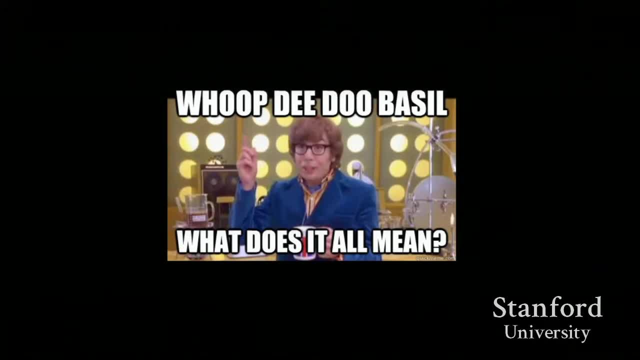 using a screen reader to interact. Victor is going to walk you through what the experience is like for somebody who is using a screen reader to interact, So let me just show you how that works. There's a screen reader. This is a screen reader. 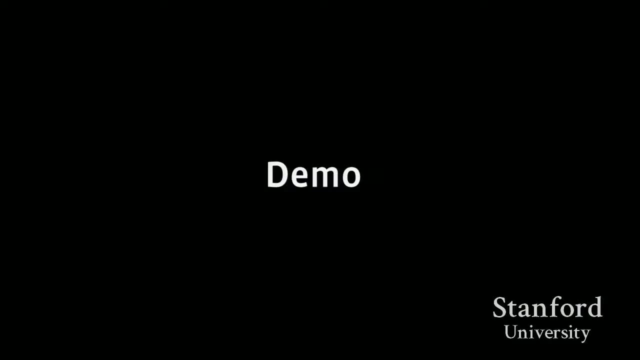 There's a screen reader. You can also open the screen reader and getWhat they use. You can see here how they operate. So it's a screen reader. It's something that you can use to analyze the content, interact with the computer. 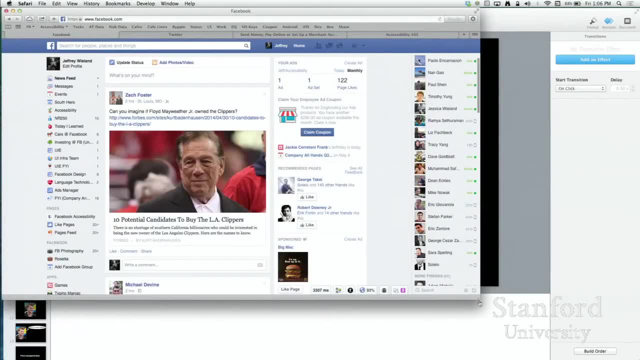 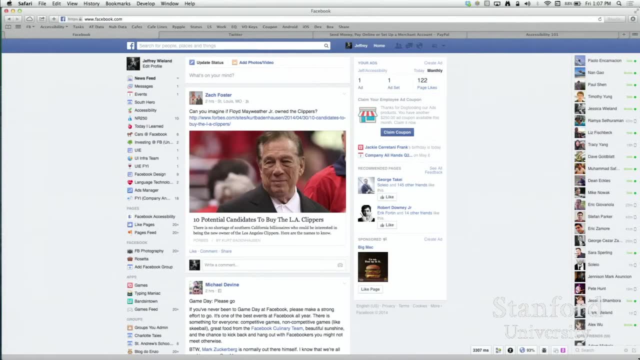 and interact with the web. All right, Let me just come here, right? Yeah, Cool. So let's just to your right here. Here's the machine, Yeah, Awesome. Okay, let's see. Is the mic working? Hello, hello. 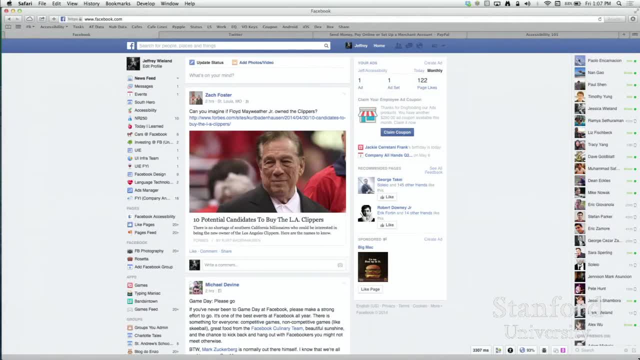 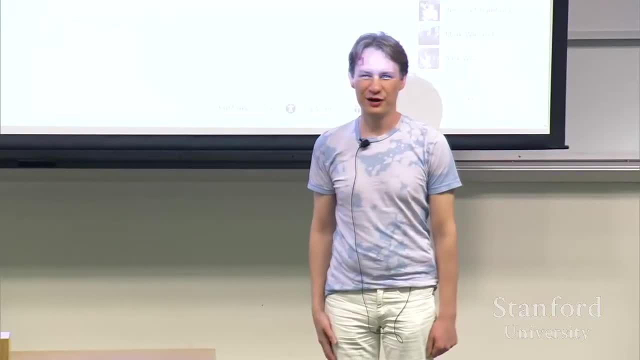 Yeah, I think so. Hey, you too. Can you hear me? I don't think so. Hello, can you hear me? There you go. All right, have my coffee, sorry. so, hey guys, thanks for coming. this is always great to talk to students. 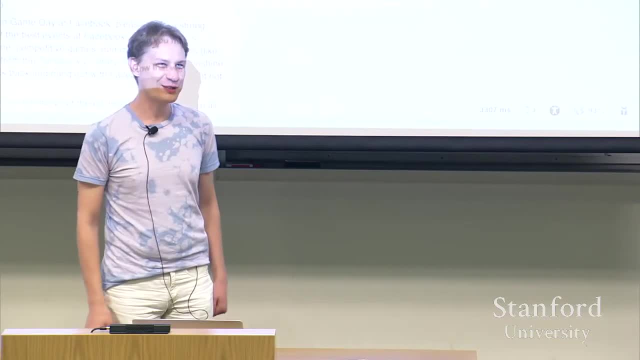 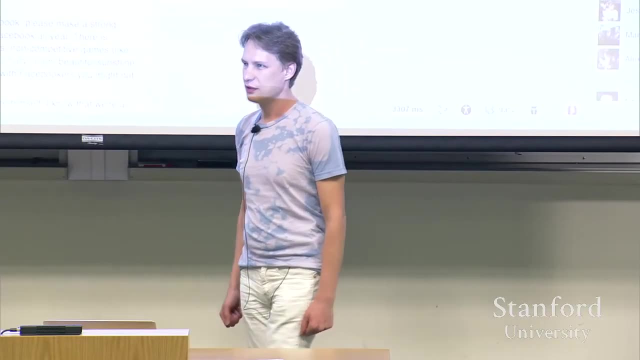 I've been one myself, as you can imagine one day, and especially to your HCI people, this is like even more amazing. this is one of the areas that I personally work in at PayPal, but this is also the area where I spend most of my life is just making the darn computers interact with me, right? 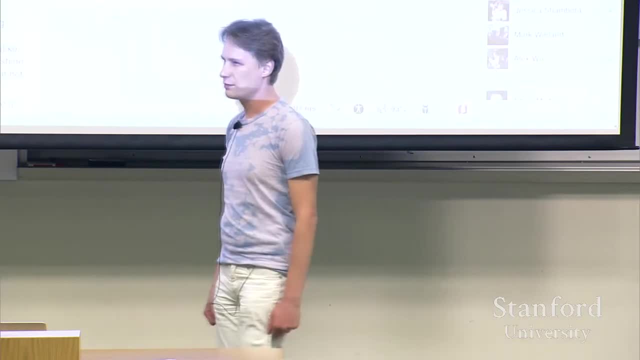 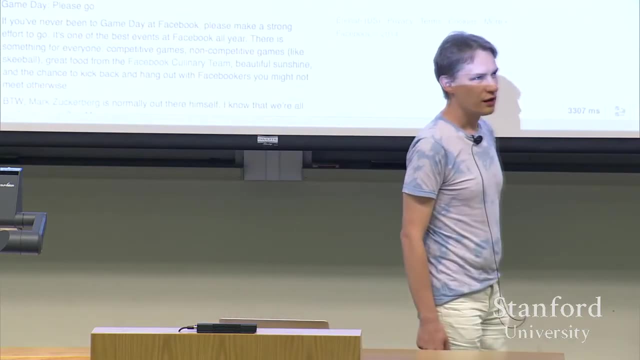 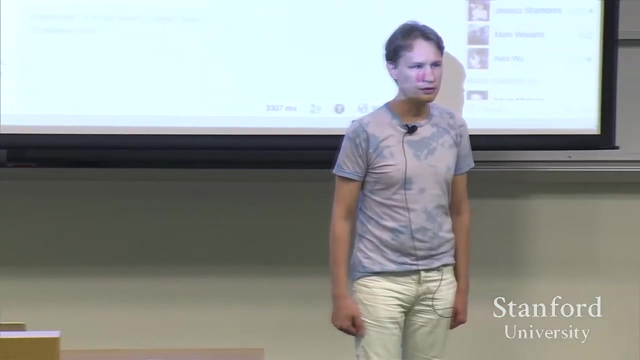 this is just as big of an HCI problem as any other one, and most of you interact with the world by looking at things around you. everything is. you've been bombarded with a lot of visual information, so naturally your visual sense is overloaded, and but that's unfortunately pretty. 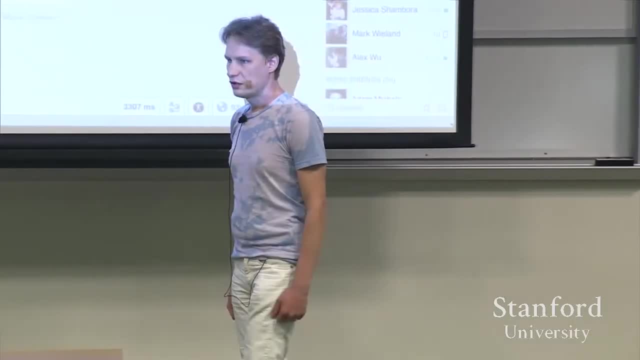 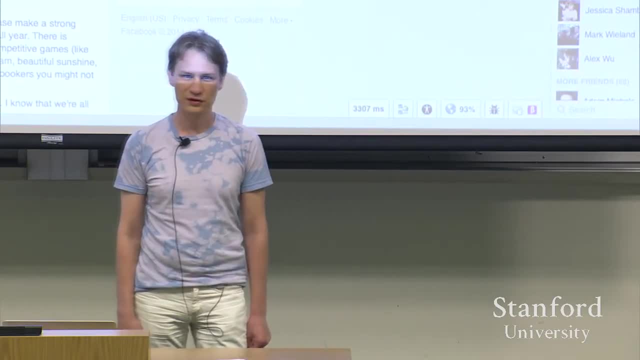 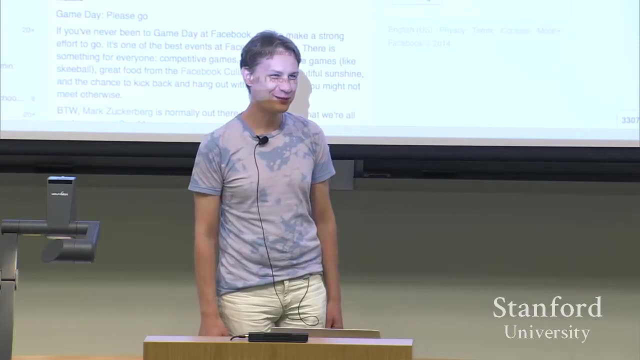 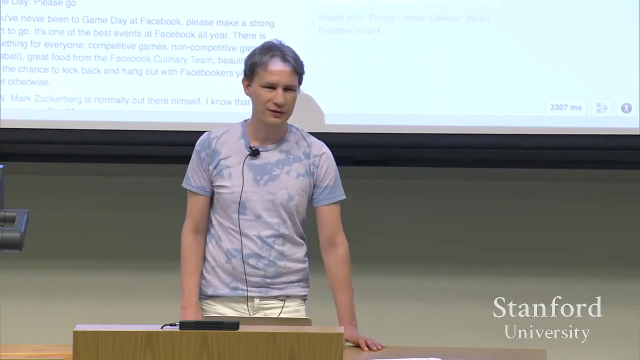 and that means that I'm not bombarded with all the junk that you guys are. this is a great thing. I don't see all the freaking ads and things like that. another great thing? I don't, you know, I don't. I don't see all the pop-ups and animations, but unfortunately, good or bad, they do interfere. 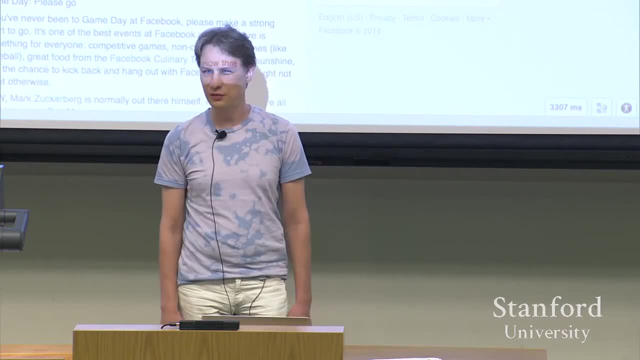 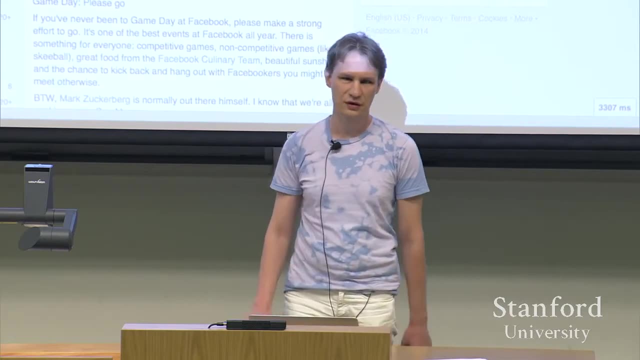 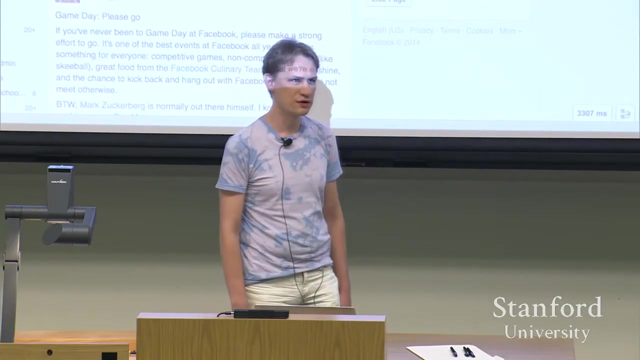 with my experience and I'm going to show you in this in a minute why so. how do I interact with the computer? I use a technology that Jeff already mentioned, called screen reader. screen reader is a slightly modif, slightly misleading name, because all of us are screen readers, right you? 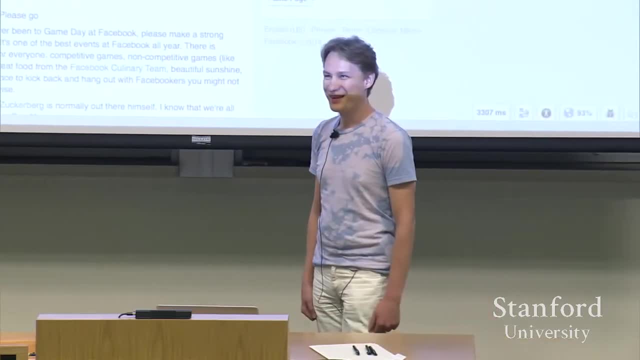 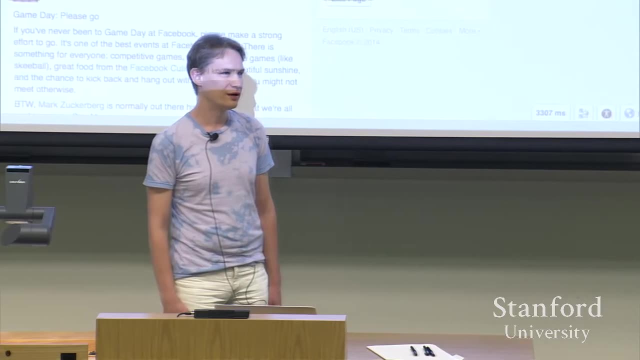 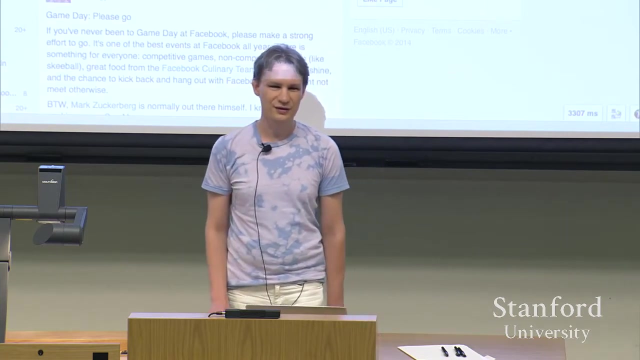 guys read screen, right right. so when I started back at the university, I had a lot of screen readers people who would read screen for me because at that time there was no computers that I could take advantage of. but the technology I'm talking about is actually a software that is built. 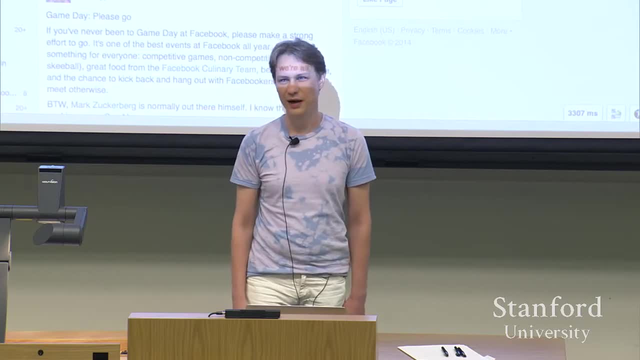 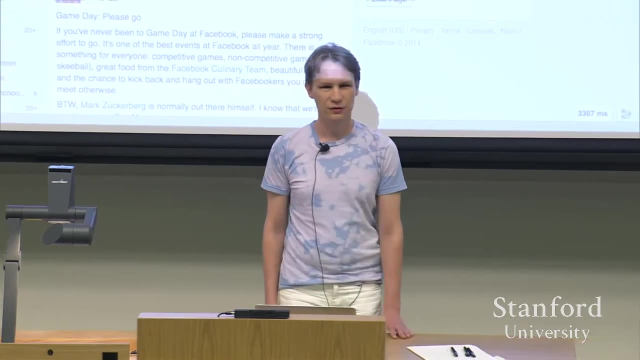 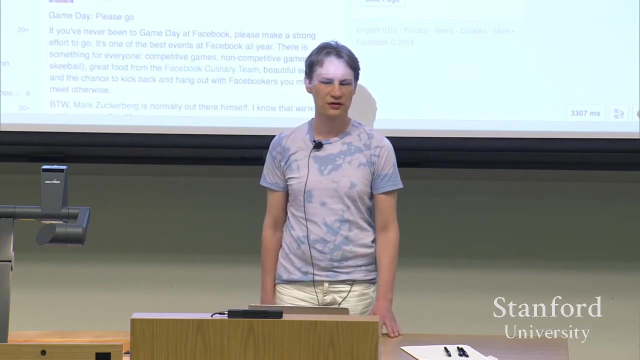 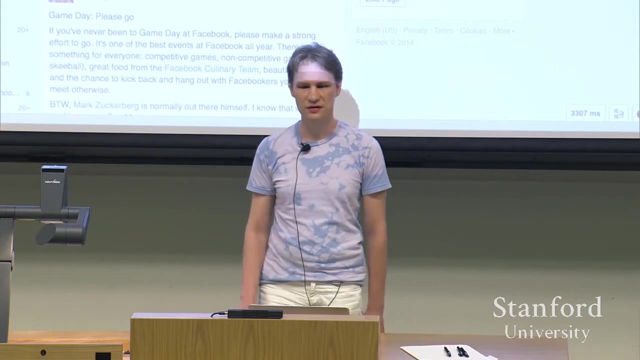 into every modern operating system- mac os, windows, ios, android, you name it. they all have the software we call a screen reader, and essentially the task of a screen reader is to to communicate this, the information that appears on the screen, to somebody who cannot see. so this is done usually via speech synthesis, and I want to separate those. 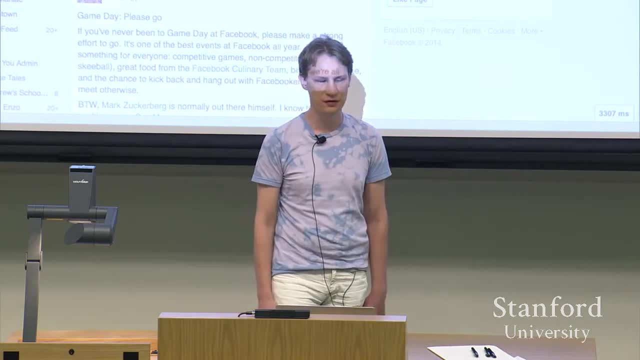 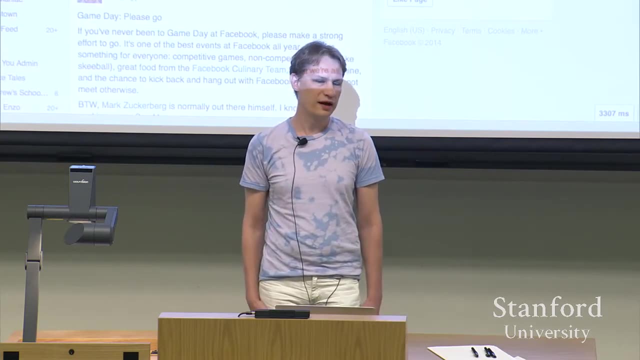 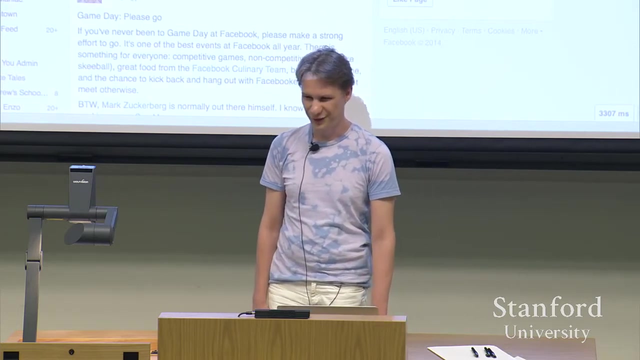 two things for you right away, because most people think that speech is a part of the screen reader. this is exactly, not, not exactly correct. speech synthesis is different from screen reader, and we'll find out in a moment why. so let me see. I haven't used Jeff's computer before, so let's see what's going to happen here. 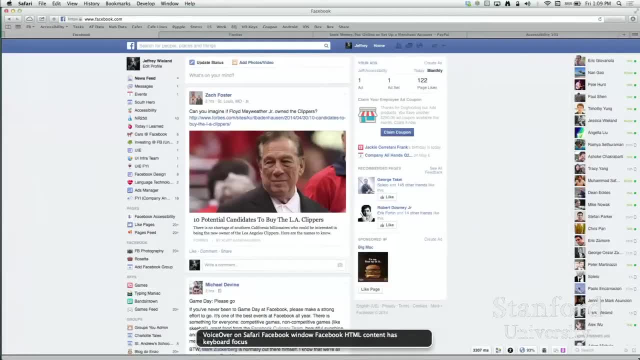 voiceover on safari. facebook window, facebook html. that's cool, all right. so back in 2005, I think, or 2006, apple said that we can make it possible for anybody to be able to communicate with a screen reader. that's cool, all right. so back in 2005, I think, or 2006, apple said that we can make it possible for anybody to be able to communicate with a screen reader. 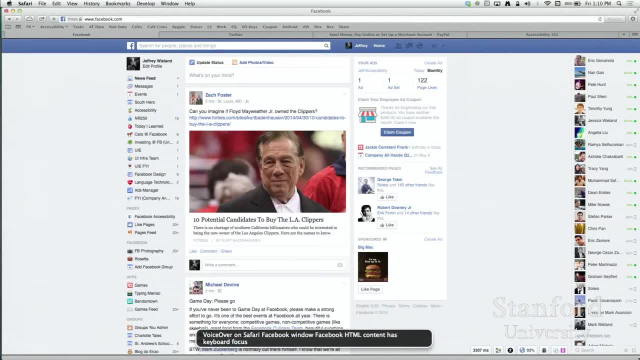 blind user to come up to any Apple computer anywhere in the world, press a shortcut key and be ready to go. any blind user to come up to any Apple computer anywhere in the world, press a shortcut key and be ready to go. at that time what you had to do. and on Windows, if you're like on anything before Windows 8, you still have to do that. 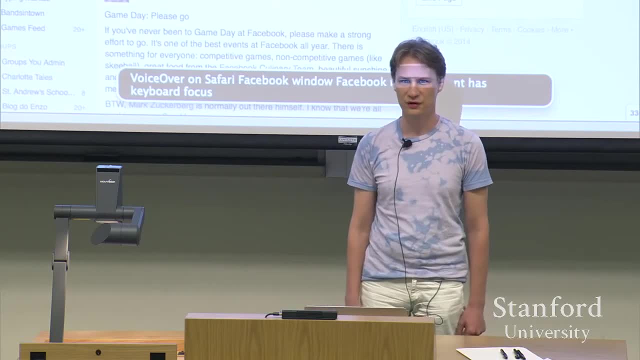 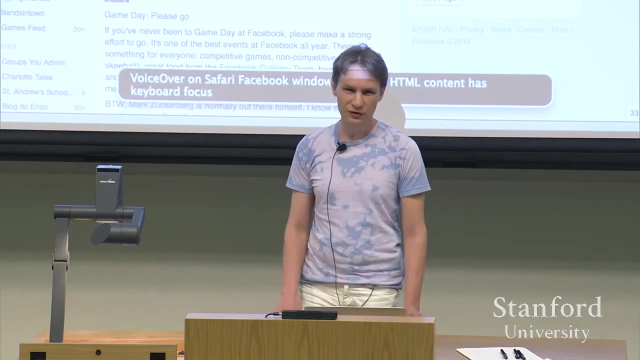 you have to actually ask somebody to go and download for you the piece of software, help you install it, launch it for you, and only then you will be able to go ahead and use the computer with Apple. all you need to know is that when you press command F5. 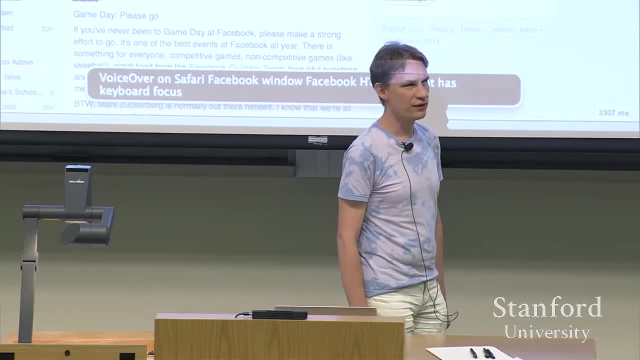 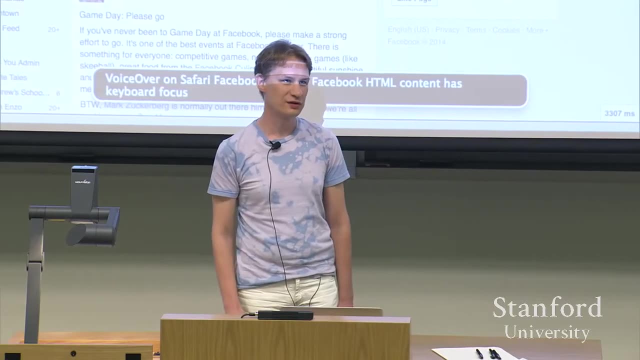 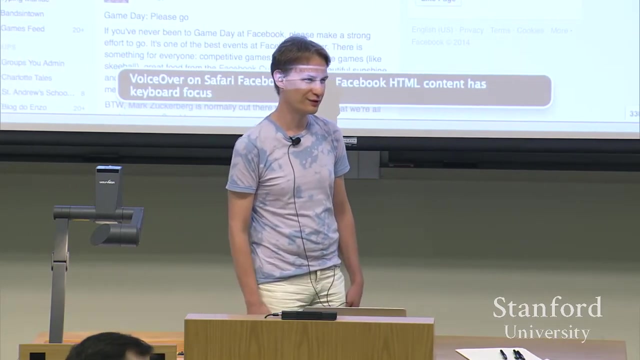 this thing launches, no matter what you do, are you whether you're reading your email, whether you're on Facebook or, you know, using PayPal or whatnot? it's gonna launch and it's gonna start talking to you. so from then on, most likely, what's gonna happen to you? just gonna get confused because you're like I don't. 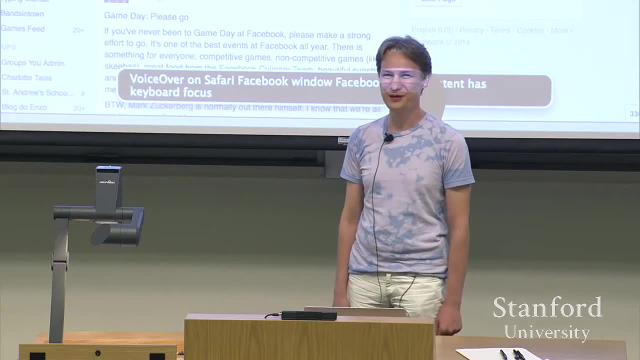 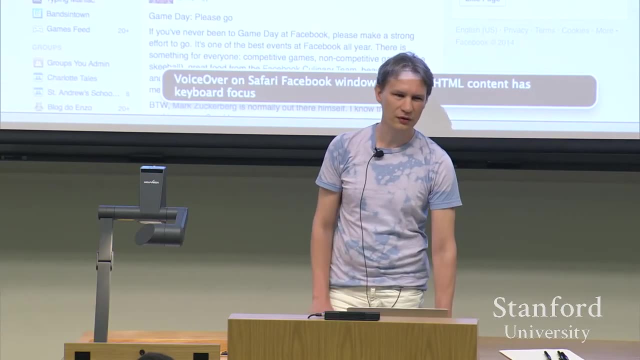 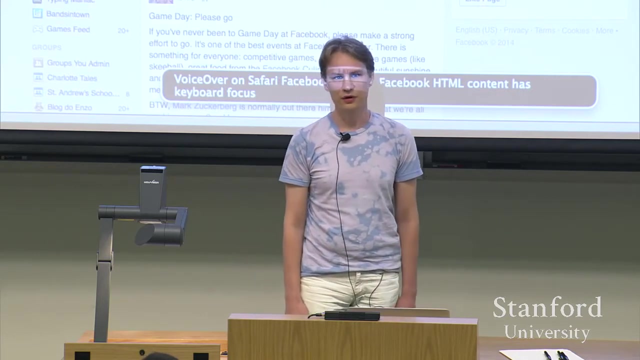 know what to do with this thing. right, because one of the things you will find out, that screen you will. not only that it talks, which you probably need to be able to understand, but it also you probably need to be able to understand, but it also will in interfere with with the way you use the computer. I'm not gonna go into. 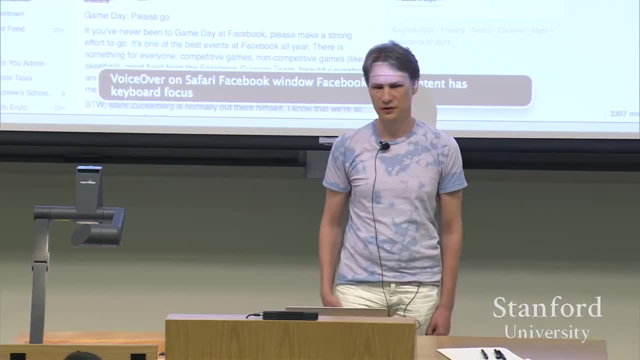 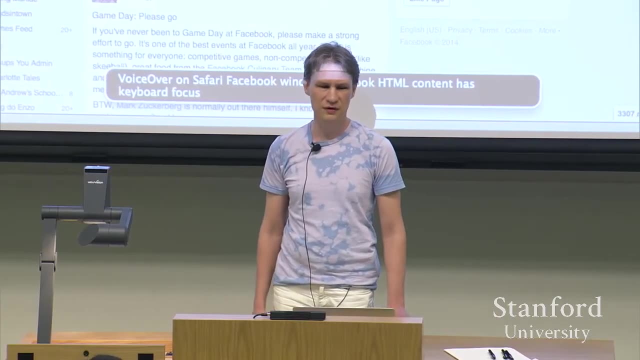 all the details because it's a little bit maybe more advanced for this particular presentation today, but suffice it to say that, in order to be efficient and using the screen reader, you need to know how it works. I mean, it sort of makes sense, right? I mean, in order to be able to to drive to San. 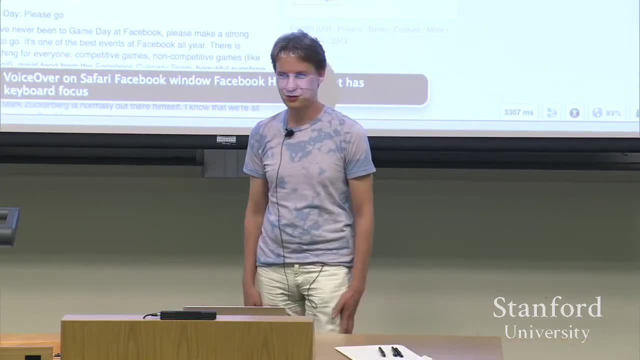 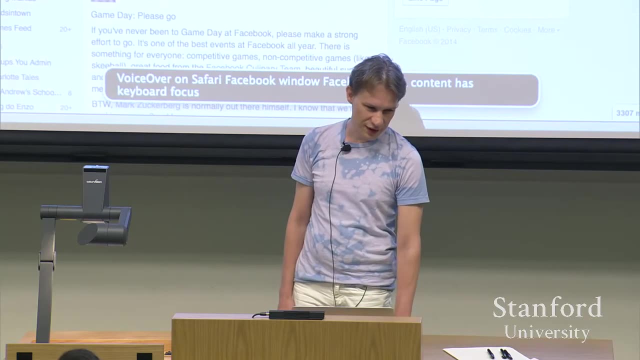 Diego, you need to know how the car works right. so same way. so learn the rules of the road. so the rules of the road for the screen reader is that, as a blind user mouse is useless to me, number one. so anything I do on the web or anything I do on a 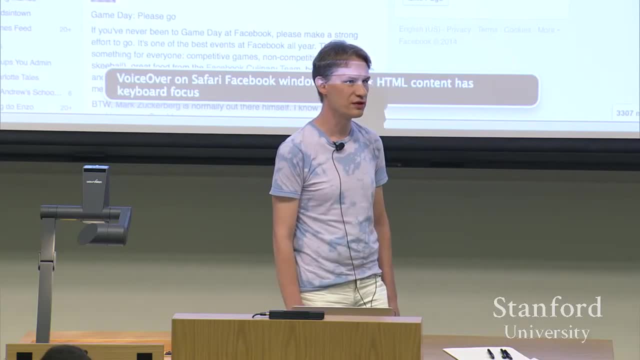 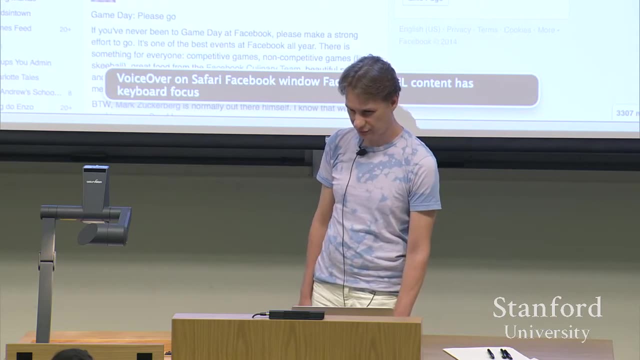 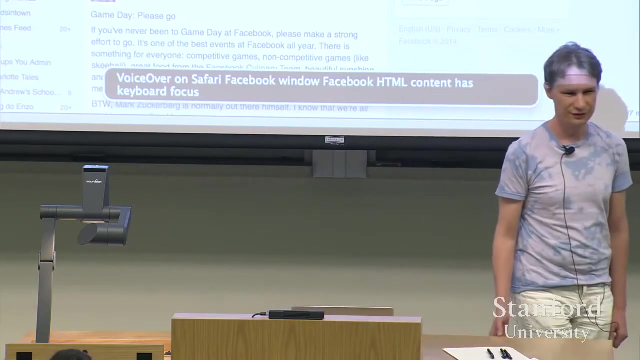 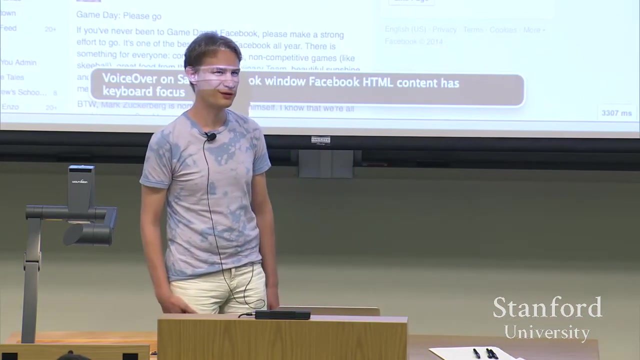 desktop needs to be available, accessible, reachable via keyboard. most of you guys probably know the keyboard right. how many keys you think you know on the keyboard? what is the bit? what is the biggest? what is the biggest key on the keyboard? oh, that was too quick. what key do you need to press to continue? oh, that's an old Microsoft joke. 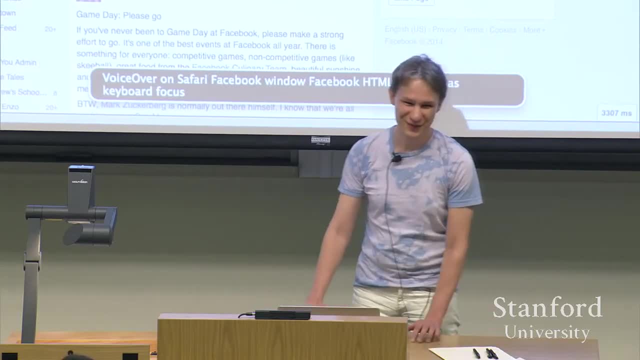 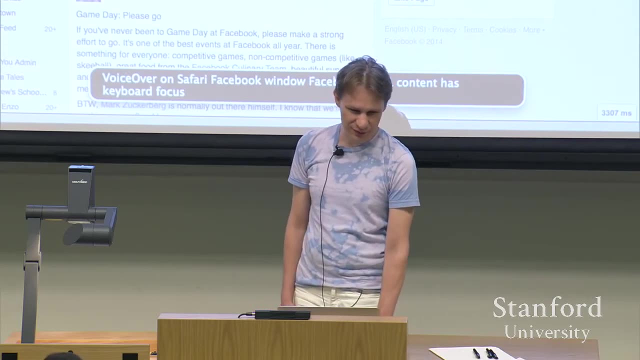 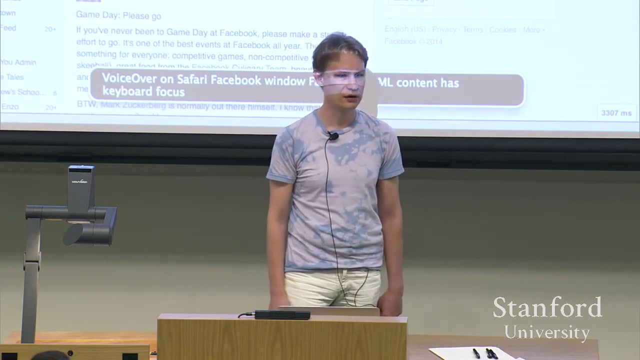 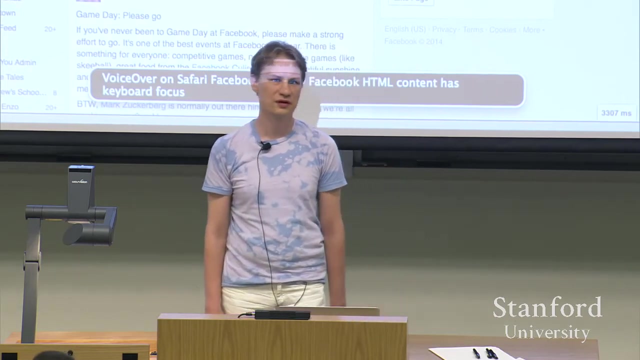 sorry, press any key to continue, okay, okay. so in my instance, just to keep things simple, I need to use mostly tab key and arrow keys to be able to do anything- well, not anything- most everything- on the desktop. there are other shortcuts you'll see me using. they're specific to a screen reader and 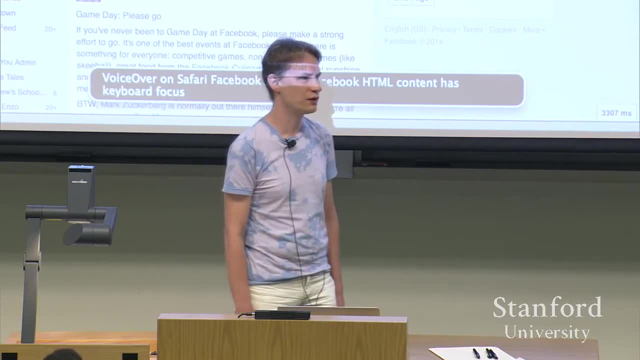 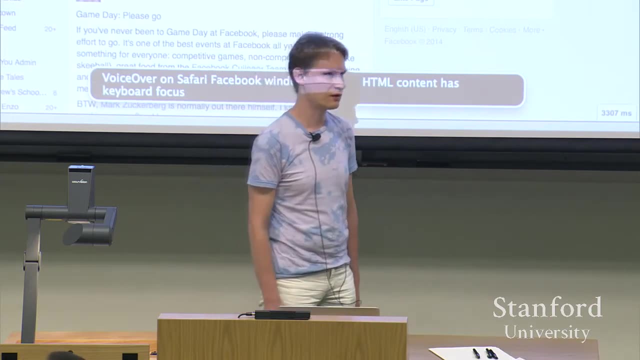 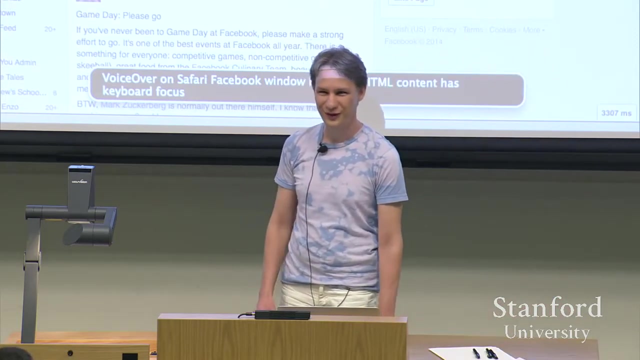 by the way, this particular screen reader is called voiceover, as I mentioned, is built into every Mac. so this is great. if you don't believe me, go to your closest Apple Store. and if you want to impress your, your partner or the sales rep rep in the store, just press command of five and like: hey, did you know anyway? so 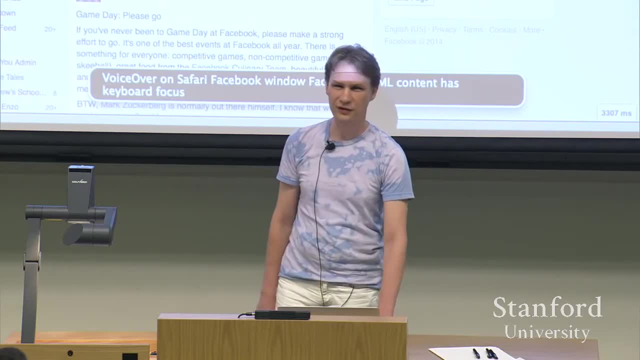 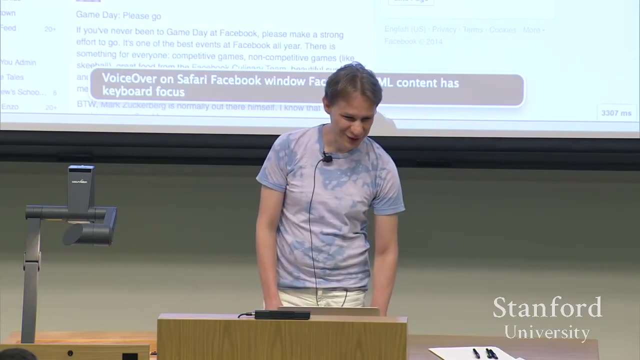 press it to turn it off when you're done. well, I think that's not necessary. actually, that that's. that's fun, if you don't. actually, that is the coolest thing ever. okay, so like Facebook finder. so I'm gonna go to the desktop, the first thing I'm gonna do. 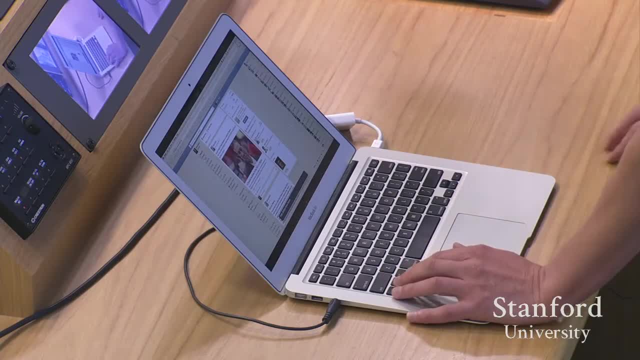 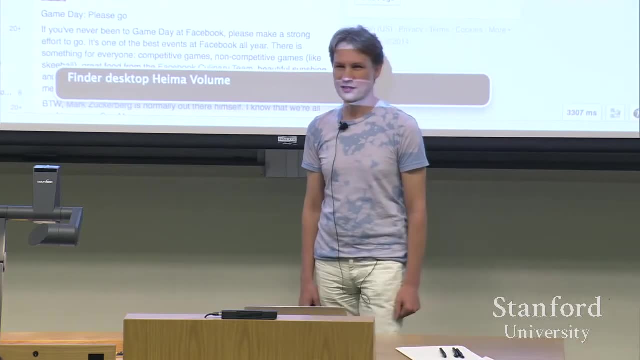 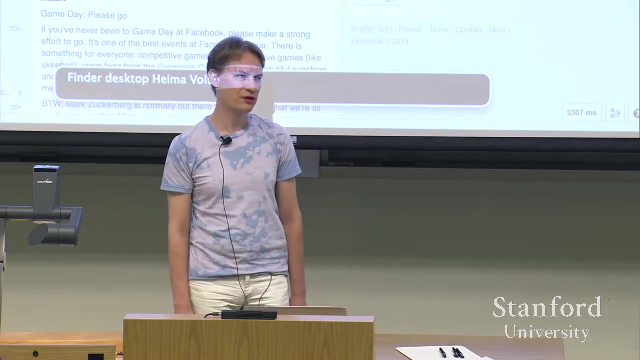 I'll slow this thing down, as you can imagine, just like with the car, there are people who drive slowly, there are people who drive like crazy and there are people in the middle. that's the same way we read with the screen reader. right speech is a very personal thing. some people talk fast, some people listen fast. 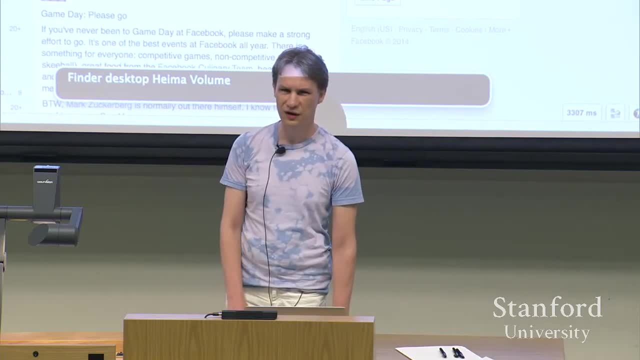 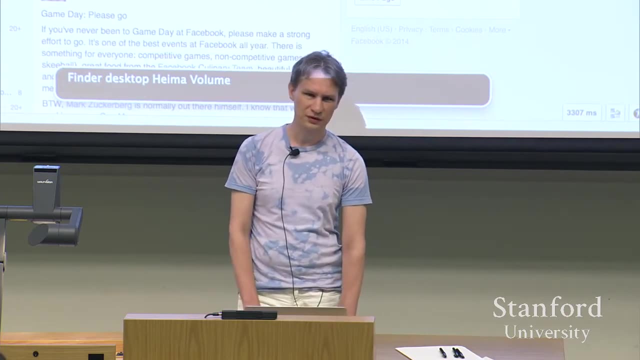 and so, in order for me to be able to interact with a screen, I kind of need to find what's the most, what's the most uh appropriate thing for my particular ability to listen. uh, most people. volume: one hundred percent. pitch: fifty percent. intonation: fifty percent voice: alex great: fifty percent most. 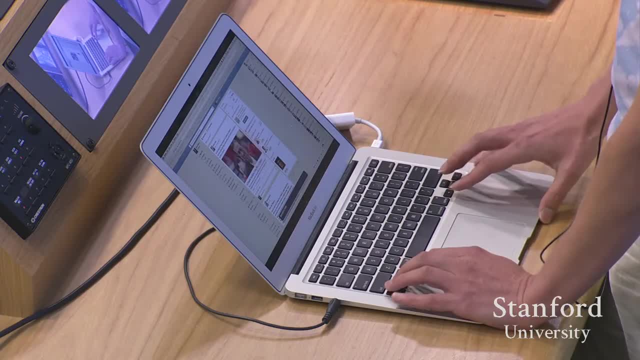 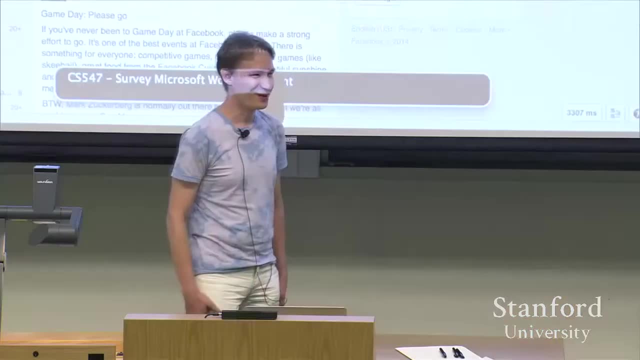 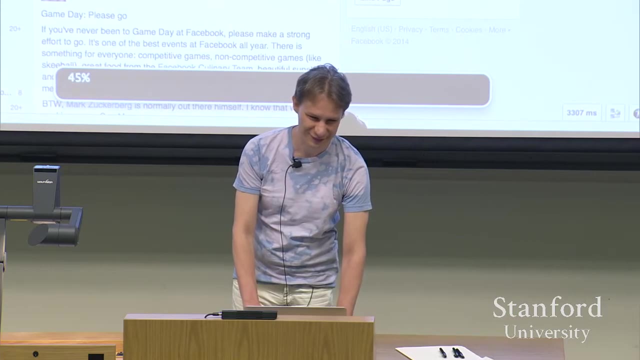 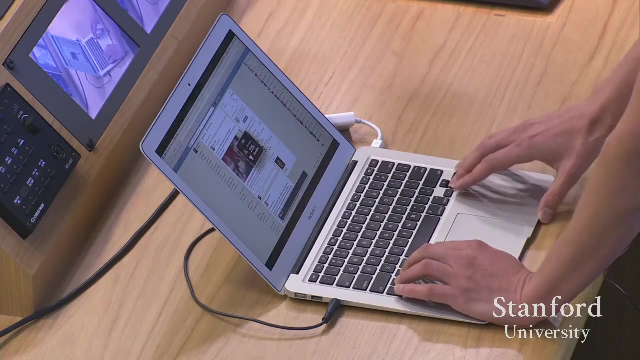 people will listen to something like that. all right, did you get it? okay, cool. so for you guys, i'm going to slow it down just because i'm really nice person. fifty percent, thirty five percent, all right, actually, you know, this is ten one percent. okay, you got lots of time right, do you? we? 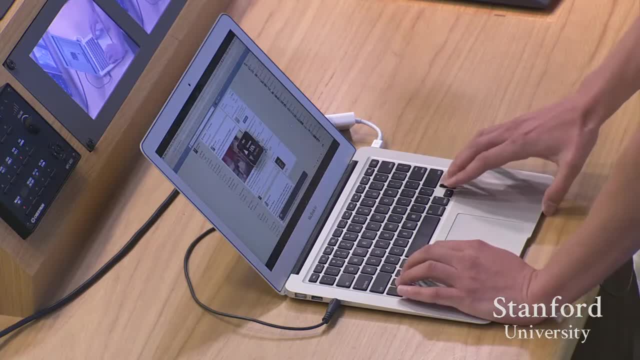 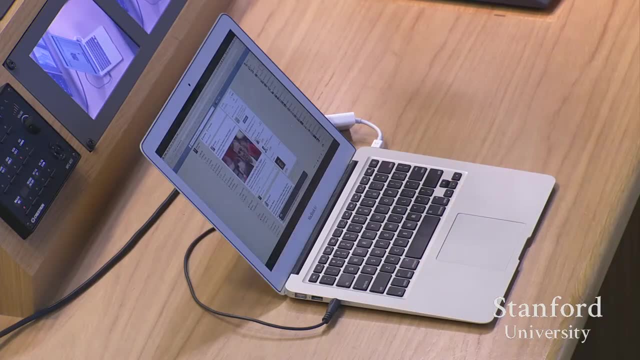 can sit here and listen. okay, anyway, i'll go back to something more. uh, nominal: 46, 36, 41. okay, tell me, this is too fast and um, we can switch. so i've got this screen, i've got this thing talking to me, so now you know i can. 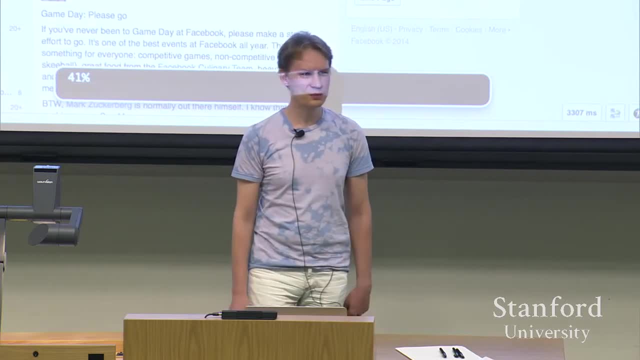 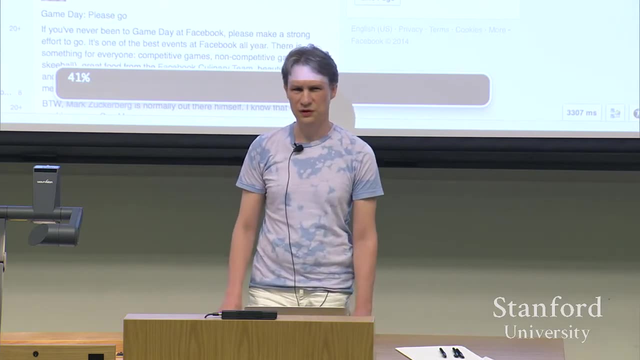 switch the speed. and again just want to repeat this because in the field of hci, super important to be personalizable, right, and so the same thing with the screen reader is a piece of piece of software and i want to be able for it to work for me. 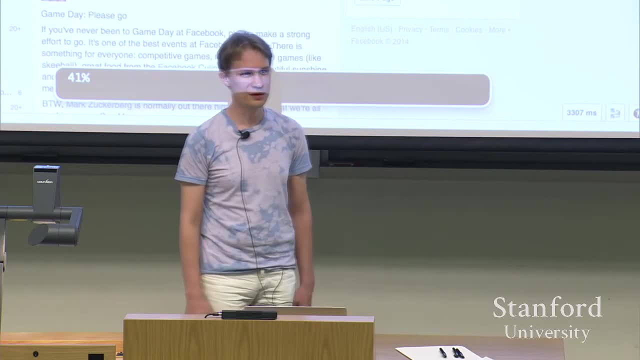 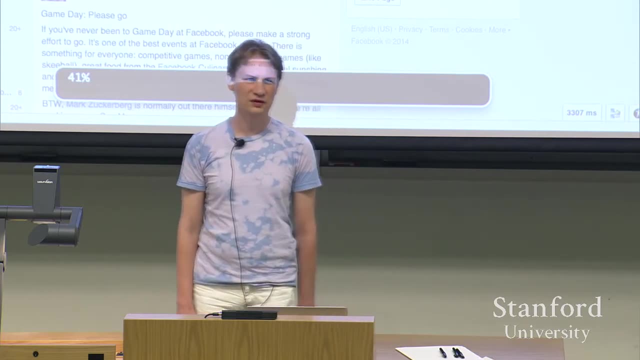 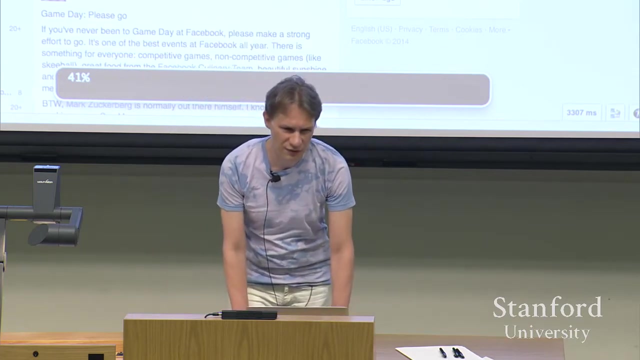 as opposed to me, work for it, right, i mean, who is the master here after all? so and so, so i set it to the speed i want, um, the other thing with speech synthesis you can do because, again, um, um, some voices are better, other voices are not as good. so with the screen reader i can actually go ahead and say: you know, 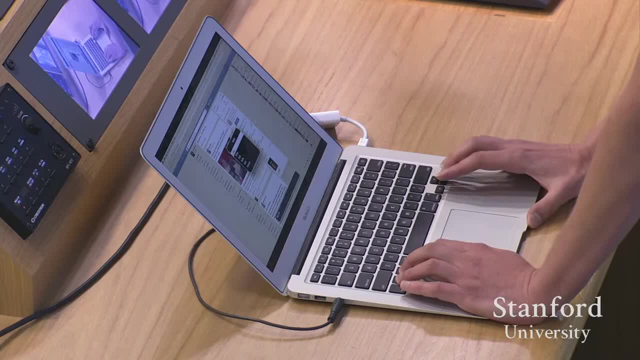 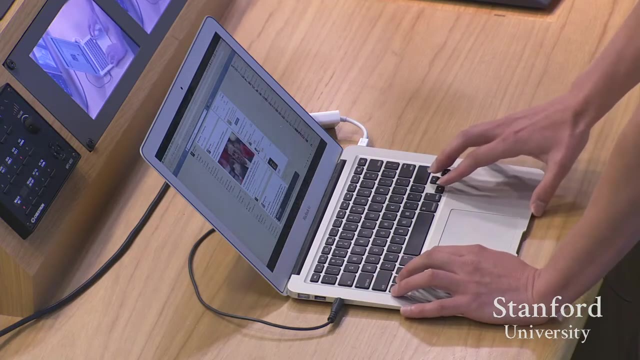 i pitch 50 rate voice, alex. i like bruce. different voice, fred. anybody here loves radiohead. alex, bruce, fred, they use this voice, i think, on their okay computer album personal folder. so if you don't believe me, go back, check it. it's pretty cool. 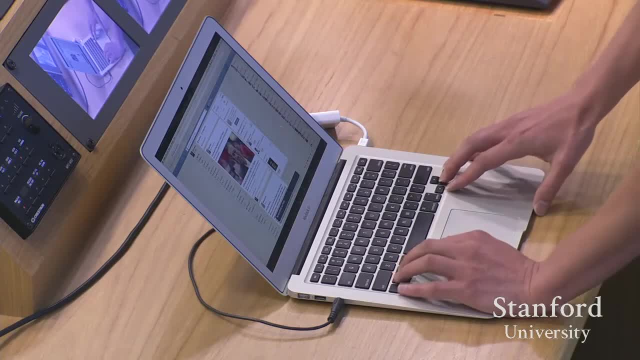 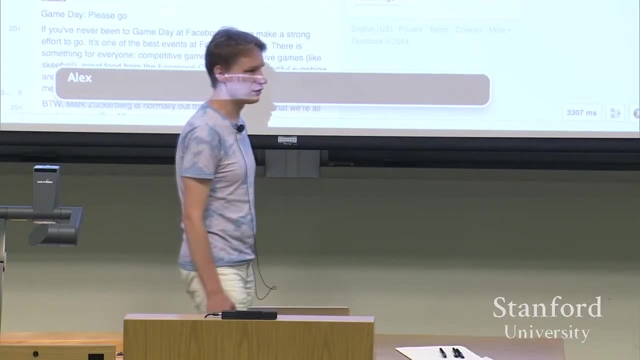 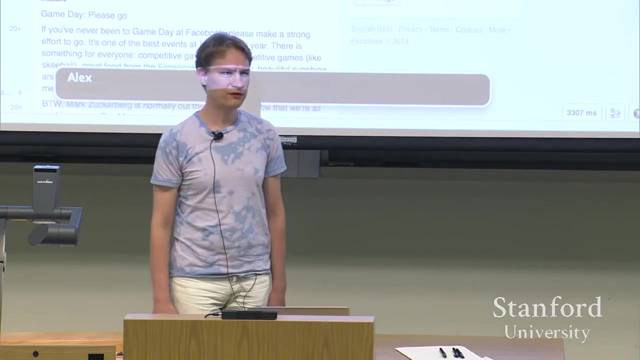 it's a very old, like mac os 9 or something like that voice, kevin, alex, anyway. so there are high quality voices. they're like sort of low quality and something in between. you can purchase them. uh, the most recent um mac os comes with like 25. 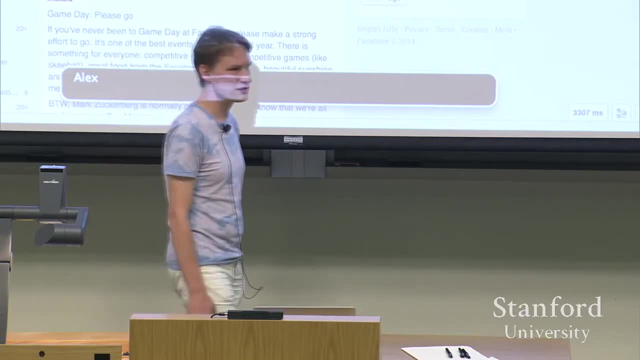 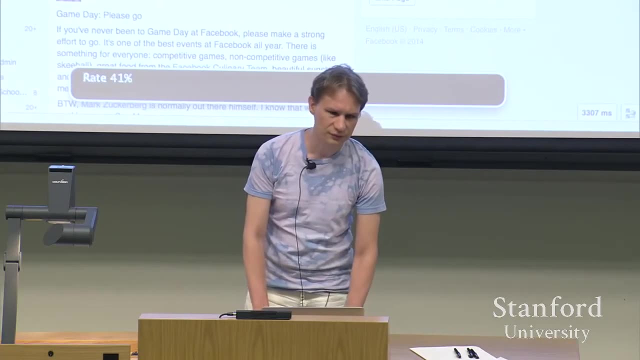 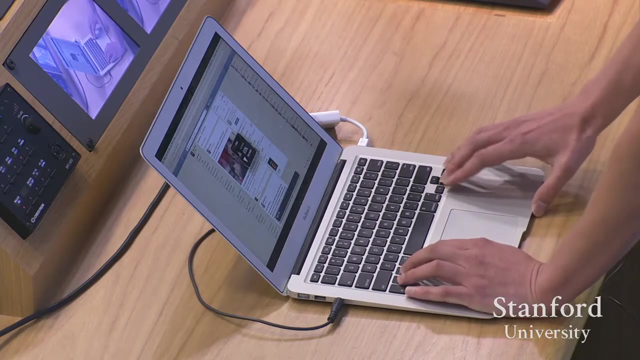 voices in 25 different languages and with different genders, and i mean it's amazing. you can really adjust experience any way you want. you know just the same way. um rate 41 pitch 50 percent, um. you can go and change the page: 75 percent, 40, 30, 15, 5. 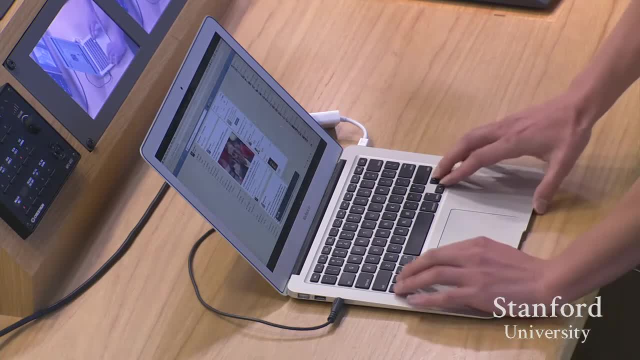 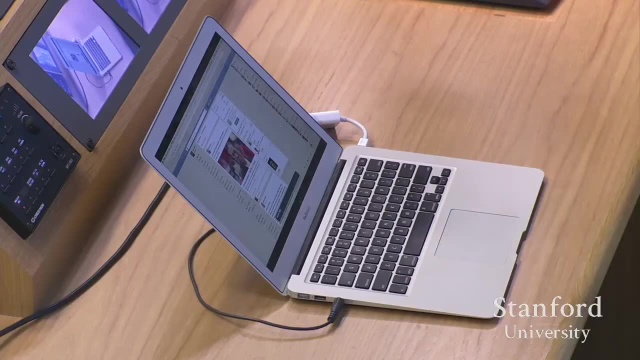 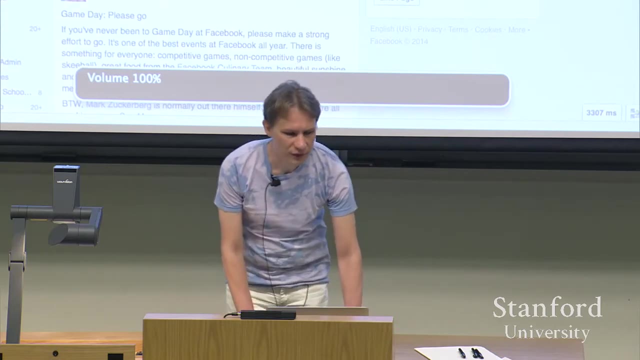 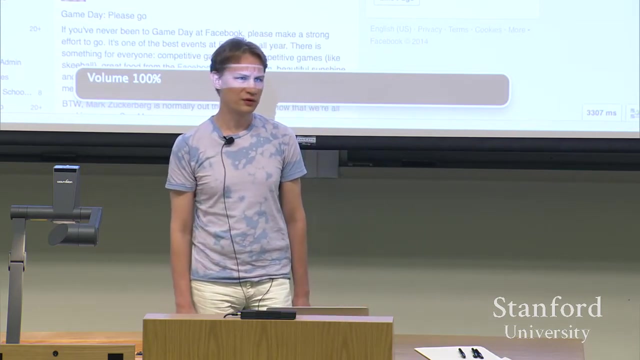 okay, this dude is really serious now. yeah, so 35, 50, volume, 100, and you know there's all kinds of other stuff, so there's volume and blah, blah blah. so, um, let's, let's do this. um, no, actually i'm gonna postpone this for for for a second. um, so, to navigate, uh, on on and, for example, on the dock or 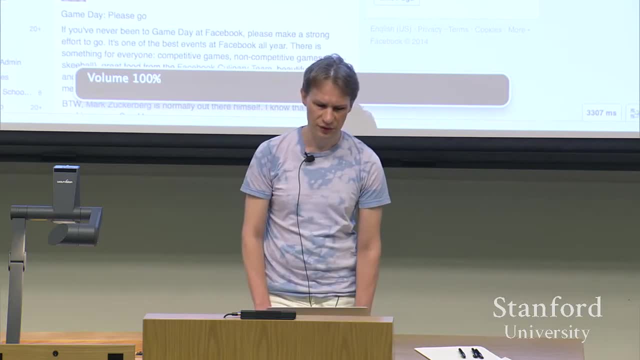 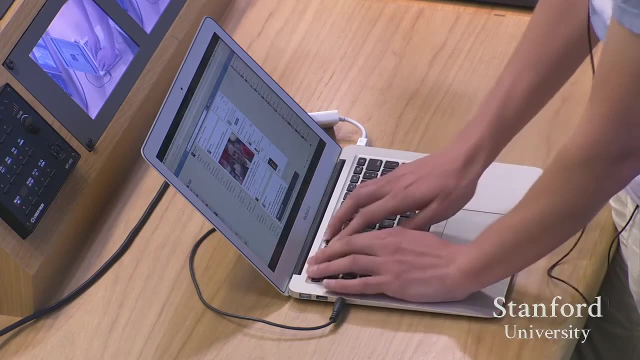 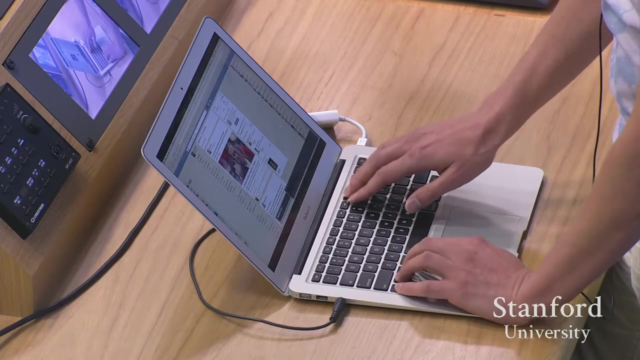 on desktop i would be using a tab key or arrow keys and i expect the screen reader to give me a feedback. dock finder: open one. uh, one thing about voiceover that you guys may have noticed already muting. let me just double check. if that's, show braille panel, hide braille, the voice over. quick start in this voiceover on. 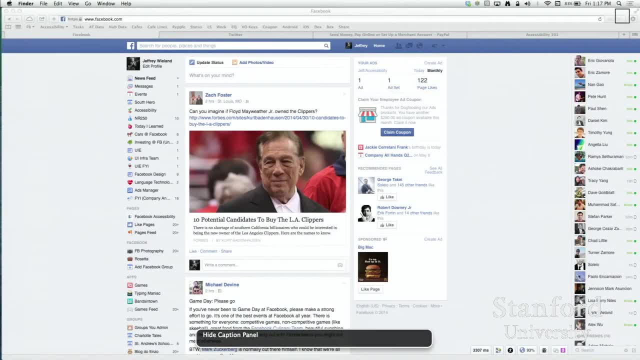 finder desktop hi caption panel. hide caption panel. oops, where's this caption thing? here we go. show caption panel. okay, i, i don't know, jeff, on your screen, where it appears on the left side, i think, is by traditionally where it is, you will, you will also see like a visual line that's telling you, it's telling you in. 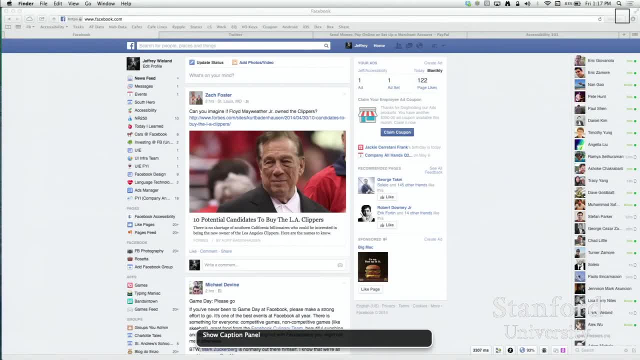 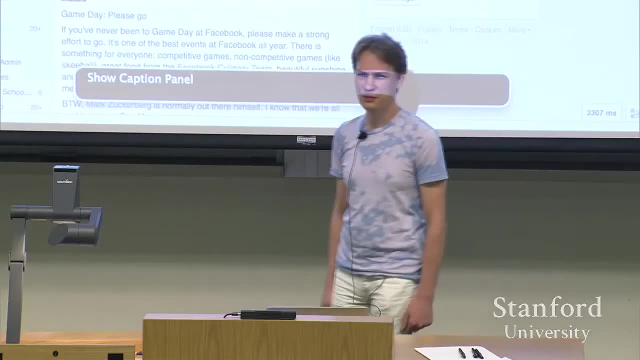 text what the screen reader is saying. don't assume that this is the behavior. this is just. apple is trying to be cool, which is great also for educational purposes, because if somebody is deaf and they cannot hear a screen reader, they can sit down together with somebody who is using the screen reader. 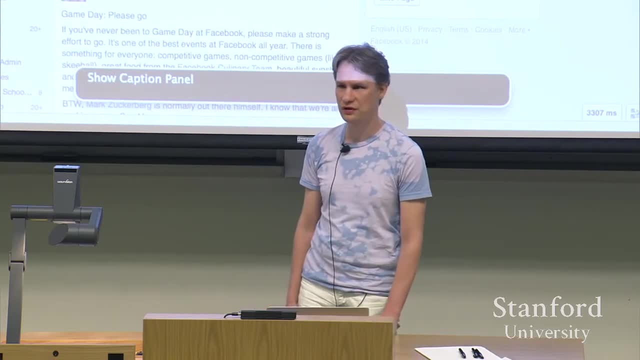 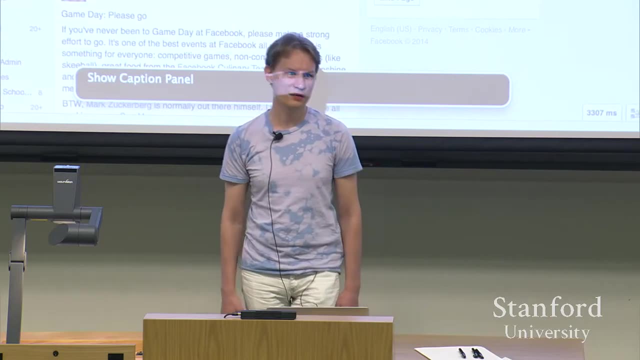 and being able to, you know, either work on homework together or just just interact or whatever. it's pretty nice feature, also great feature for developers, in fact. um, a quick story that i heard from this is authentic. i heard it from people who worked on voiceovers that 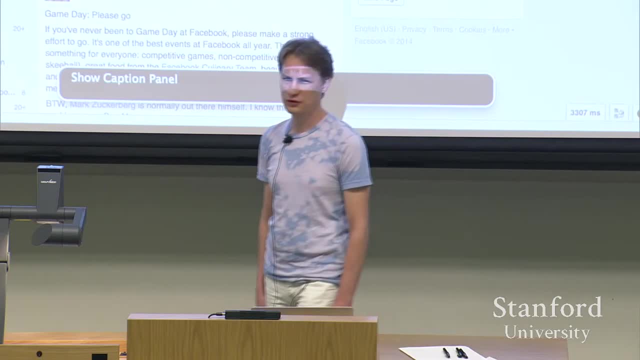 the way visual panel was born is that it was actually originally used for debugging purposes because engineers hated to listen to them and it's a big deal to me. so i'm gonna do it real quick and i'll quiz you guys on the real voice. so no, i'll just ask you guys the question right now. 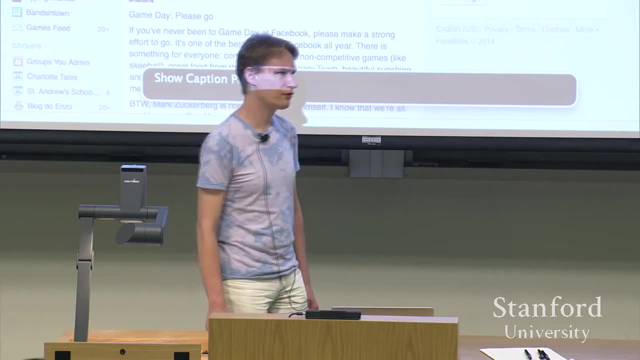 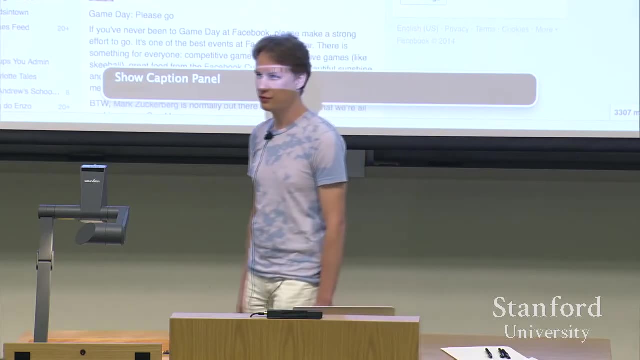 to these synthetic voices. And so they figured out: hey, why don't we just take the output of the screen and just put it on the screen? And then the product manager walked in and he said: what the hell are you doing? And I was like, oh, don't worry, it's going to be gone. 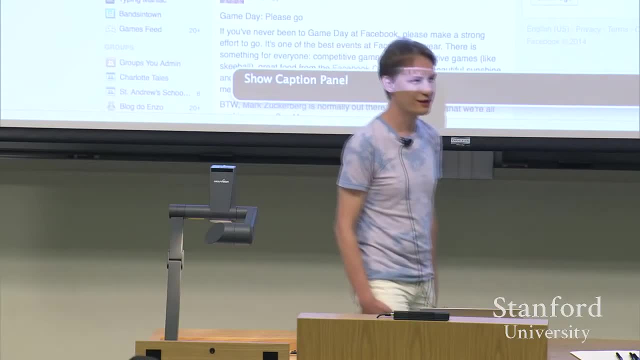 By the time we go into beta it won't be there. It's like, wait, wait a second, what is this? Oh, and then he looked at it. he liked the feature so much he said we're definitely going to leave it in the product. 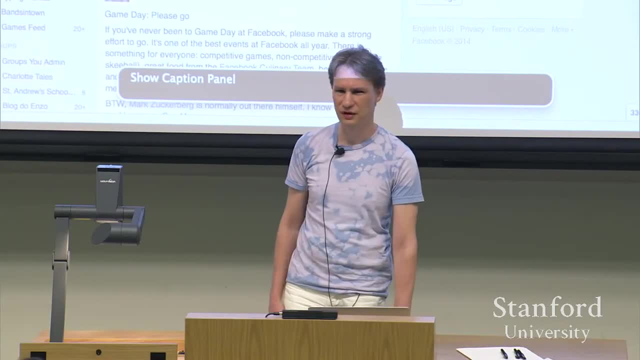 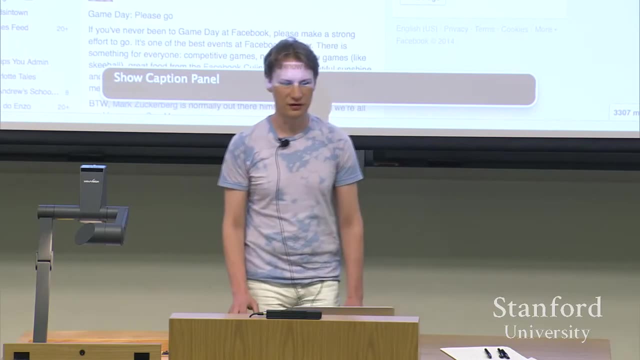 And so it ended up a really, really cool thing. Developers love it, And for you guys, when you start using the screen reader, maybe just something that's going to help make it easier for you to interact initially. So back to the dock. 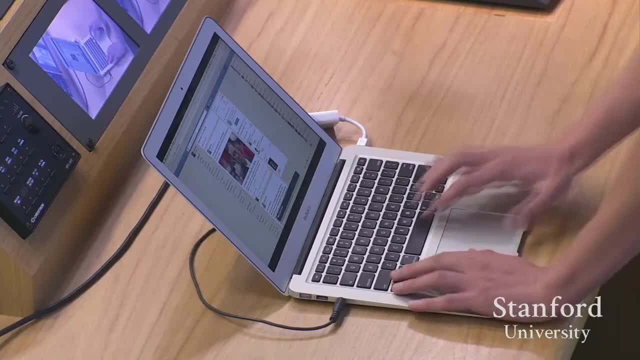 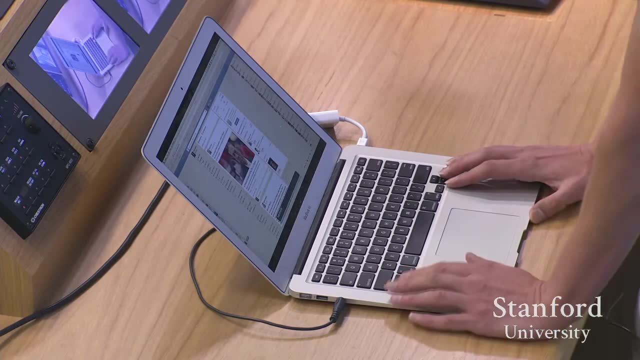 So I'm going to be using left and right arrow keys And dock. Oh sorry, he's got a vertical dock now. I remember Trash 20 of 20. So I'm using the up and down arrow keys to move between the items on the dock. 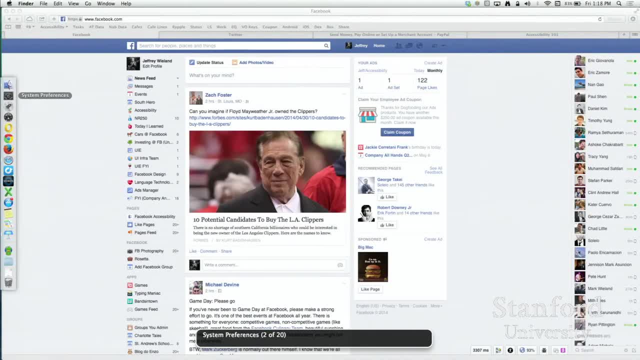 Finder: open: 1 of 20.. System preferences: 2 of 20.. Launchpad: 3 of 20.. Dashboard: 4 of 20.. So pretty simple, right? It tells you what icon you're on. 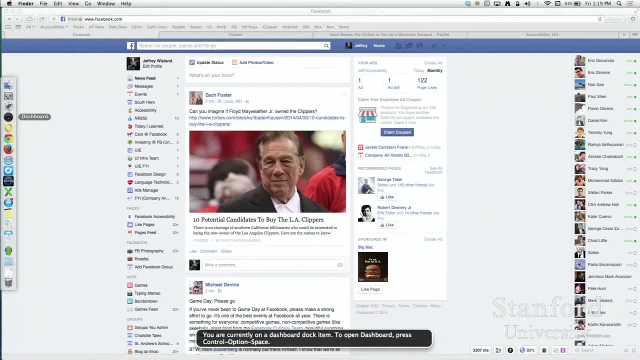 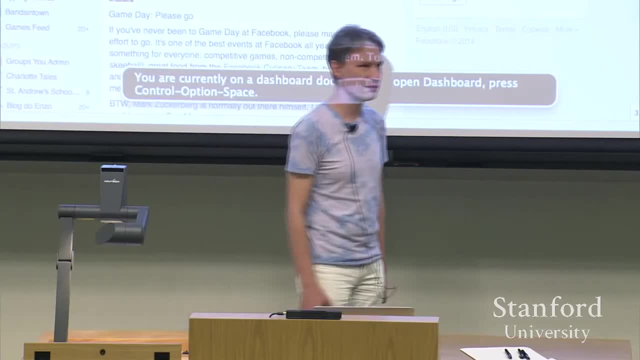 Anybody who is not familiar with-. You are currently on a dashboarditem To open dashboard press Control. Anybody else who is not familiar with accessibility can you? did you notice anything else except of the name of the icon when it was spoken? 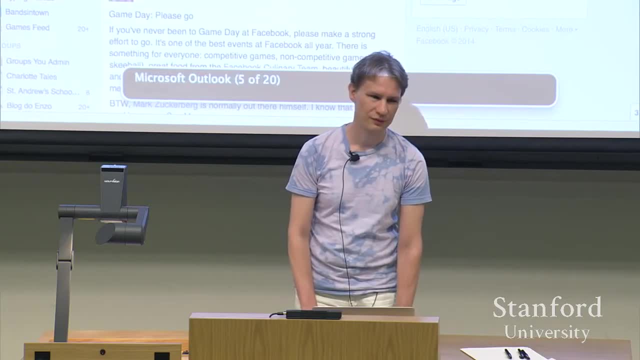 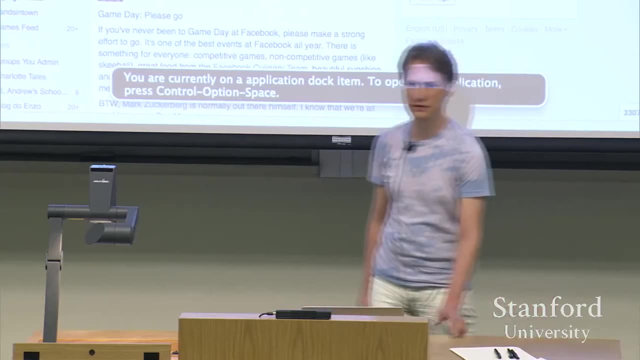 I'll give you one more hint: Microsoft Outlook, 5 of 20.. Anything So? you said Microsoft Outlook, and then it said something else. You are currently on applicationitem To open this application. 5 of 20.. It said Microsoft Outlook. 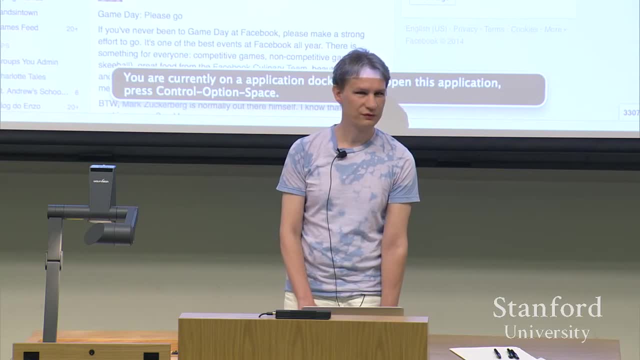 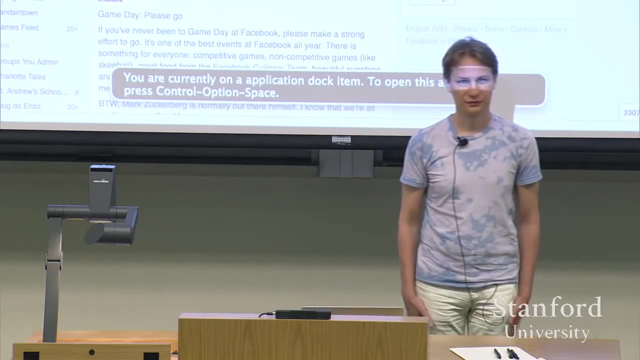 and then it said something else: 5 of 20.. Item number: 5 of 20, right? So why is this important to know? Come on, be brave. I know it's supposed to be a presentation, but you know, my presentations are always like that. 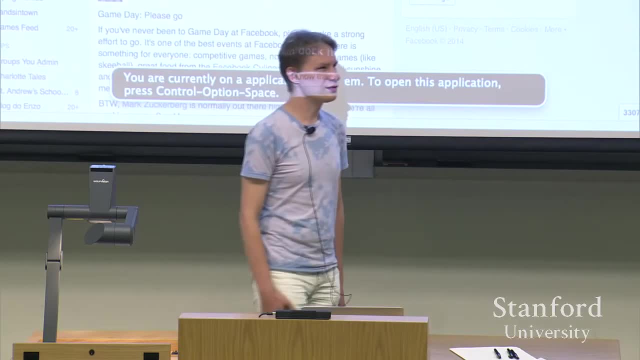 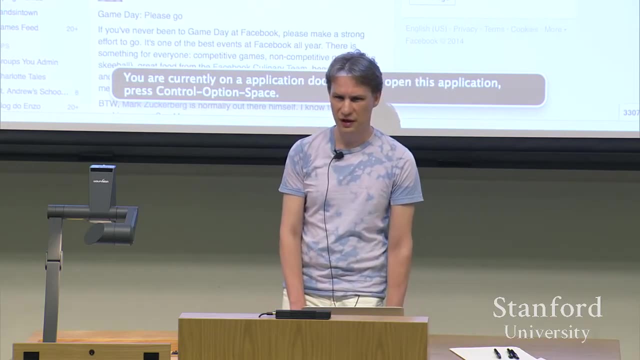 So in case you didn't know, So anyway, so the idea is to let the screen reader user know about the size of the control we're dealing with, Right? so in this case we have 20 icons and we're on icon number five. 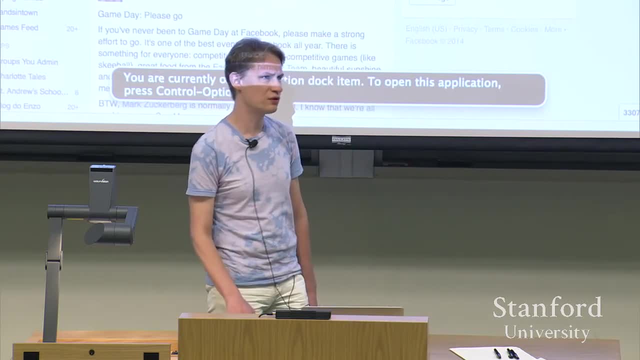 So it does help you to get oriented a little bit. So if, in case, you know that your mail icon is at the beginning of the dock, you know you're not gonna go to item 19, and then you know, wrap around. 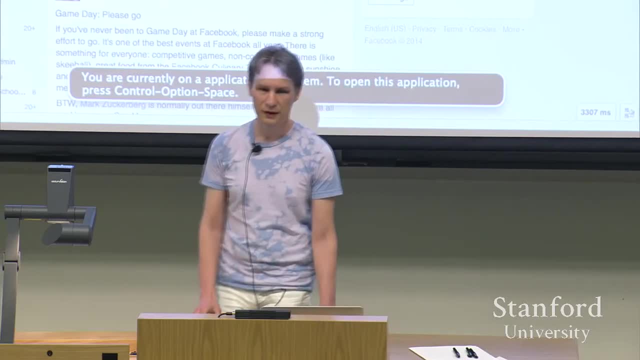 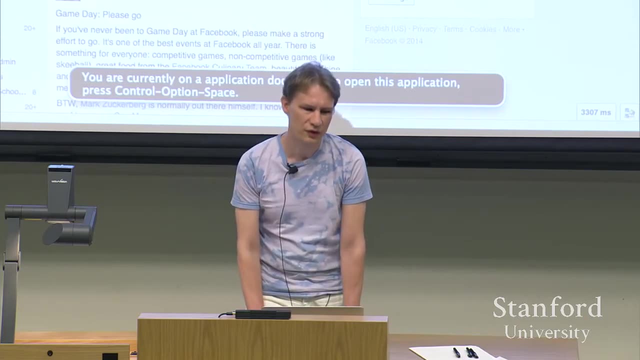 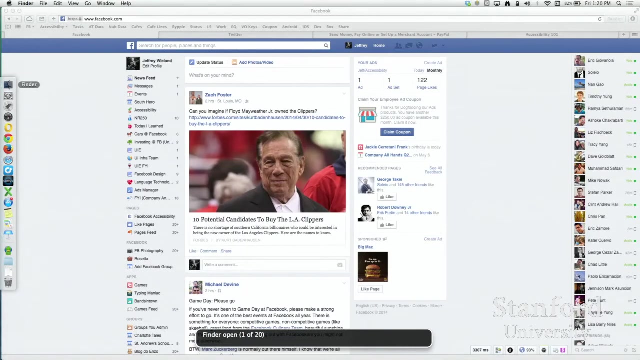 but you're gonna go backward because item one is closer to five. So somebody clearly thought about that kind of stuff and you know it appears to be very useful Before we get off the dock. Dashboard Launchpad System. Prep Finder- Track Finder Open: 1 of 20.. 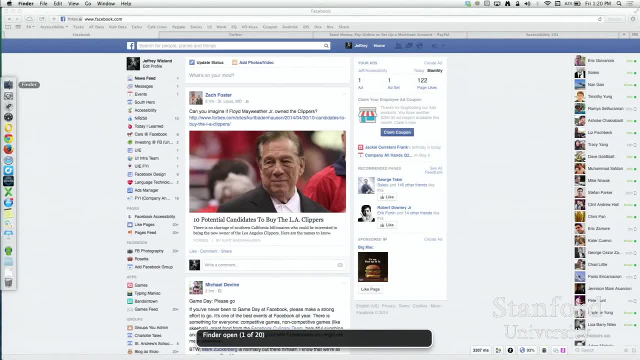 What about this one Finder? did you hear what it said? You are currently on application dock Finder Open 1 of 20.. It said: Finder Open. That's pretty neat, right. You are currently on application dot item. 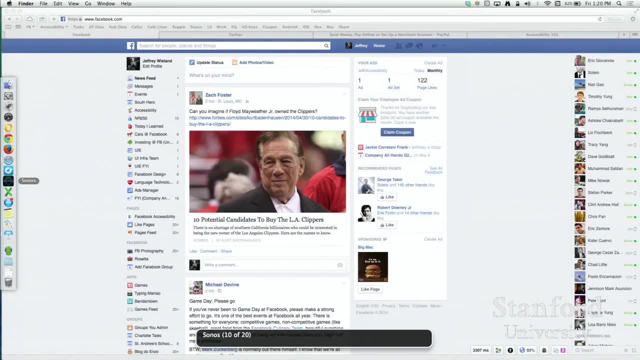 To open this application If I went to Safari, Open 8 of 20.. As opposed to Firefox 7 of 20.. It's pretty cool, right? So it tells you which of the windows is currently open. so 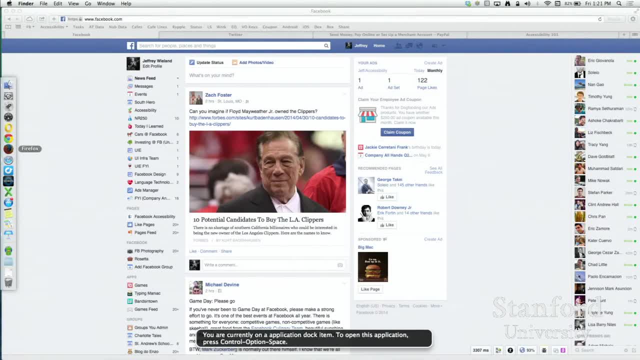 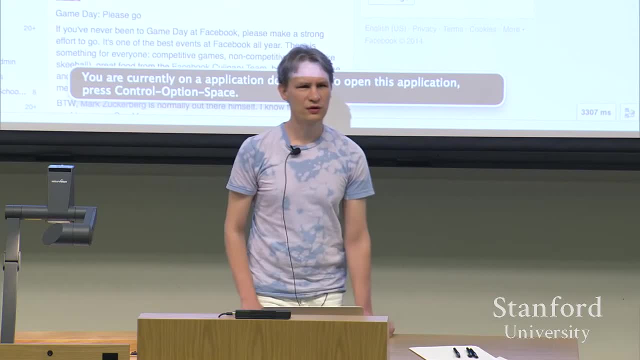 You are currently on application dock item. To open this application, press. Yeah, this is what happens when you're in beginner mode. It gives you all these hints and stuff. So this is pretty cool, right Again. great for somebody who cannot see. 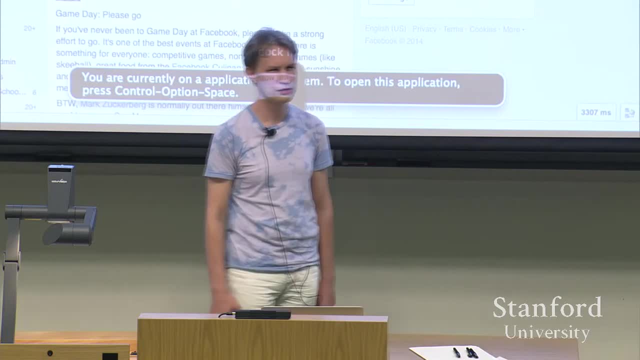 because for you guys, you take this for granted. You look at this screen. you're like: oh, I know which windows are open, right For me, I can go. I can have to go. I have to go through each of these elements. 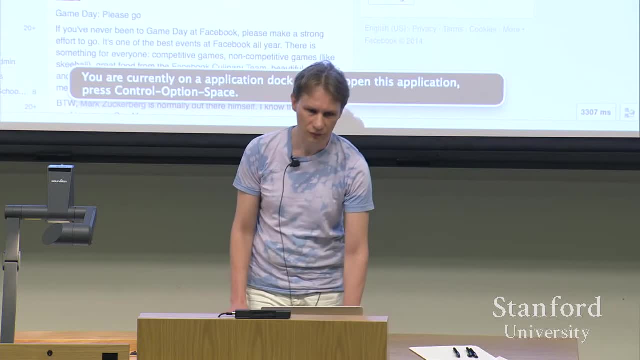 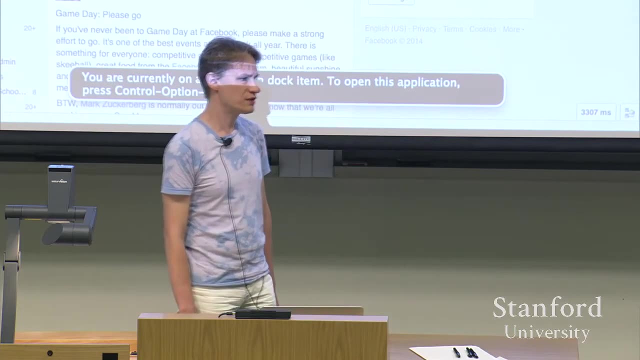 and trying to figure out. so what exactly is open? Okay, let's move on One step further. So there comes a time where arrow keys and tab keys aren't gonna do, because you know you need to be doing more complex operations. 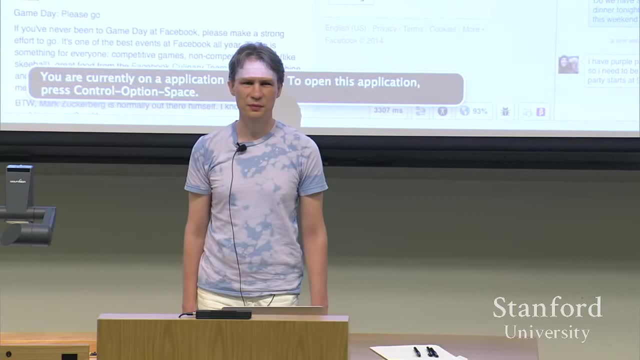 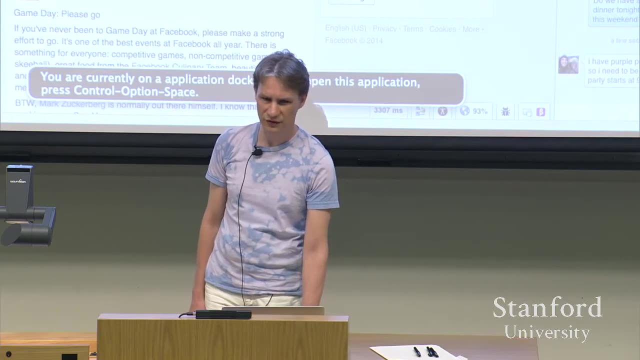 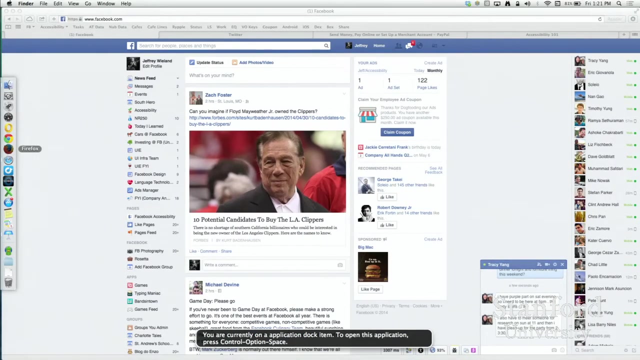 than just moving between your items. So, for example, you need to be able to switch between windows. So we know that there's at least two windows open on the screen- Finder and Safari. So so rely on me. Command tab is gonna allow us to move between windows. 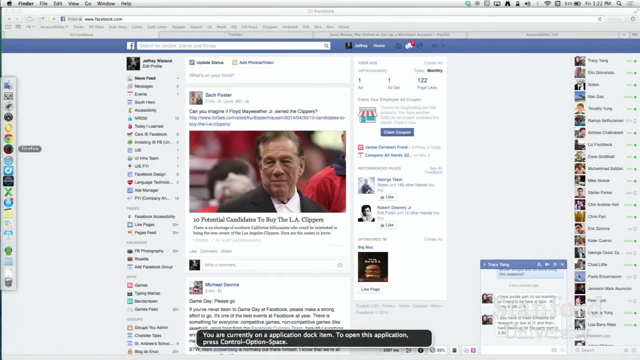 So that's a built-in Mac shortcut key we're gonna use. Let's see what happens there. Safari Keynote Finder. Safari Keynote Finder. Okay, cool, So there's actually one more window open right, Which is Keynote his presentation. 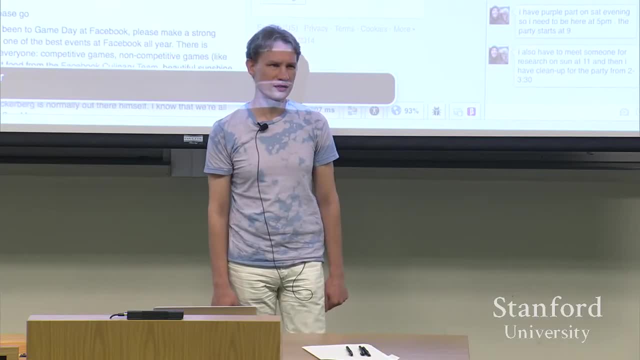 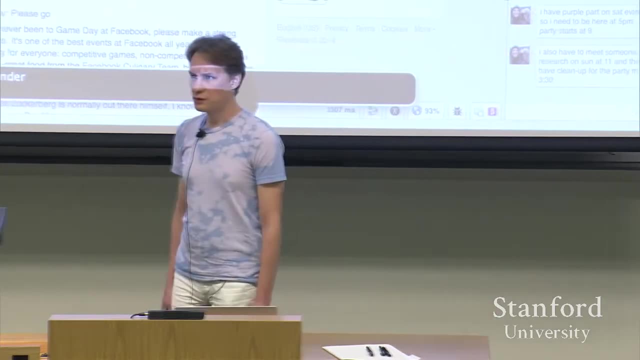 So how do I know that the Keynote is open? There's a window. you notice, there's a title in the window. Every window has this title area where it tells you what the name of the app is, Especially on the web. we'll see instances. 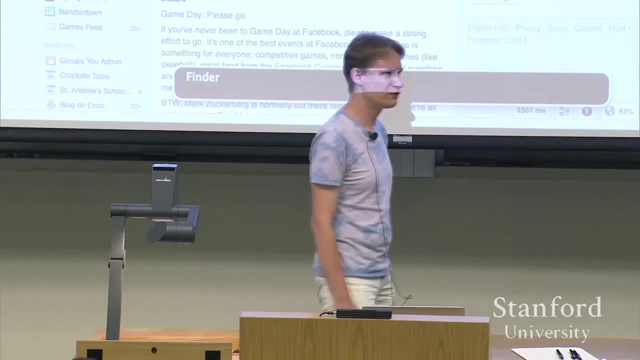 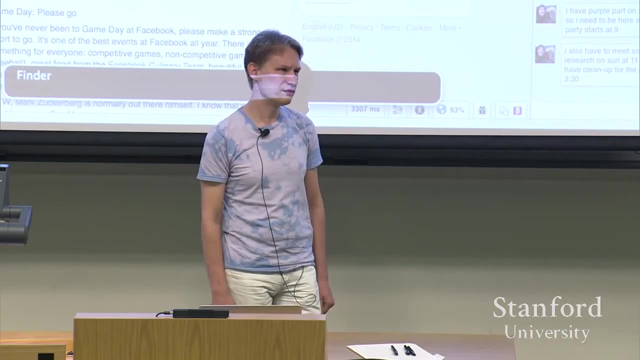 where people forget to put the title. And so when you move between tabs in the browser or you move between windows, and if there's no title there, then obviously, as a blind user, you have no idea what you're talking, what you're interacting with. 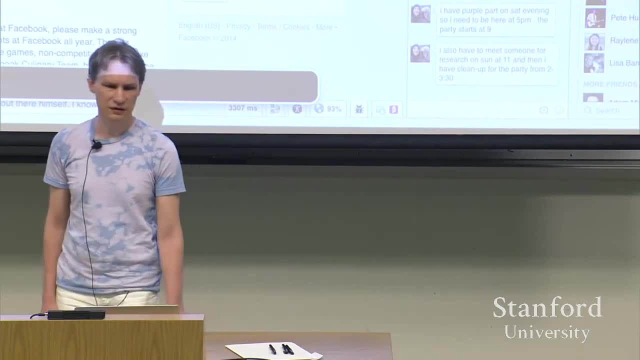 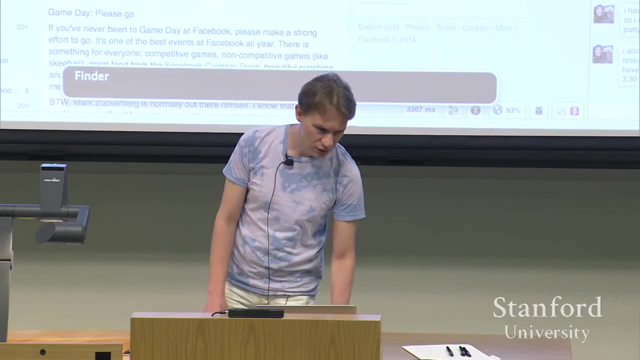 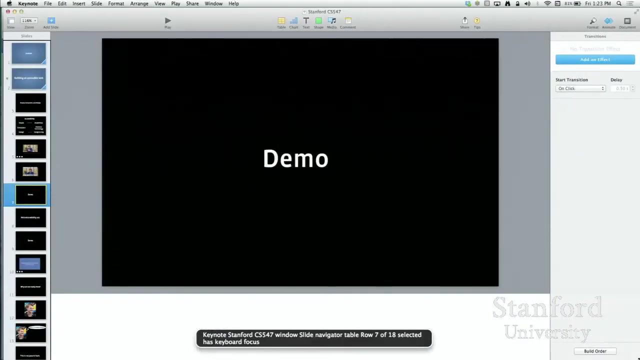 So simple thing like title in your window gives a metadata for a screen reader to announce something useful. Now, interesting enough, in Keynote's case, Keynote, Stanford, CS547, window slide nav, That's cool, right. So I know what presentation he's showing us. 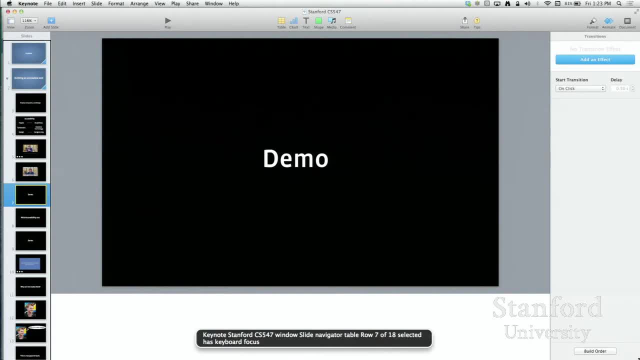 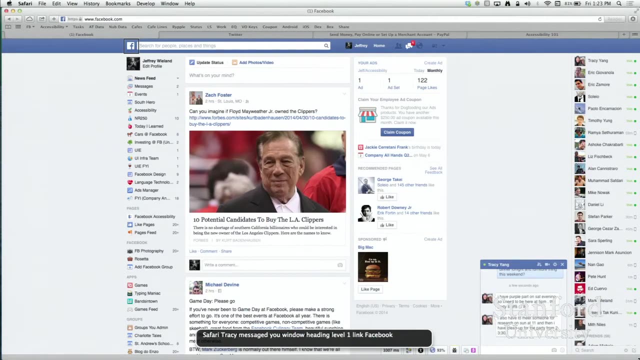 what presentation Jeff has opened. So this is nice without having to do anything, because the title is communicating to me the name of the document: Finder Safari, Safari Tracy messaged you window heading level one link base. Cool Yeah, my fiance is trying to contact me right now. 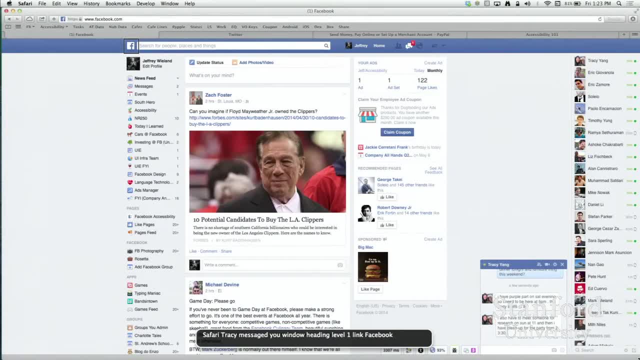 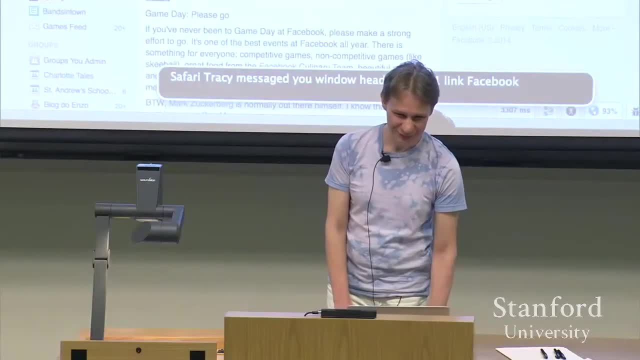 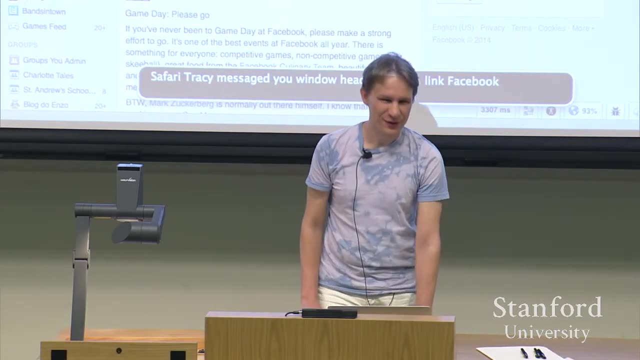 Okay, He's great. Hopefully he says nice things. Okay, Yeah, Uh-oh, Hopefully he says nice things. Yeah, he's here. Yeah, don't provoke me. So, okay, cool. So, as you can see, the context is very important. 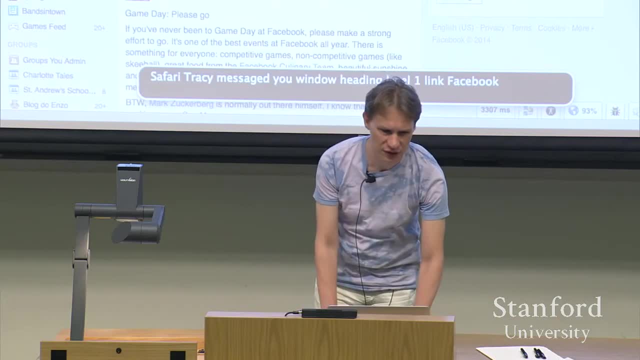 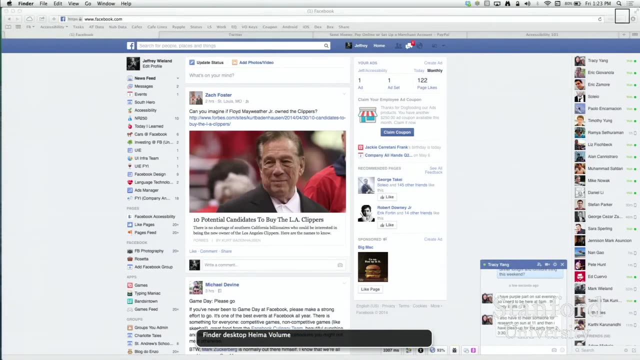 These are the title of the window and sort of to finish, the desktop Keynote Part of this presentation: Finder Find. Similarly, you know, if you go to the menu Menu bar, Apple Finder. I'm just using arrow keys right now. 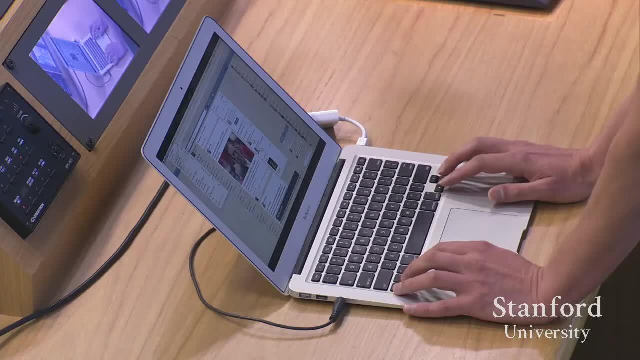 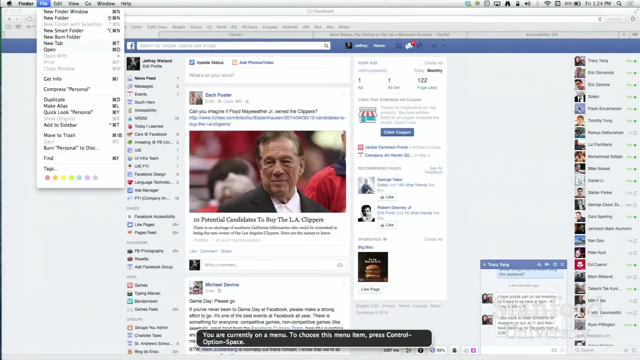 File. Okay, so I found the file menu. File menu: 25 items. You heard that before, right, So it informs me that there's 25 items in the menu. You are currently on a menu. To choose this menu item, press control. 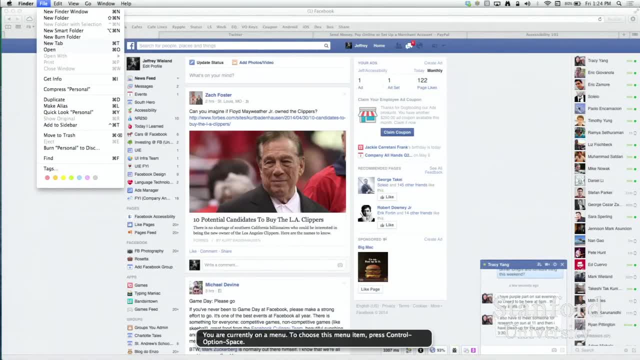 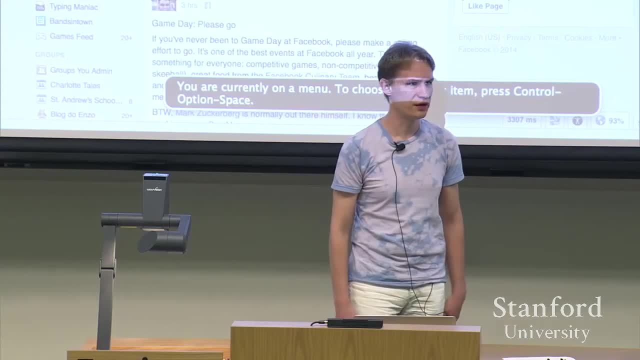 And a lot of the other transactions you would be doing with the keyboard. through the keyboard would be pretty much what you guys would be used to: Enter key to activate stuff. You know enter key to activate stuff. You know arrow keys to move left and right. 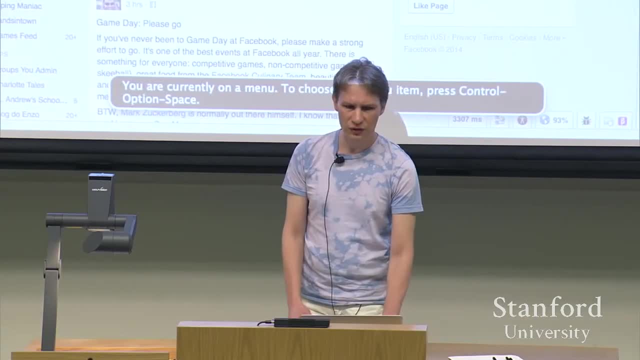 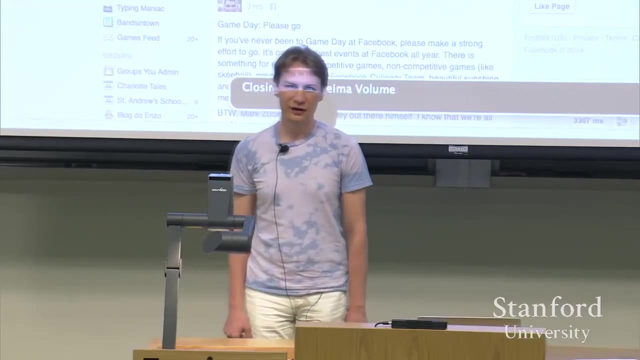 up and down and so on and so forth. So what I want to do is I'm known to go over time and I didn't ask anybody to alert me when the time is All right. So what I'm going to do is move to the web a little bit. 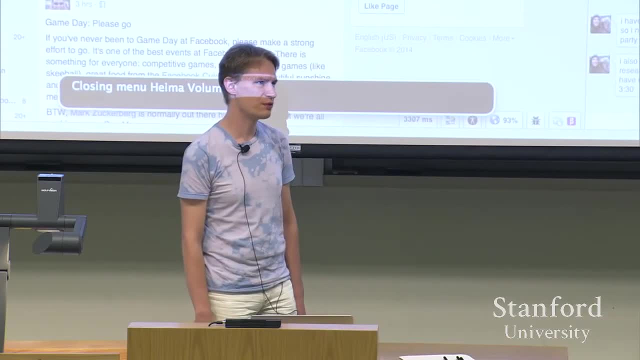 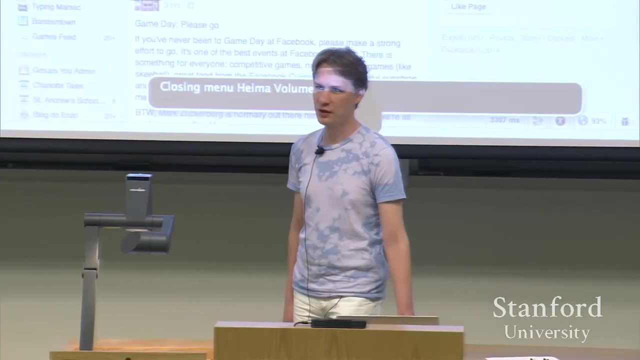 to talk about the web, and then we're going to move into the topic that excites me personally, because I worked a lot on mobile stuff and that is really, you know what gets me going. It wakes me up in the morning, Literally. 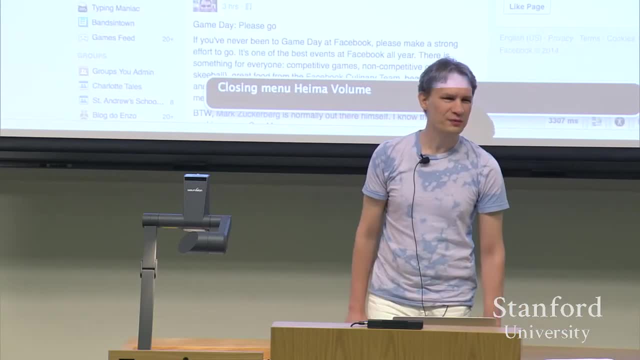 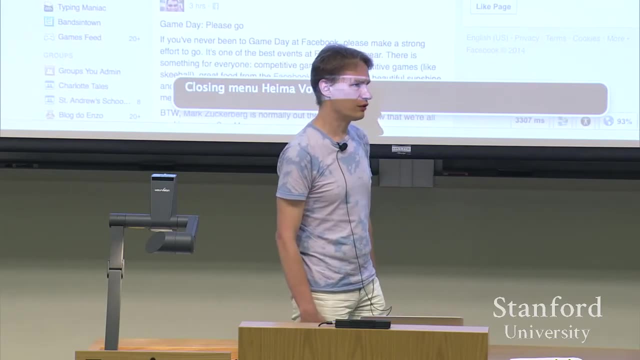 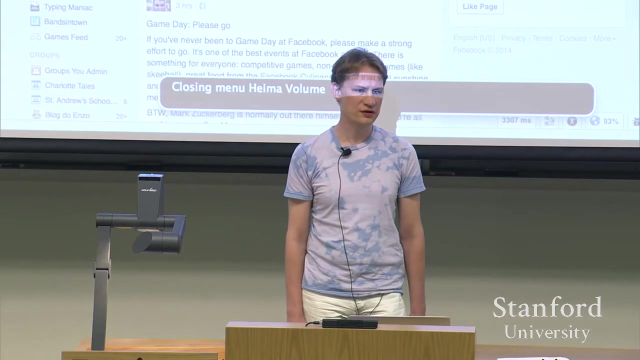 Anyway, OK. So on the web, similarly just like we have on the desktop, we have to interact with the web page mostly- well, not mostly, but by default you will be using the tab key to navigate. That will move you between focusable elements on the page. 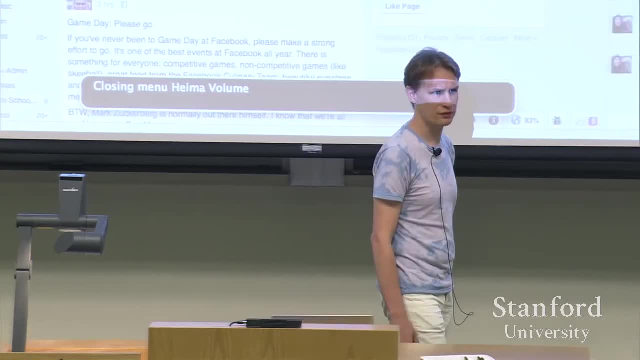 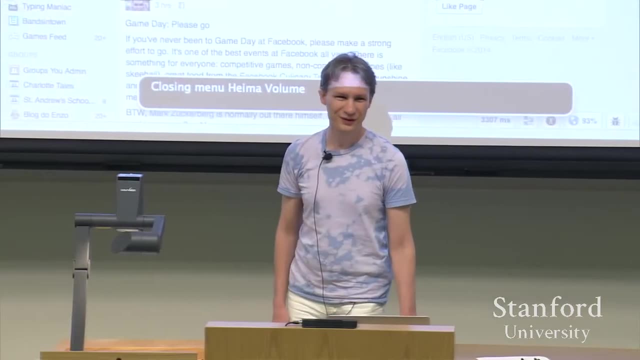 You will hear the word focus, especially those of you. how many programmers, by the way, are in the room? Are there any developers here You want to applaud? Not to me, Not to you, Not to yourself, OK, Good. 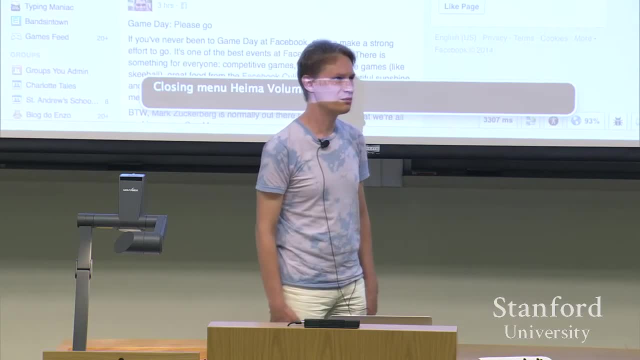 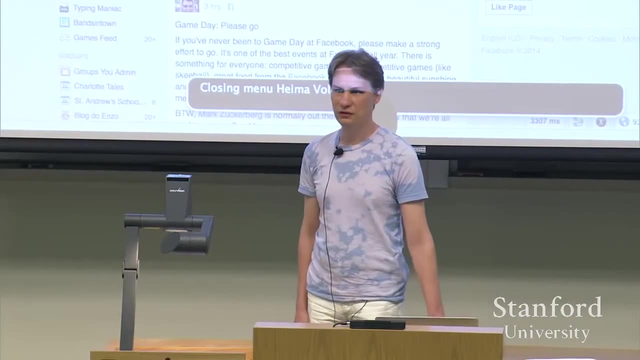 Awesome. OK, So there are some developers. So you hear the word focus being mentioned in the context of accessibility. many, many, many, many many times focus events. you know object under focus and things like that- Very important. 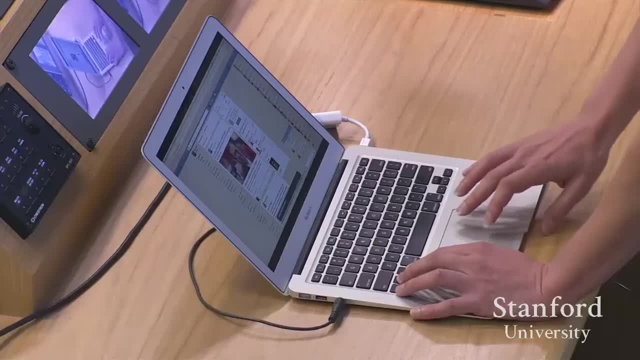 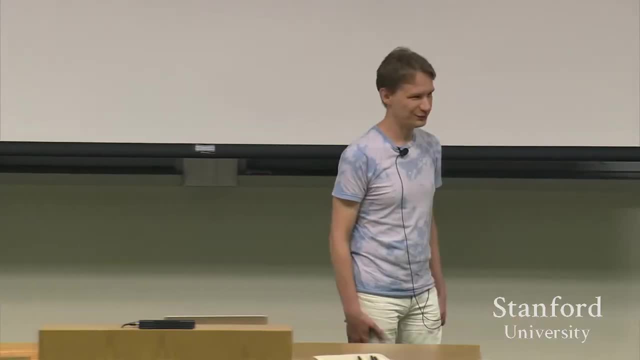 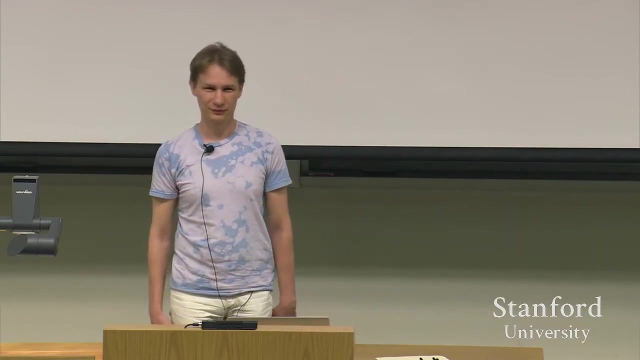 Why it's important. Trackpad Screen curtain on. OK, So I'm here on this web page and you guys don't see anything. right, Me too. So how do you know where on the screen I currently am, Anybody? 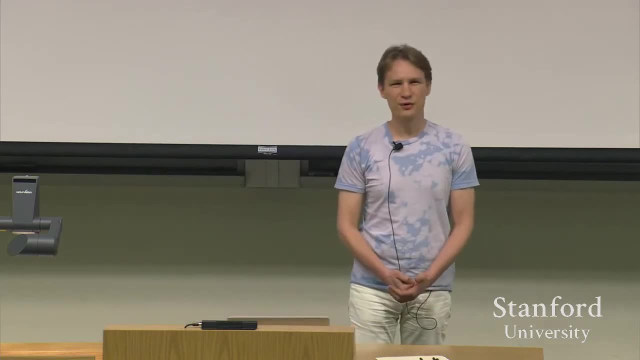 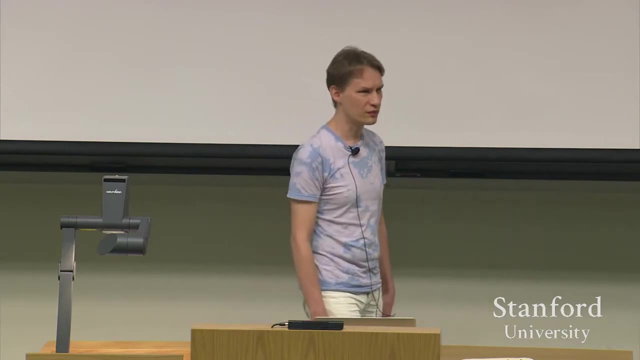 No, of course I know I'm just tricking you. It's impossible, right? Because now your contextual information is gone, Your two-dimensional vision is gone, And so what you're stuck with is what I call is one-dimensional vision. 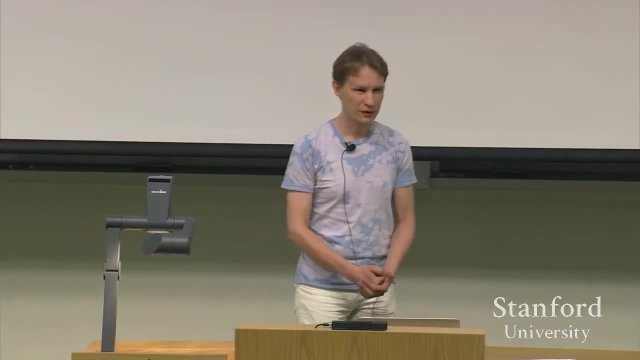 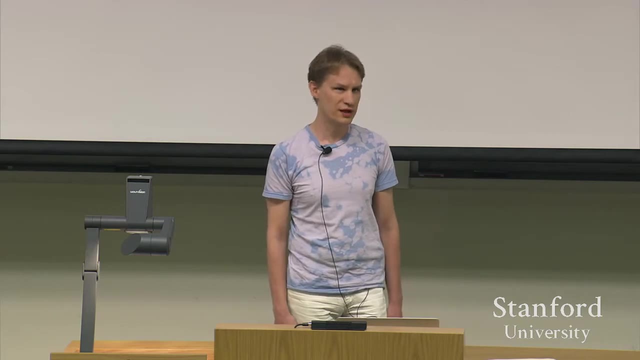 And that is basically a linear way to interact with the computer. OK, So let's talk about this, OK, OK, Luckily, the situation has changed a little bit with the introduction of touchscreens, But on the desktop we're still largely 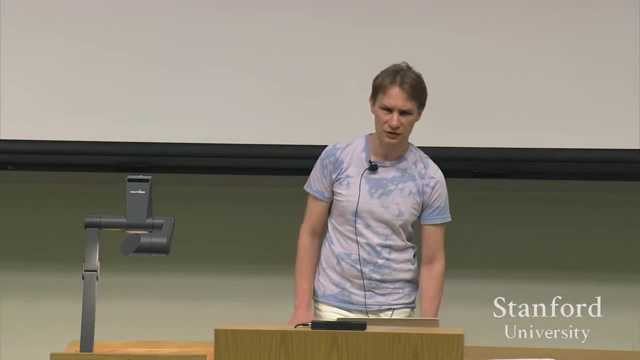 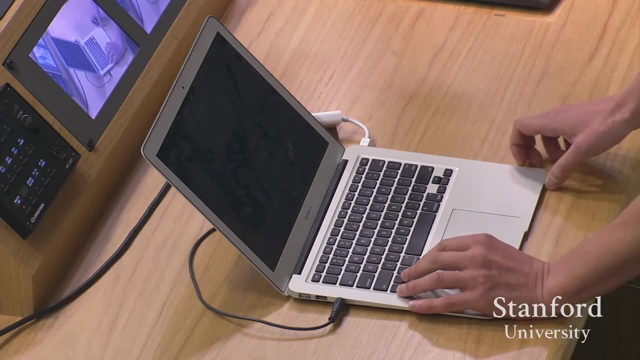 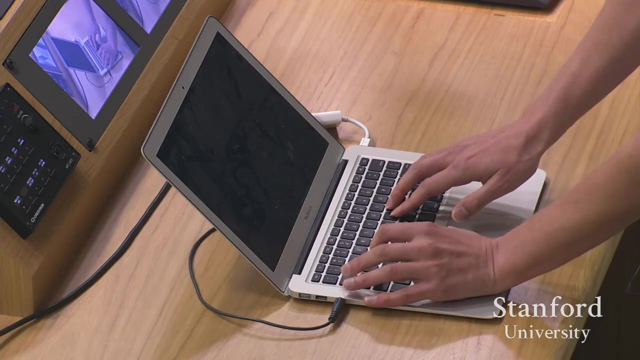 talking about one dimension, especially as far as the keyboard is concerned. So let's say I took you to a page: New tab. Now in all my questions for Jeffrey: Microsoft Word, document, Safari, Safari, new tab, untitled, search, Google or enter an address. 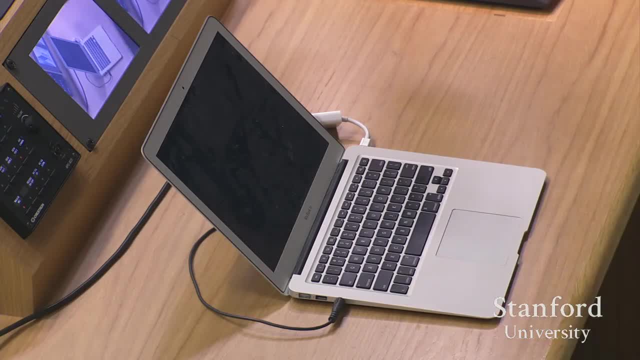 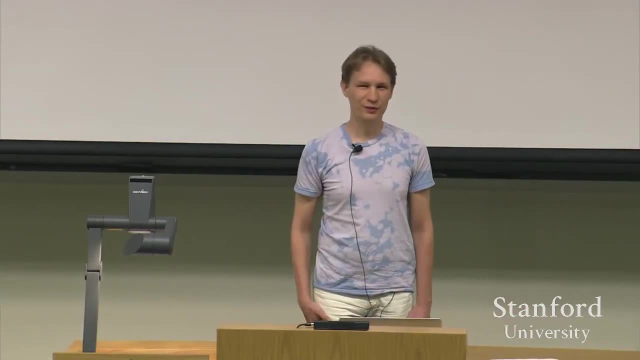 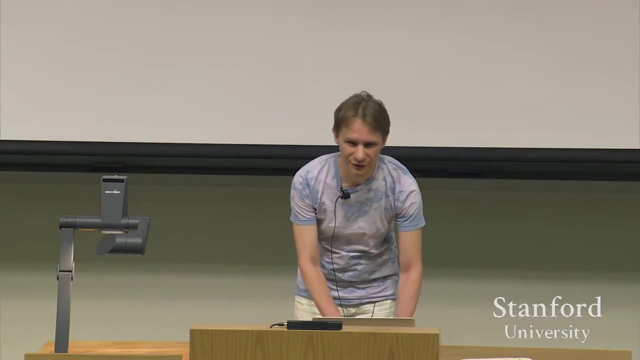 Address Search- Edit text. Where do you think I am? You are currently on a text field inside of a toolbar. OK, Google? Yeah, maybe, But that's only because Google is built into the browser, But I'm actually on the address bar, right. 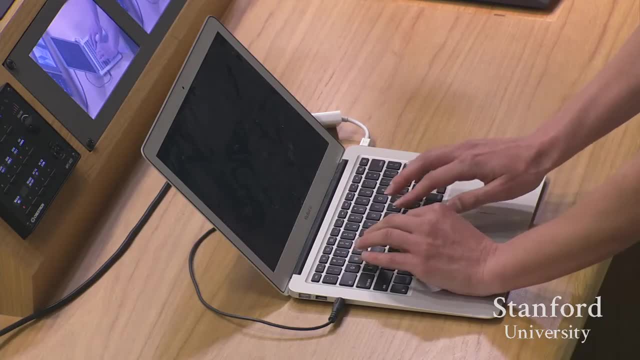 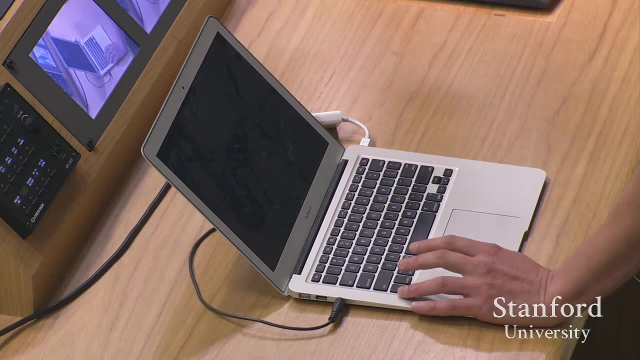 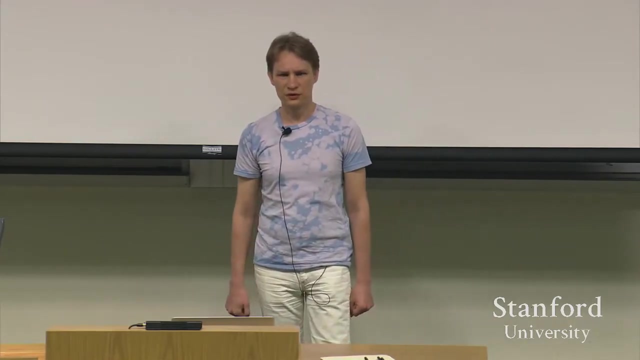 That's a fair guess. So let's do something. Open location Period M: Unhighlight. OK, Which page do you think I'm on Visit link? You wouldn't know, You wouldn't know. So this is the typical experience of somebody who is blind. 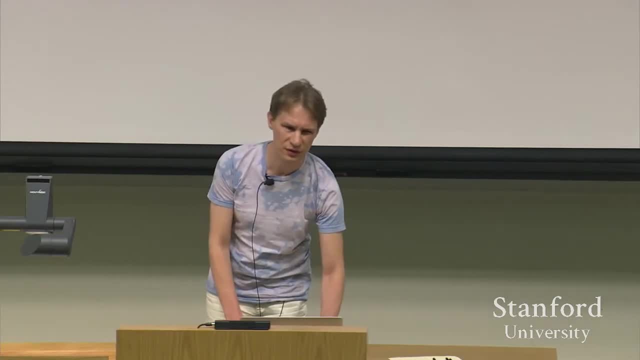 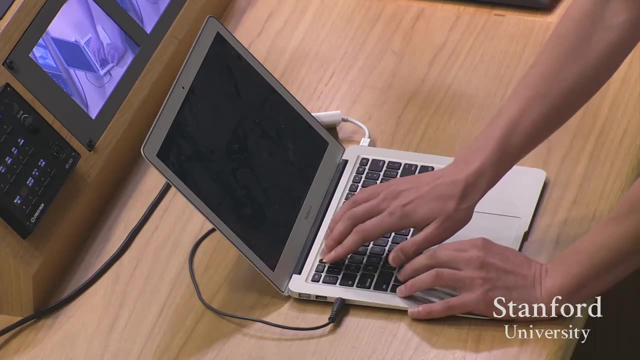 I'm going to refresh this page so you guys can actually hear the title of the page And this way you will know. Reload page: CNNcom- 87% loaded Visited link image: CNN List four. Screen curtain off. 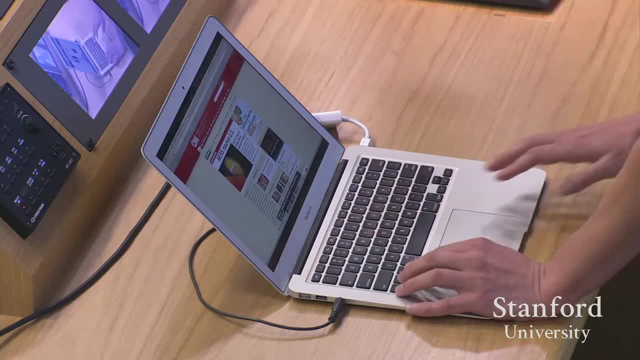 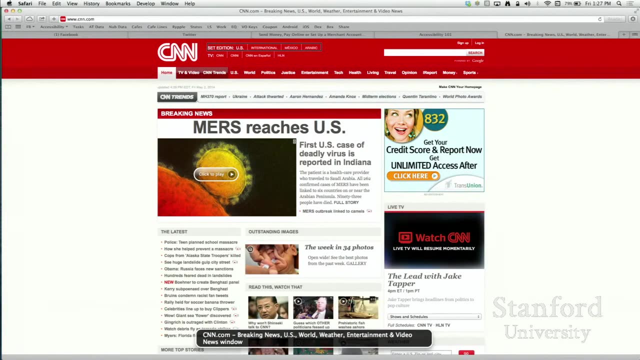 Display bright, Brighten. CNNcom Breaking news- US World Weather, Entertainment and video news Window. So that's the title of the page. OK, So you kind of know that I am on CNN, CNNcom, right. 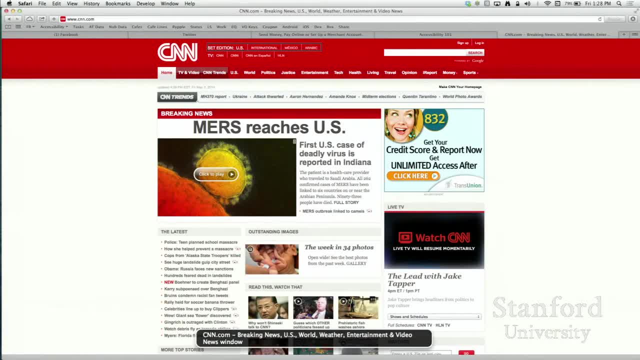 What else do you know about this? Not much, because we're right now on the page And I, as a blind person, have no idea about things on the left, on the right, I have no idea where those stories appear. So the way I deal with this situation, 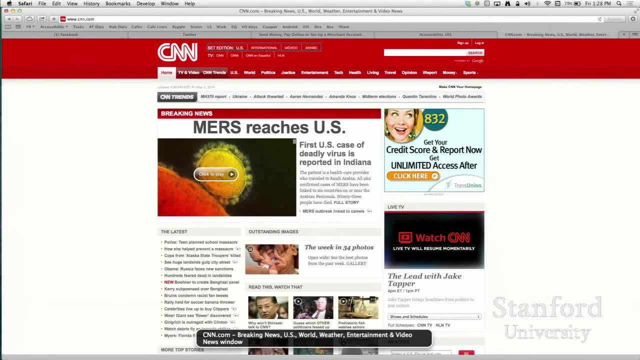 is that you start gathering, You start mapping out the screen little by little, So you start tabbing Link Link International, CNN International. Link Mexico CNN Mexico. Link Arabic CNN Arabic. Link TV List five items: 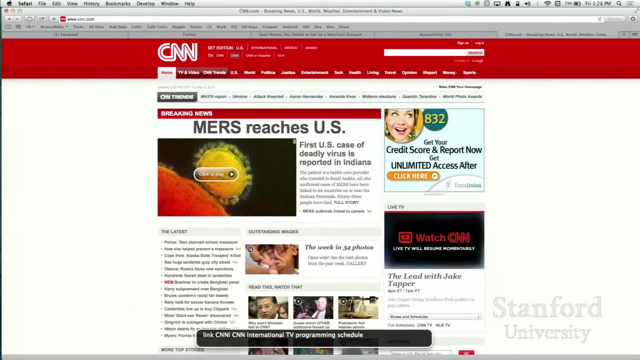 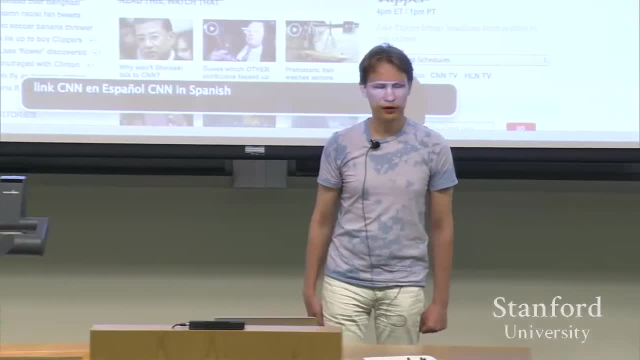 Link CNN, CNN TV program. Link CNN Me CNN Inter Link CNN On Air. OK, Before you fall asleep. so we're going through some kind of toolbar, right And so, if you just imagine, I'll let you use for the rest of this exercise. 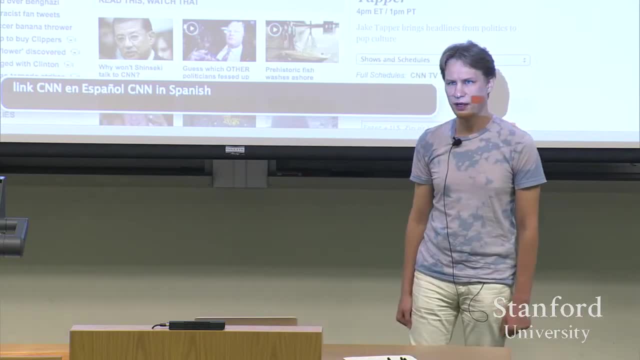 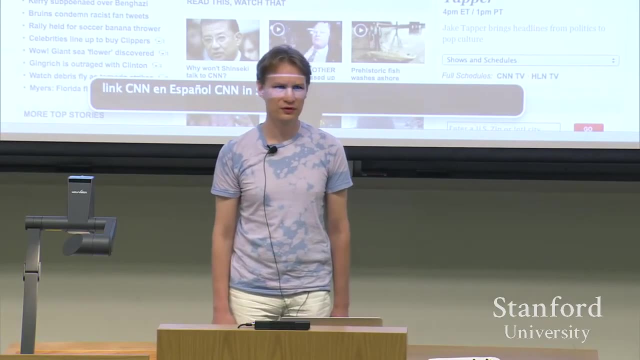 let you just use your imagination. You literally have to go through the page. if you're a beginner especially, You have to go through this page. It's like looking through a straw. You know you slowly move a straw across the screen. 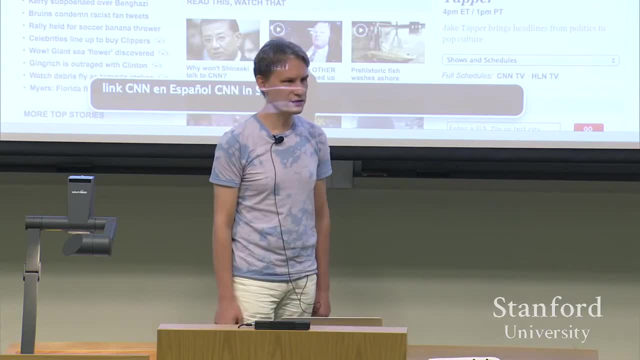 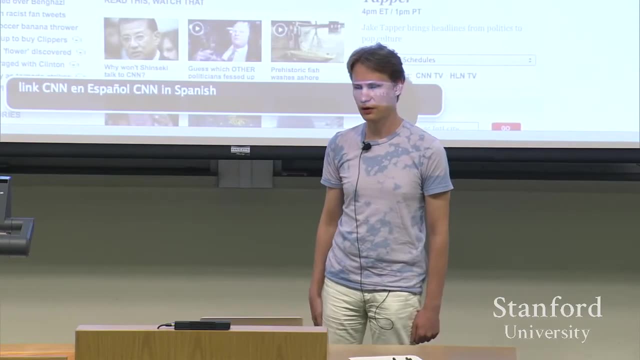 You're like: oh OK, Now I start getting it. So on the left side or maybe first comes the menu bar, then second comes, Eventually we're going to get to top stories And then we're going to get to probably some kind of advertising. 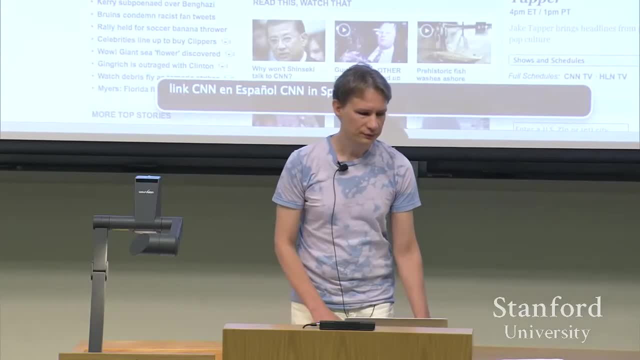 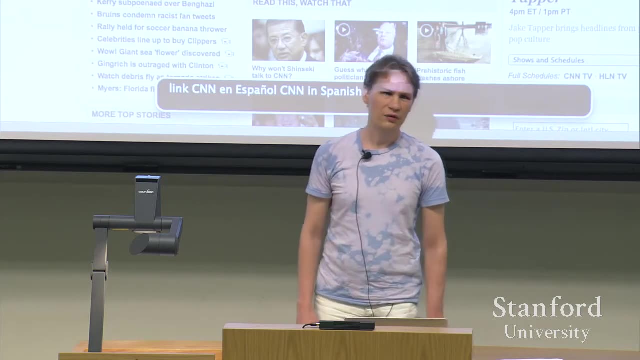 And then we're going to get to some kind of footer, right. So this is basically how a screen reader user works to learn about web page. Now we have this language. Hopefully I'm not going to steal thunder from Ramiya. 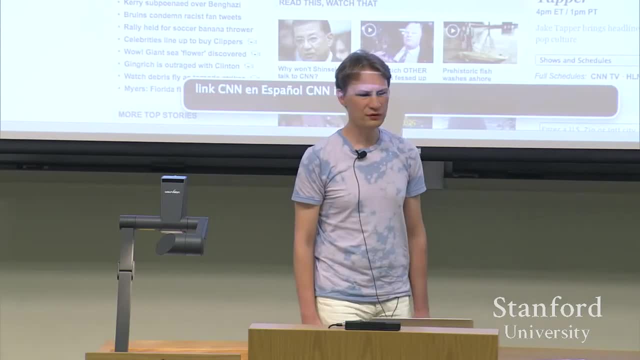 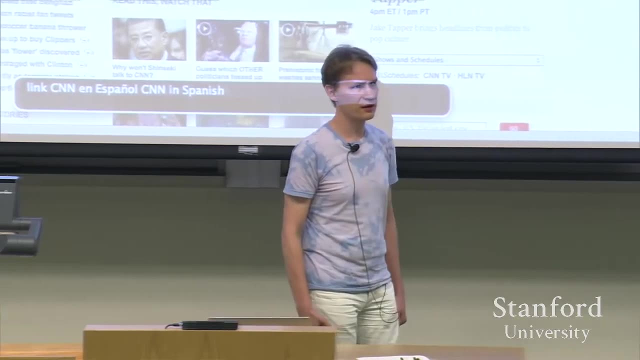 but I have to mention a couple of these things. So we have the language of the web called HTML, And HTML lets us mark up our page in such a way as to make it easier for somebody, like a screen reader user, to dissect the page and avoid all this repetitive tabbing. 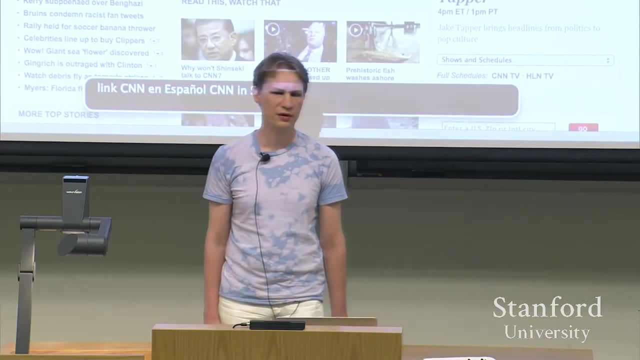 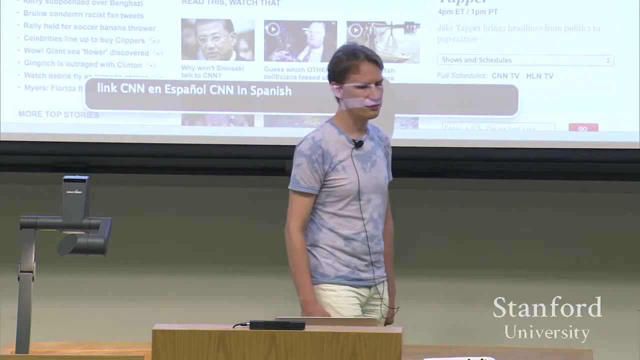 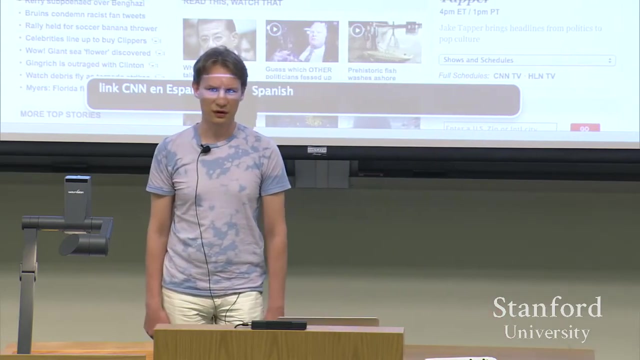 So you do this only when you absolutely have to. But if the page is marked up correctly, you can actually reduce the time that you have to spend tabbing through the page, Because HTML gives us features like HTML headings. We've got form fields. 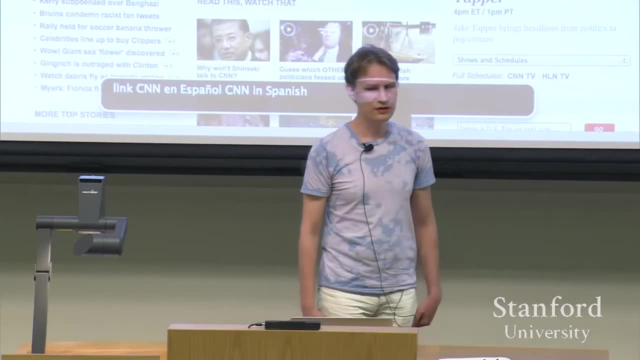 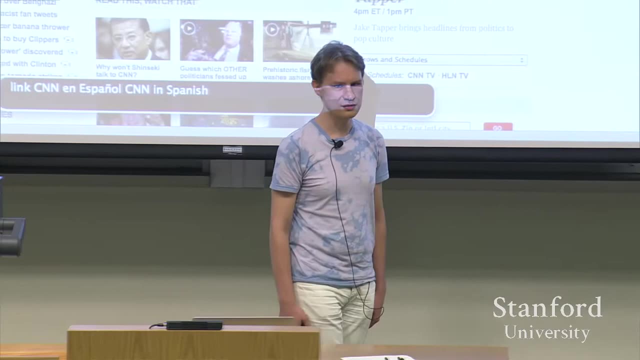 We have lists, And so, if we use all this HTML correctly and provide the necessary semantic information, the screen reader, being software as it is, can take advantage of that stuff. It says: hey, I'm smart, I can figure that out. 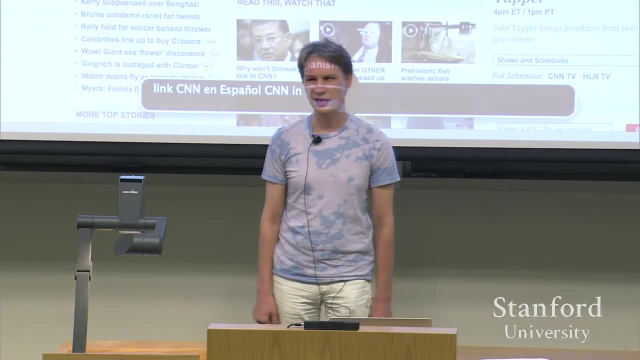 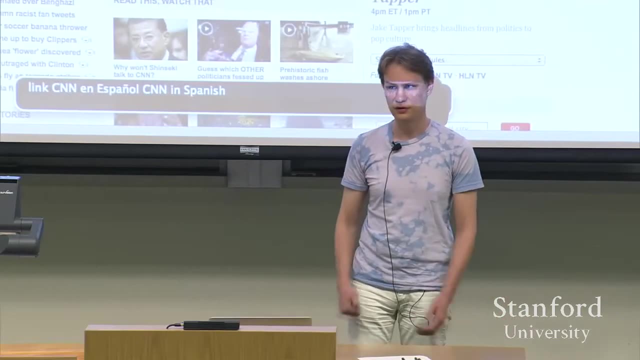 I take a web page, I scan the DOM. I can see the headings, I can see links. Now, if the heading, of course, is only a CSS heading, but it's not an actual H tag, the screen reader, as smart as it is, it, would know that it's actually a heading. 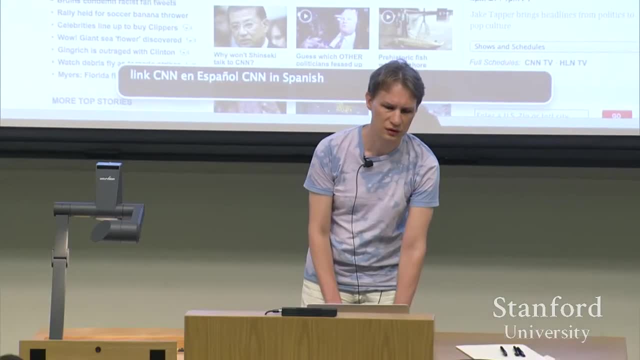 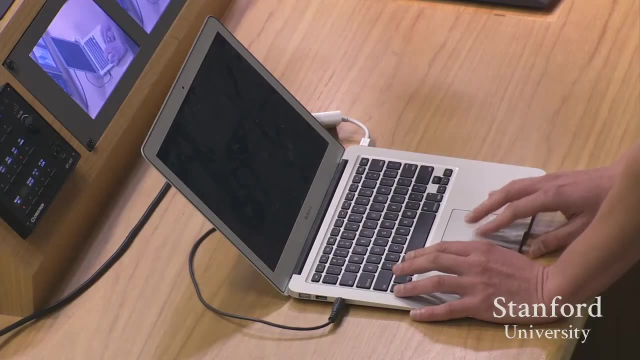 So to show you what I'm talking about, I'm going to turn on the screen. Let's see Where's the thing. Screen curtain on. OK, Here we go. VoiceOver muted- Oops. VoiceOver Link Page. 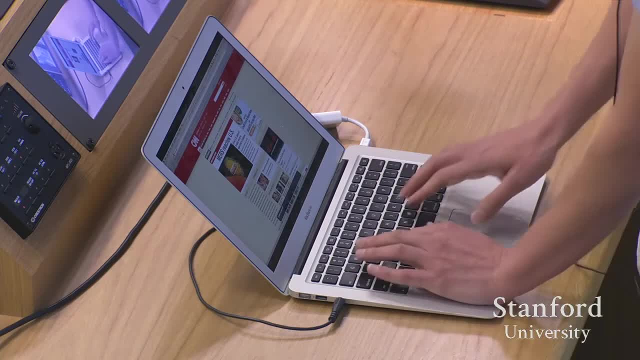 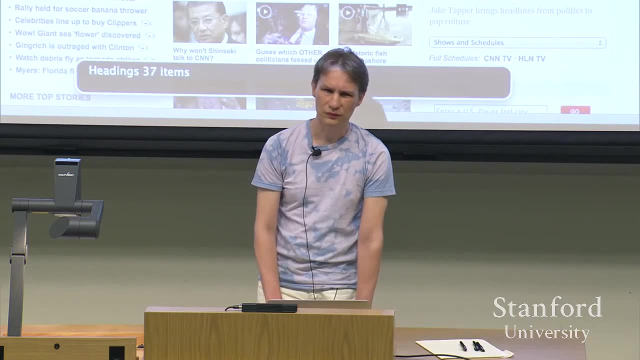 Oh no, Screen curtain off. OK, cool, Here we go. I just wanted to double check. So what I'm going to do, I'm going to show you, like a quick overview of this page. Headings: 37 items. 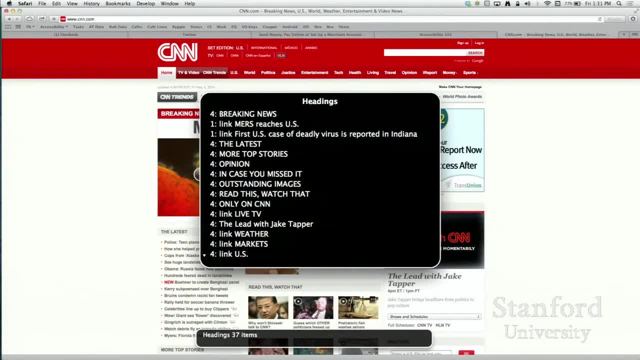 You guys should see that Right. So there's a list of headings And as a screen reader user, I can go through this list and actually decide which of the headings I really care about. For breaking news. one link merge reaches US. one link first: US case of deadly virus. 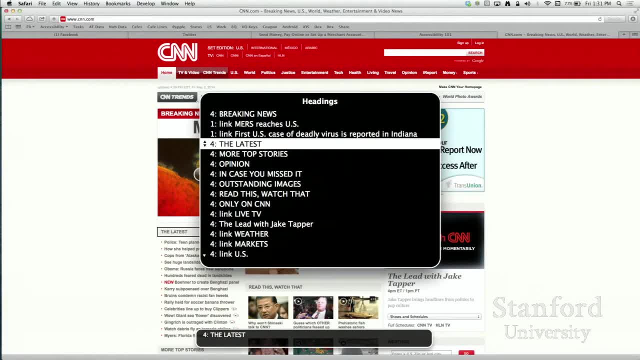 is reported in Indiana for the latest. OK, so you've noticed that also next to that, to each heading, there's a number Right: One, four, three, two and so on and so forth. This page, by the way, is poorly structured, but that's a separate story. 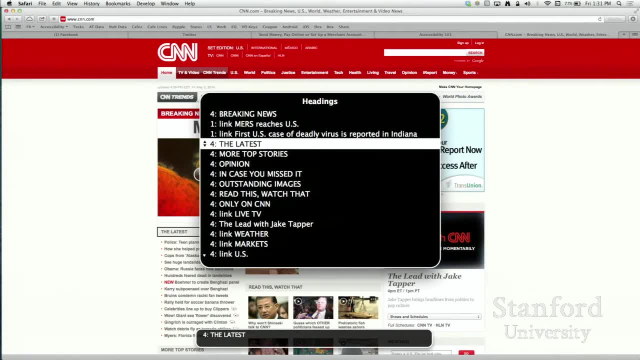 We've got to cut this out from YouTube video Anyway. So these are different levels of headings, Just like in Word document. if you guys create bibliographies or things like that, or when you have chapters and subchapters and sections, it's pretty much the same way. 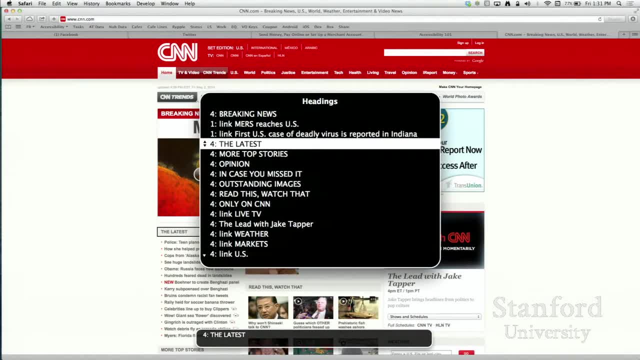 Right, Except in HTML, we use heading levels to indicate that. And yes, there are shortcut keys to let the users, once they know the page, once they learn its structure, there are shortcut keys to say, hey, you know what? 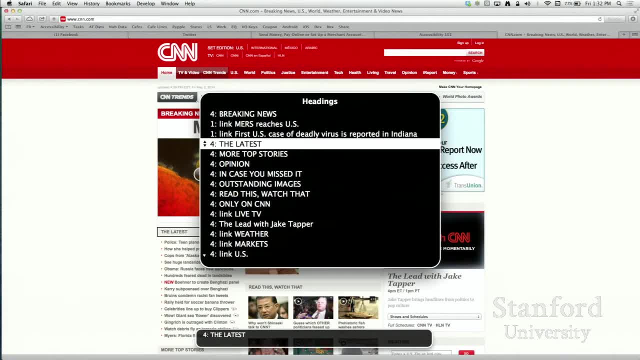 I know that my top stories begin with heading level one, so I just want to jump between those. I don't care about other headings. OK, So all of these things are available, So I just pick one of these headings. Let's say, for breaking news, one link merge reaches US press. enter heading level one. 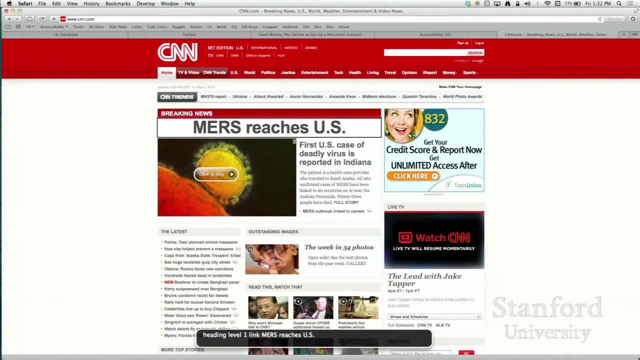 link merge reaches US And the focus jumps to, to that particular place on the page. You are currently on a heading level one inside of HTML, So you can see just immediately how, by using headings, I already cut down a number of keystrokes. 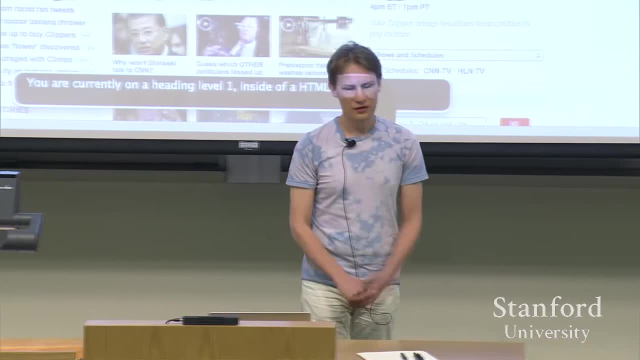 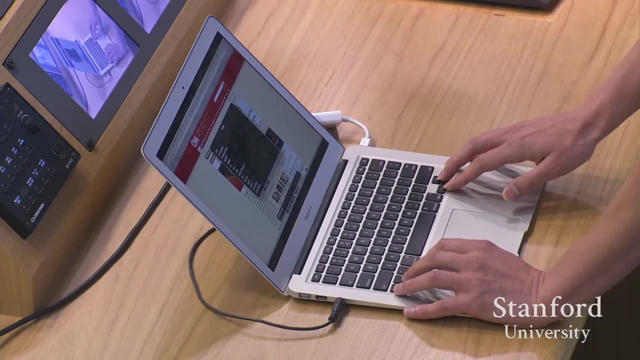 that I have to press just to get to the middle of the page. So you know, essentially there you can see there are other things like headings, links. three hundred ninety one items. Wow, See how many times you'd have to tab Three hundred ninety one. 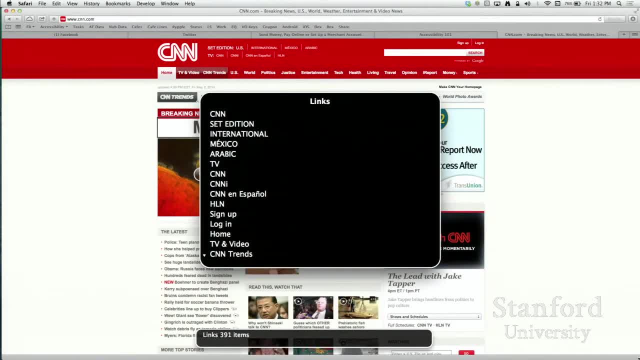 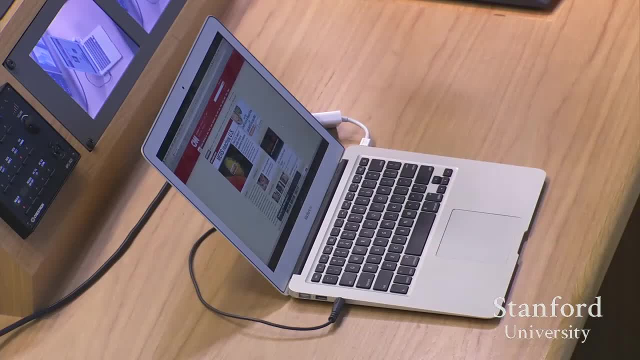 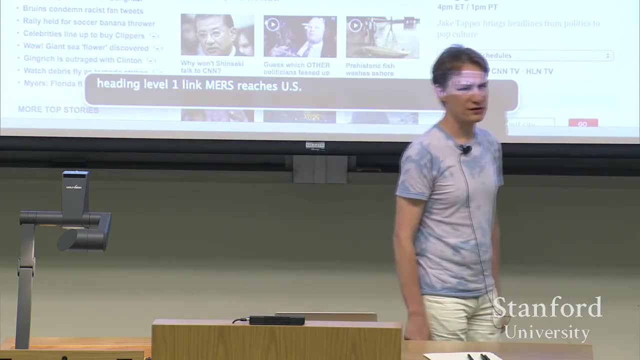 And that's at best. So there are also other shortcut keys to get you to, because obviously not everything on the web page is focusable. There are some elements on the web page that are: either. there are pieces of text, you know, like subtitle of the story. 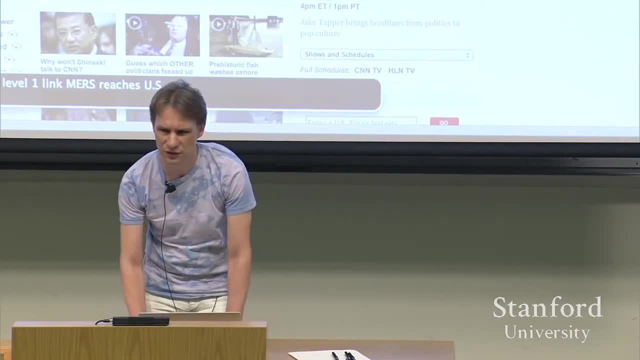 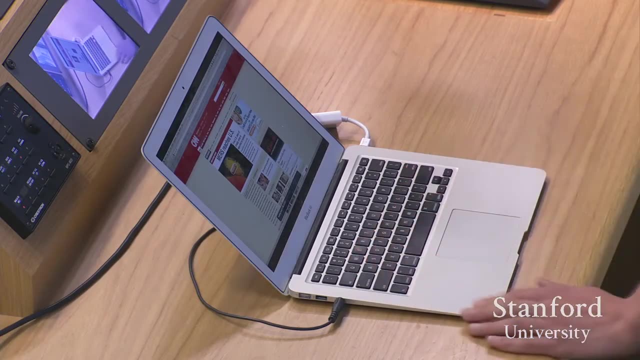 So there are shortcut keys to let you go through that. So I have. I can simply move through the DOM in this link. OK, So let us quickly. So this is, in principle, how screen reader works. I'm going to see Check out Jeff's. 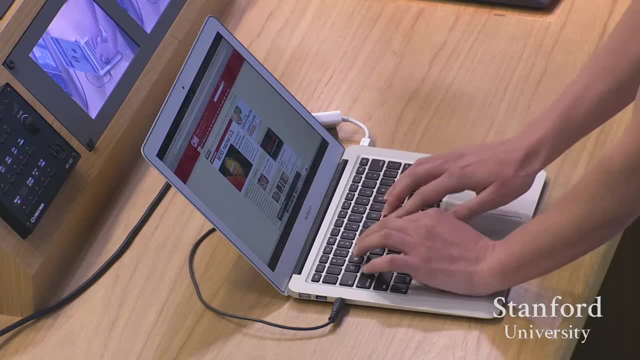 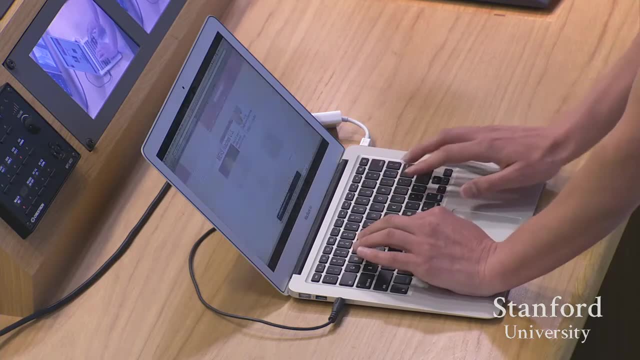 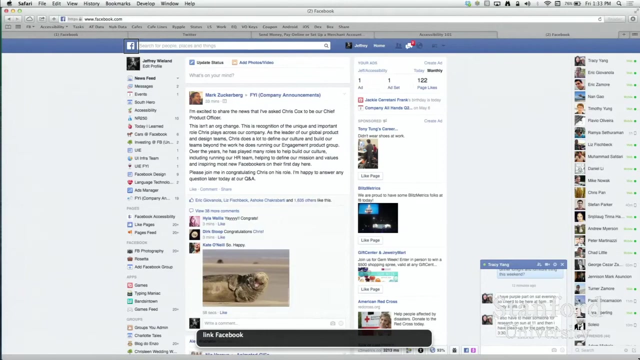 Should I use Safari or Chrome Open look, Oh, Here, See on selection: See Period M. unhighlighted insertion to Heading link Facebook. So, without going to Facebook, many of you guys are using Facebook. I hear that they are currently on a heading level one inside of HTML content. 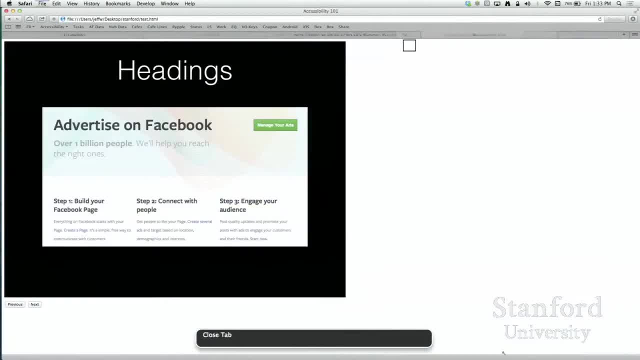 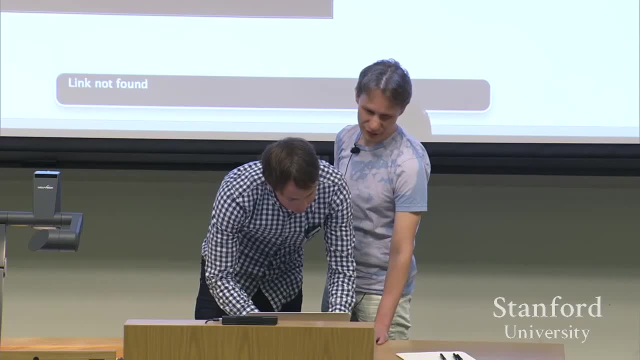 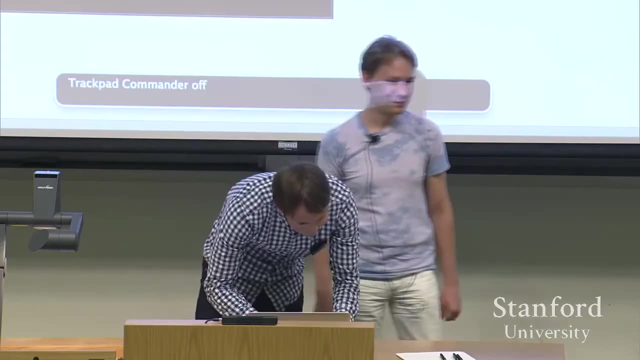 Oh, So actually? Oh, Enter To mess, Click No. Link not found. Next button: Previous button: Heading link not found. Wait, You got it. Trackpad commander. OK, One Facebook Link: Facebook. 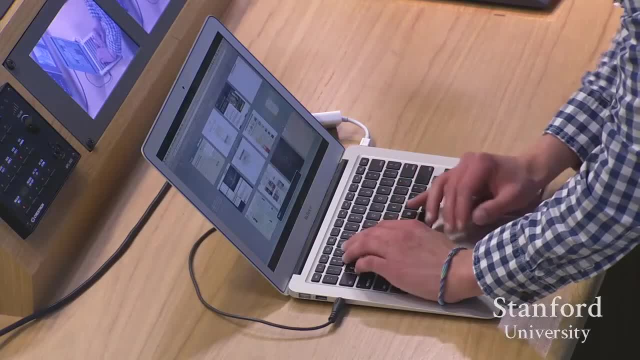 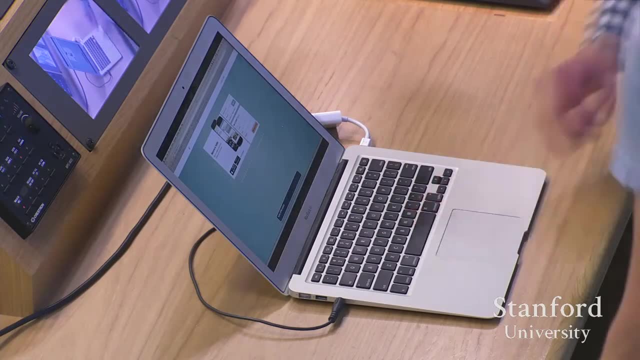 Close tab. Twitter- New tab. I asked you. You said it's OK. Accessibility: Twitter: Twitter: HTML content. OK, Cool, All right, But teenagers are Currently on HTML content To enter the Facebook Or something. 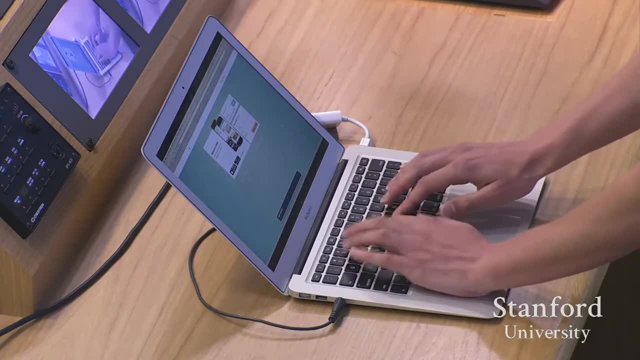 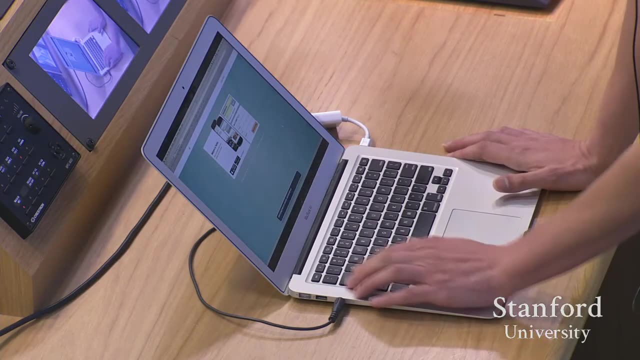 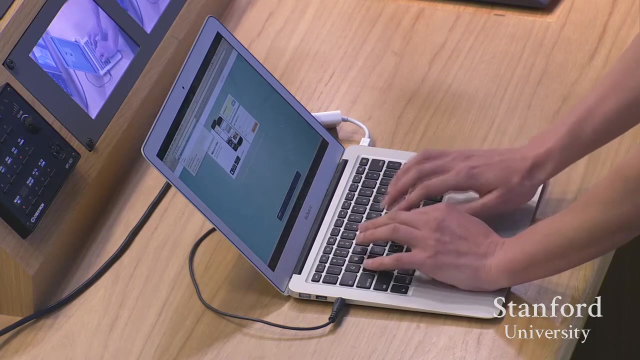 Yeah, Yeah, We can use something else. Open location. Oh, Sorry about that, Jeff, I didn't mean to. I asked you Password, Secure Sign in, But Open W P O M Slash. 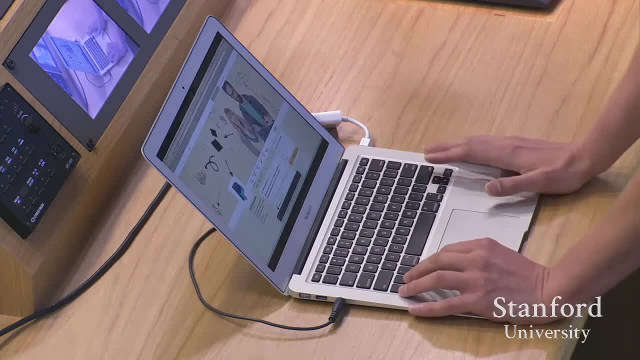 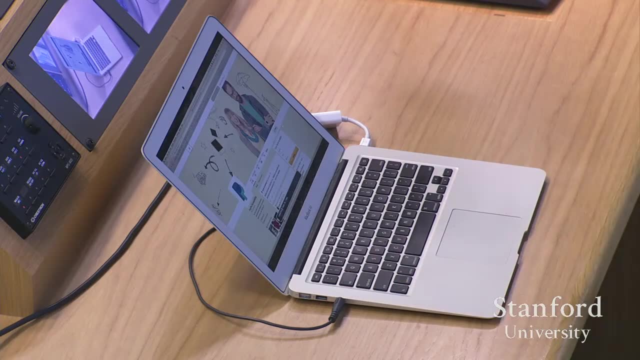 Com Slash A A L All right Heading level two Visited link Twitter List. So So When we move into the world of web apps, Obviously Not everything is going to be as simple as just like moving from link to link. 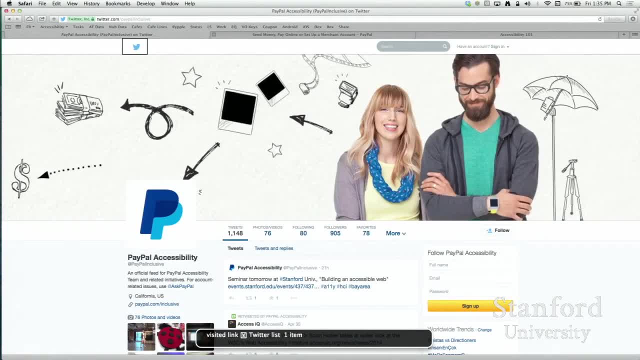 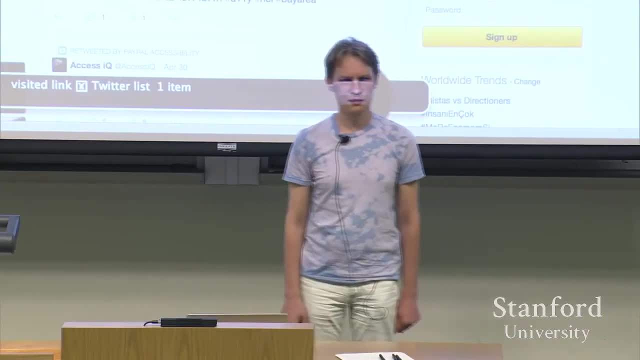 Or You know, Moving between headings, And so Twitter And Facebook And Gmail And Some other leading Providers Have done some amazing job In Sort of Exploring How can we take the web feather. 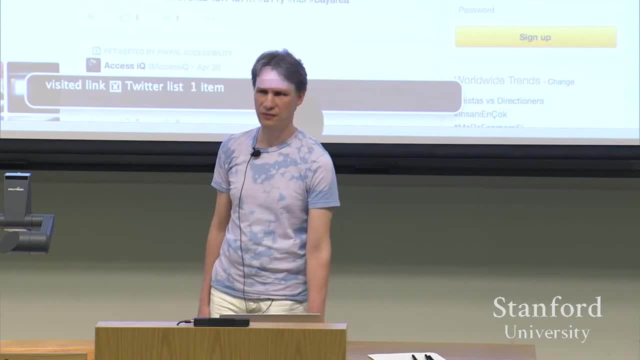 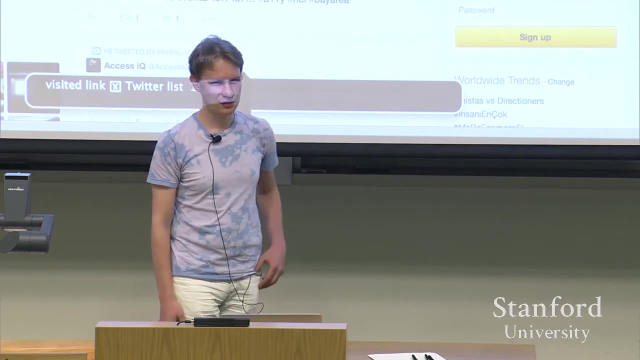 And You know, For example, Take the web feather When we have to deal with Web apps. So, For example, In Twitter's case, And Facebook is the same. But since You know, Jeff, We couldn't get it working. 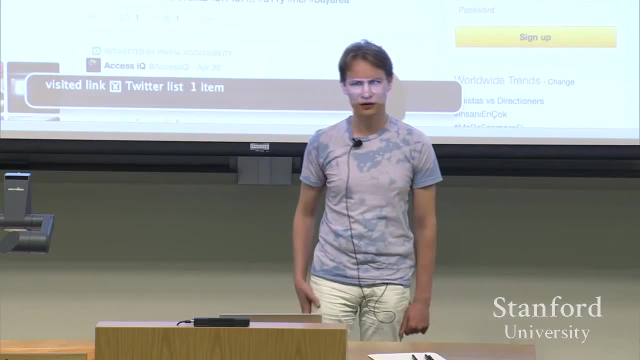 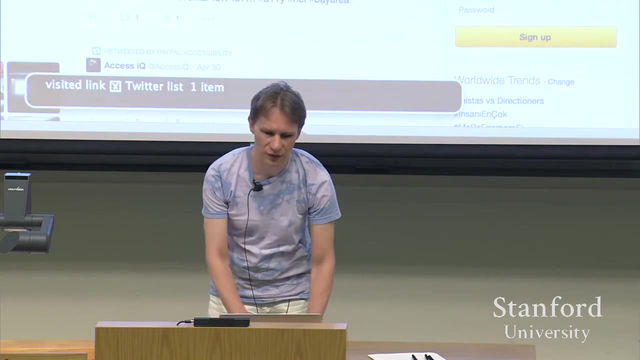 So They're kind of like in parallel. They provide a lot of shortcut keys To let the users Feel like they're using the actual app And Not just Website. So, For example, In Twitter's case, I can use. 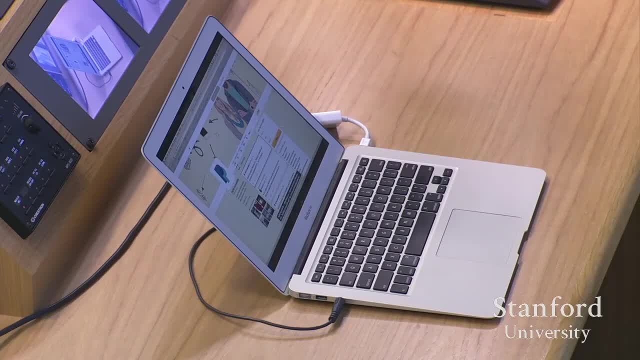 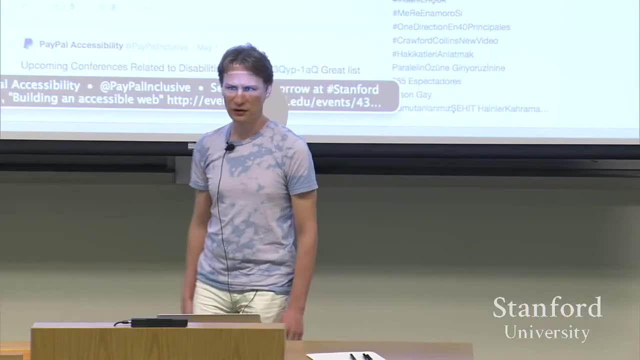 Actually Let's Well. Yeah, I can use The same thing on Facebook. You use J and K To move between Posts, Which is really Really cool, And you notice The screen reader Will actually announce All of this magic. 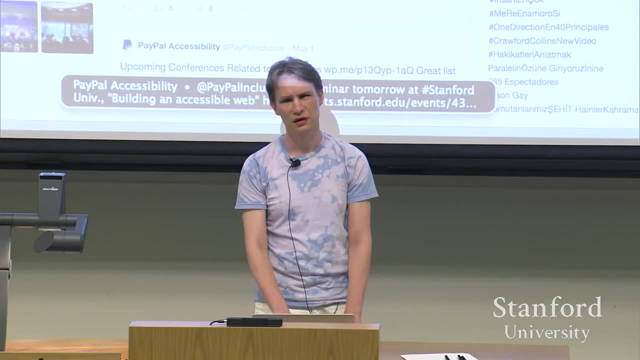 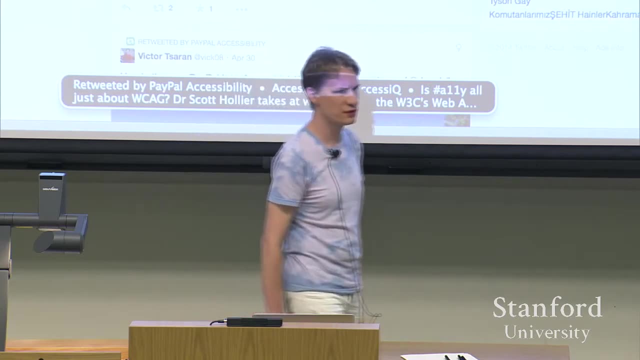 Of course, Is done with the help of focus, Right. So Every time the J key moves The Retweeted by PayPal accessibility, So The focus Is being moved To that object Right. So In this, In this case, 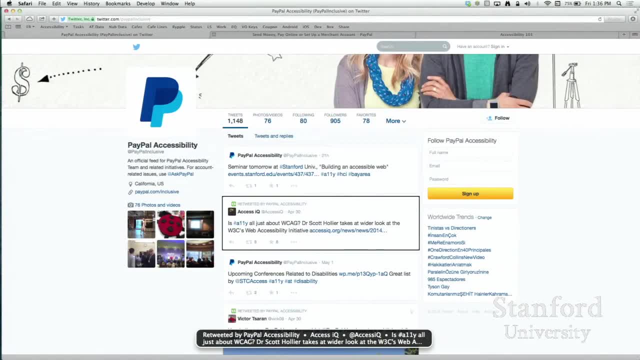 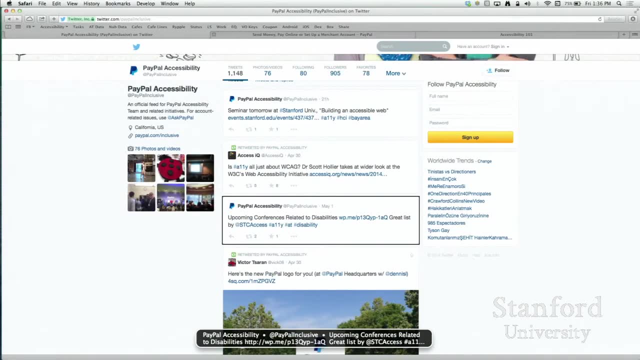 It's going to be a tweet, And, And You know It's going to be Yeah, Okay, Wow, Not too few voices. Yeah, PayPal accessibility: That's okay, Because I don't use it myself. So 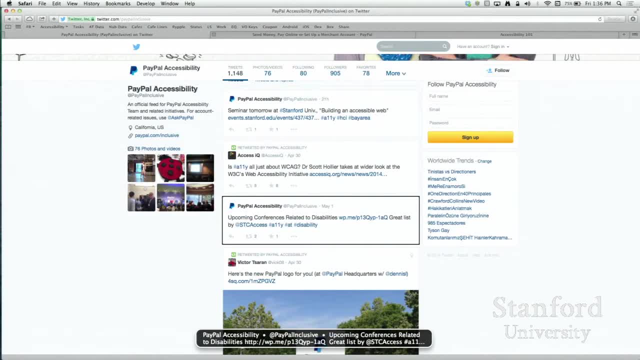 Yeah, I have other editors I like So, But anyway, So It's, It's a pretty unique Thing To do, You know, J and K, And But this is okay Because this is like You know. 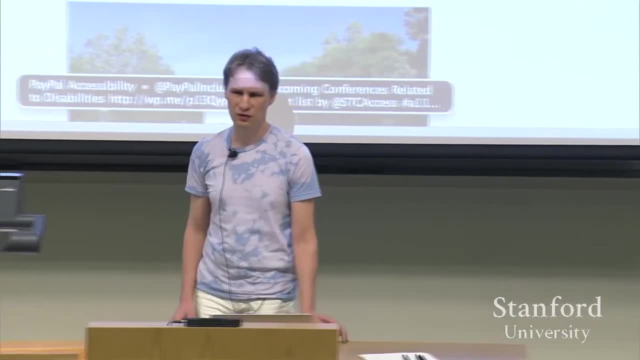 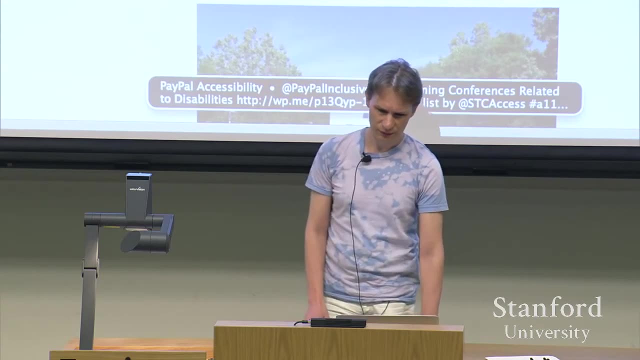 On YouTube. The same thing You can use, You know. The same thing In the case Of, You know, Not just being like A regular, Just looking At the regular Website, But also Working with More complex 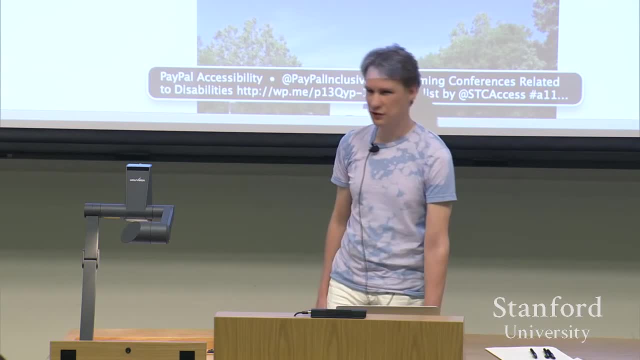 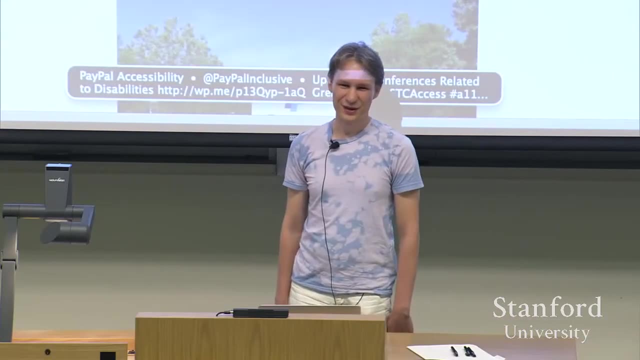 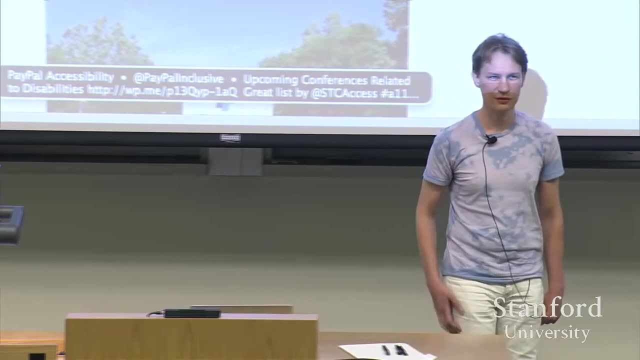 Applications. So If I wanted to know What shortcut Keys are available On Twitter Or On Facebook? Anybody Wants To get The shortcut Key. Sorry, The shortcut Key Is a public And private. 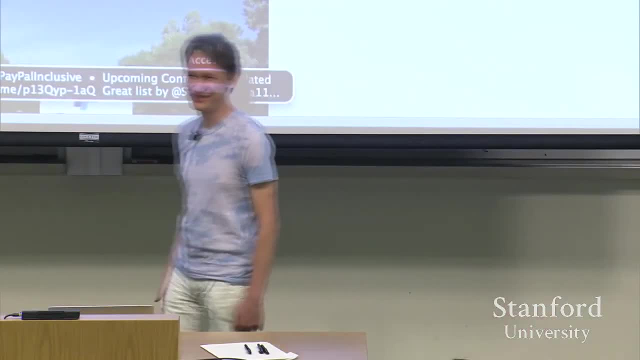 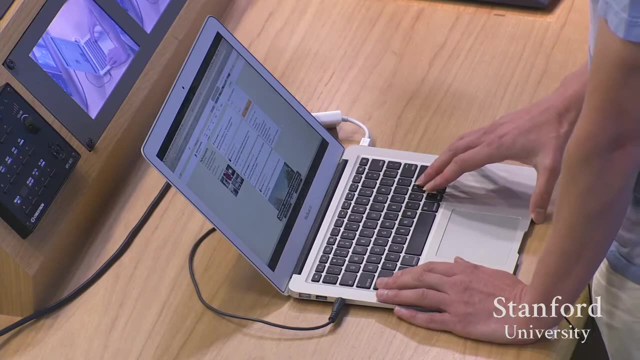 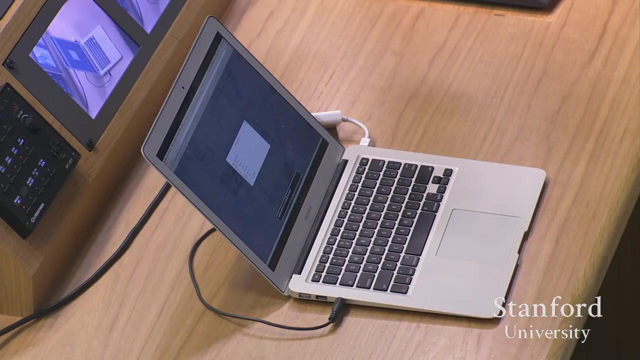 Key. Without those Keys You can't get To the rest. So There's Always One Key You gotta Know, Right? Good, Guess Anybody Else Question Mark? Okay, Let's. 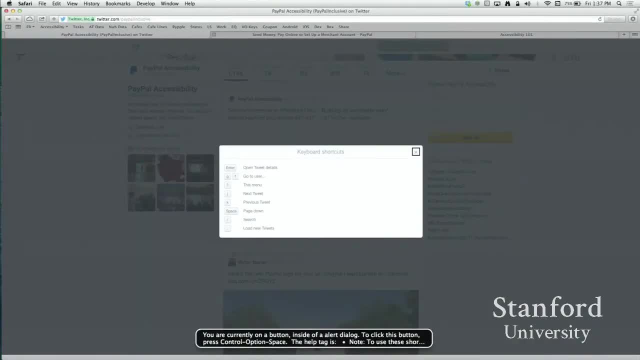 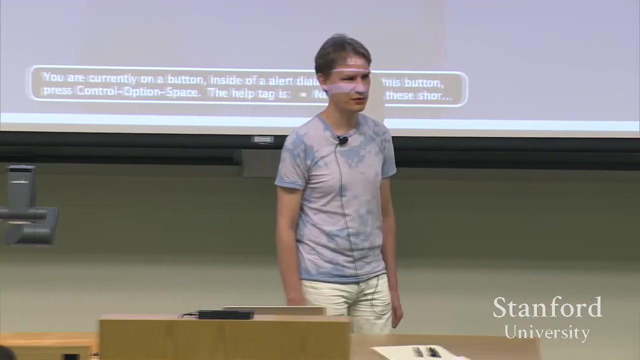 Do Keyboard Shortcuts, Alert, Dialogue Close, Which Is Really Important? This Is Going A Little Bit More Into Beyond. I Think Basic Stuff, But Essentially 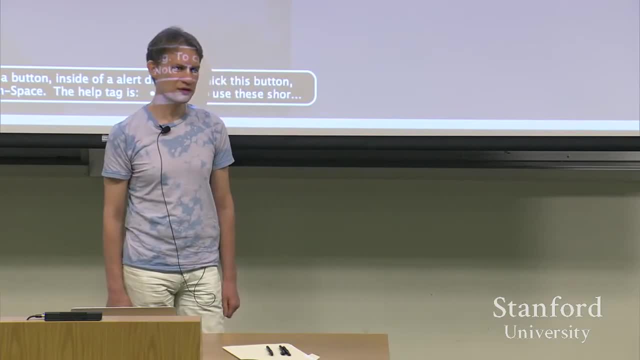 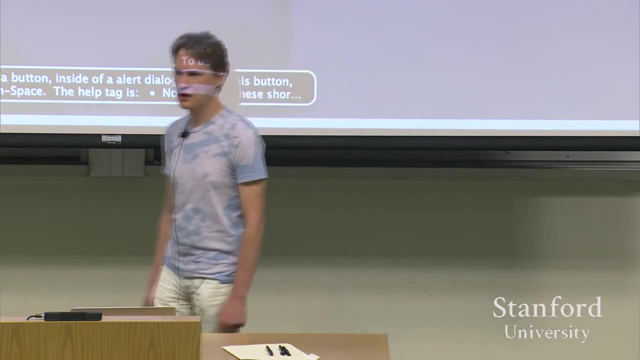 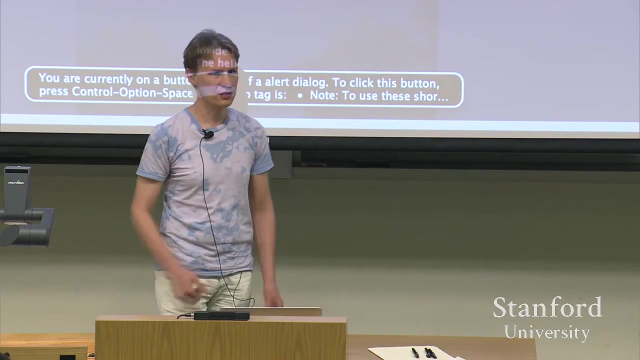 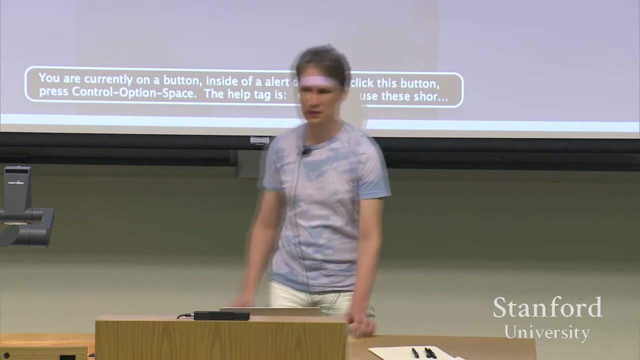 One Of The Big Problems On The Web Is That You Use A Screen Reader, Because For Screen Reader, Diff Doesn't Mean Anything, So There. 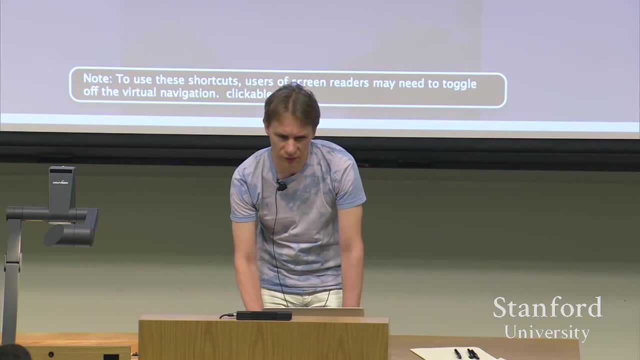 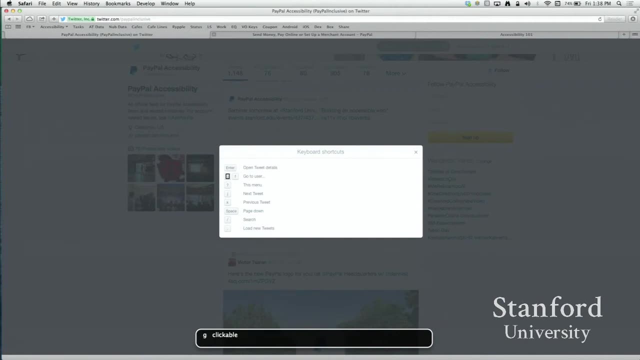 Are Certain Super Semantics We Can Lay Over In The Code To Communicate That F, F And So On, So Forth. You Go And 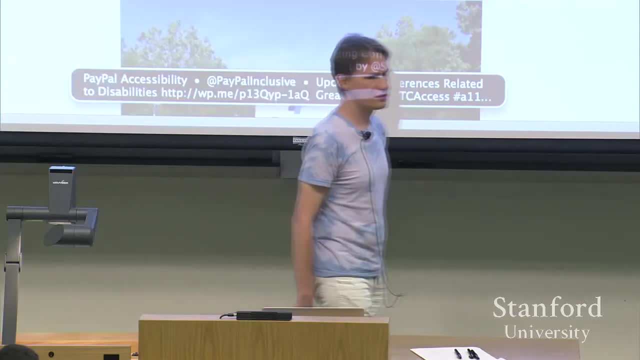 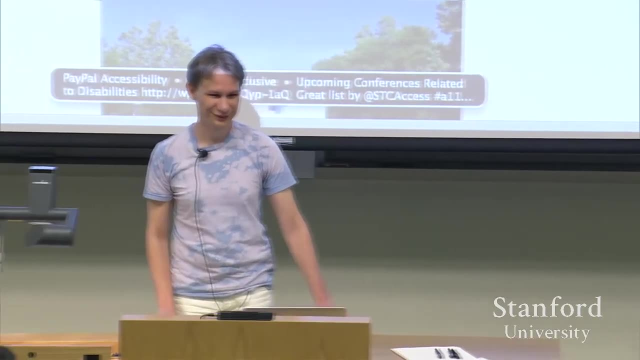 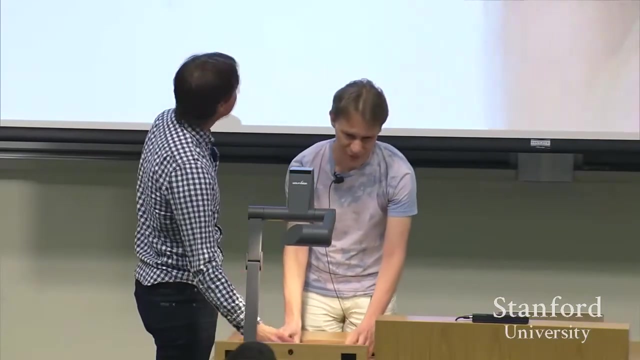 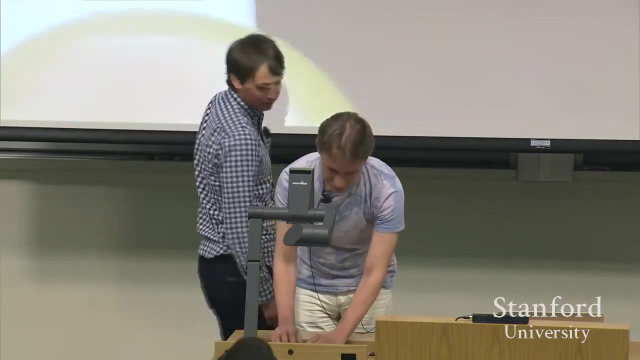 You Study All The Shortcut Keys, But Yeah, This Is All You Need To Know, Even On Facebook. Just Let's Hope Nobody's Going To Send. 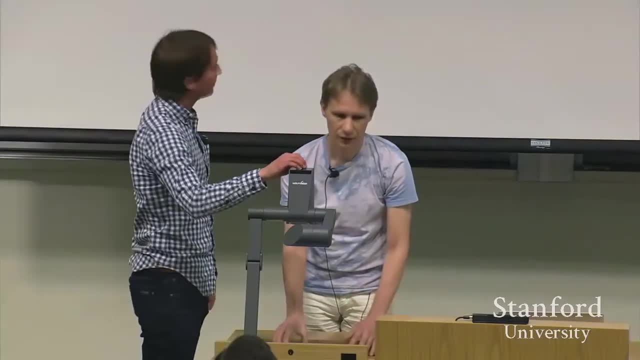 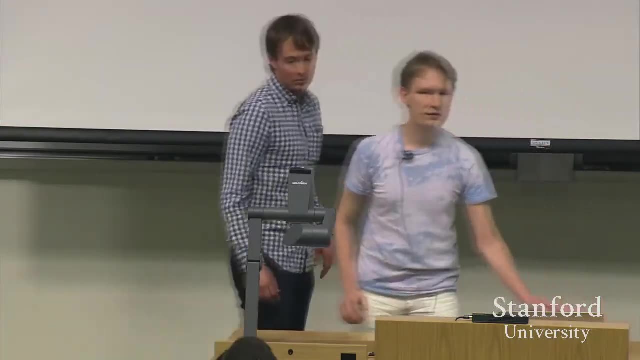 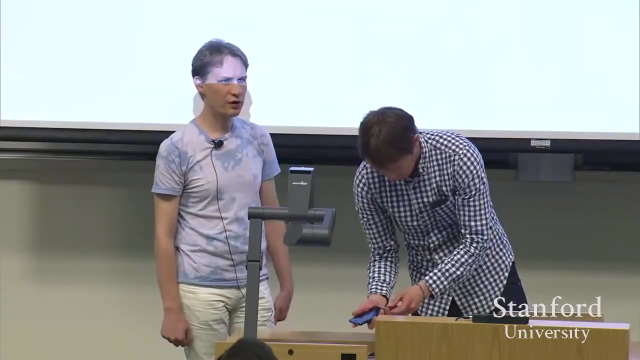 Many Messages. Okay, Okay, Can You Give Me What Do You Keep? Yeah, Oh, It's From Here. Yeah, So So In 2009.. We Already 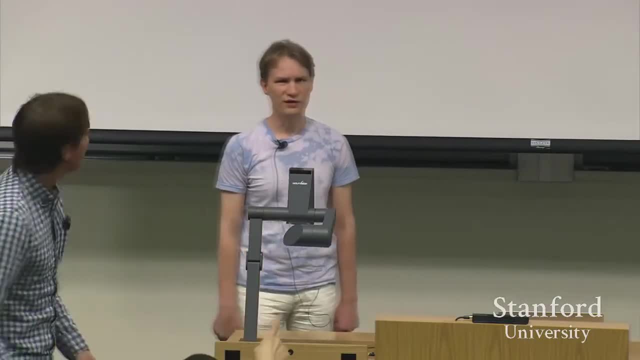 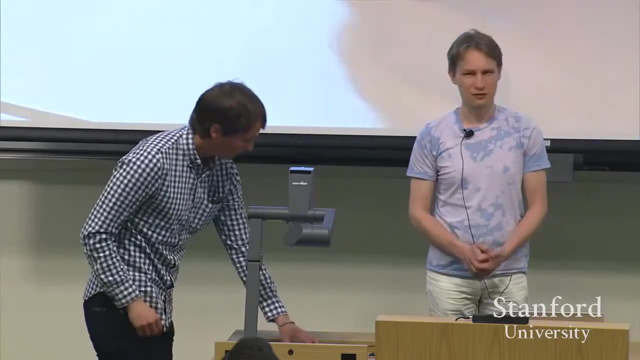 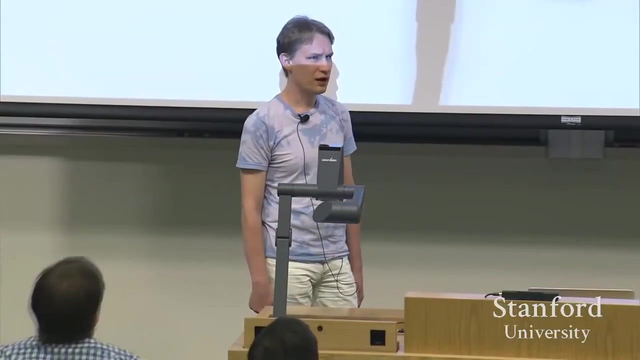 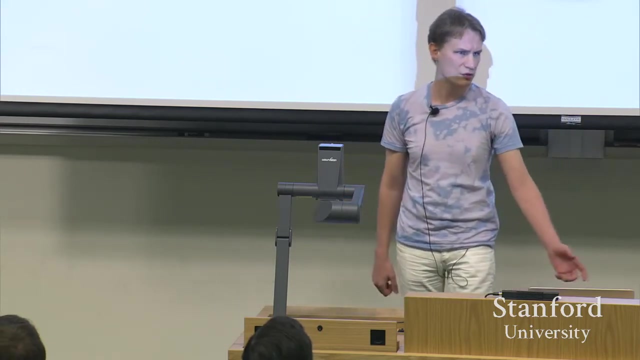 Have This Key And You Can Use This Key Because You Can Feel Each And Every Key, Or Even In The Case Of Nokia, You Can 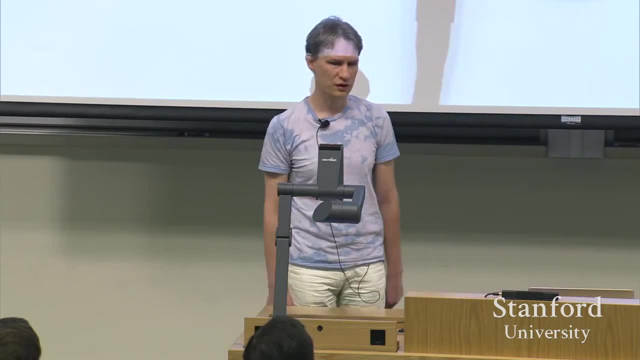 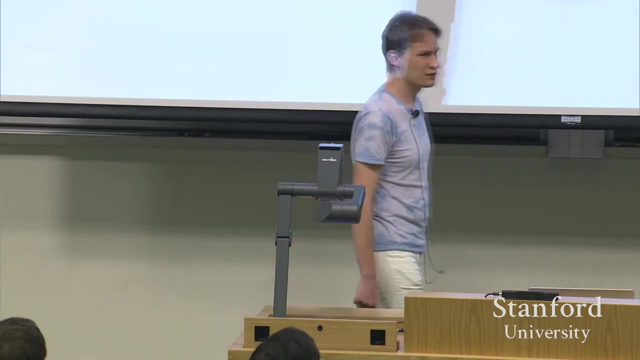 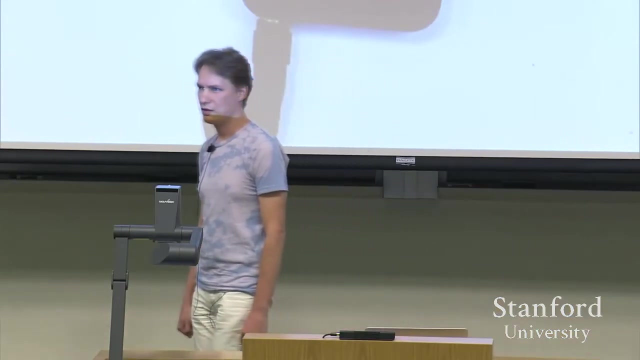 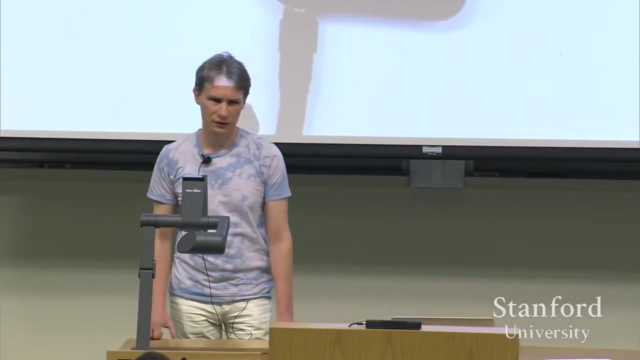 Use Buttons Or A Smart Shirt And They Put It In The iPhone. Okay, That's Great, We Got There, First Step. What Is The Biggest? 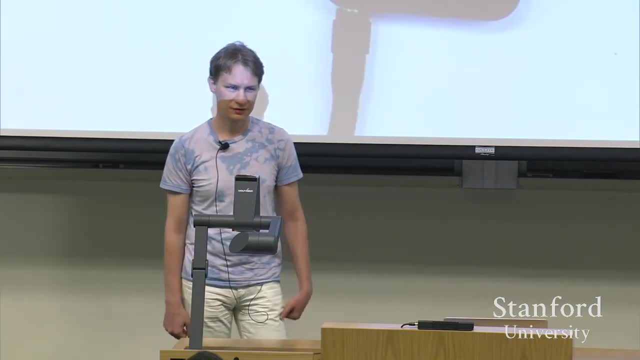 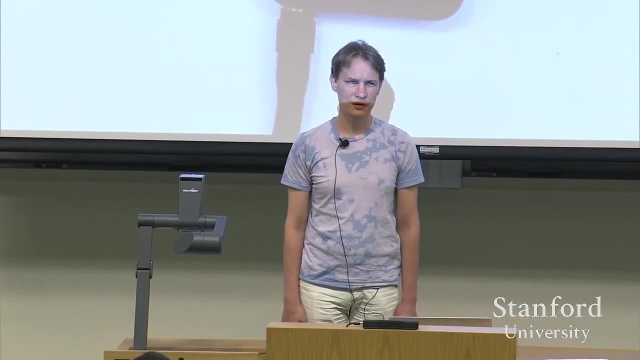 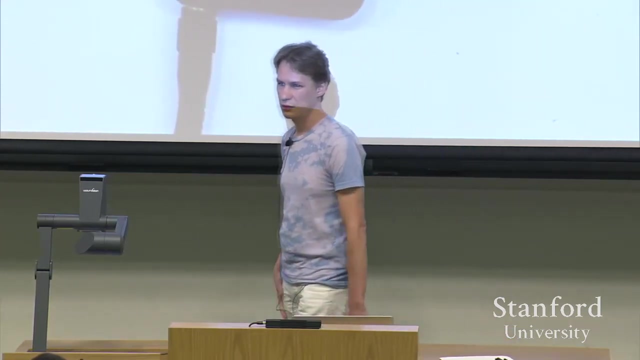 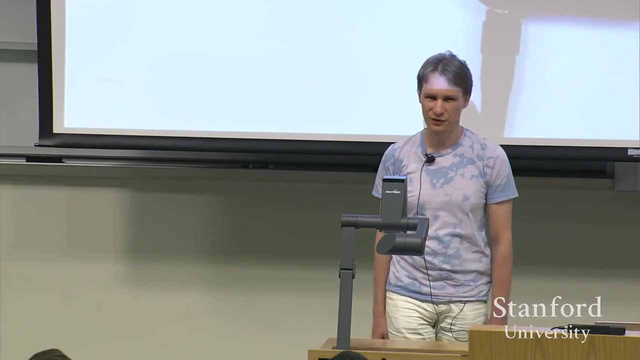 Problem. You Guys Are Smart People Here, So We Assume That What's The What's The Big Thing? It Has To Something With The Way You. 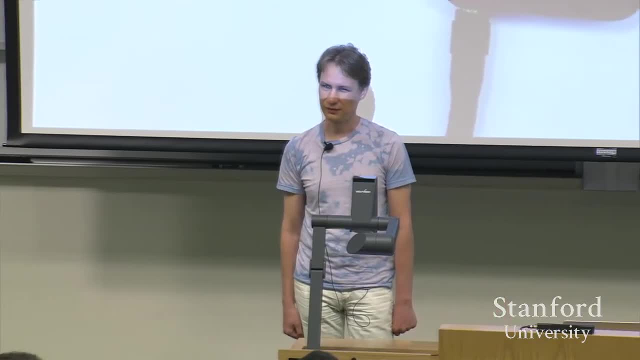 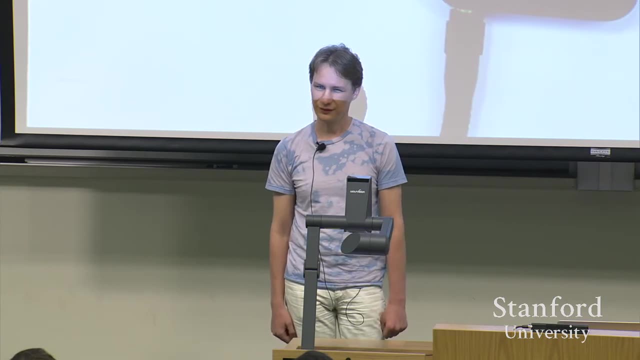 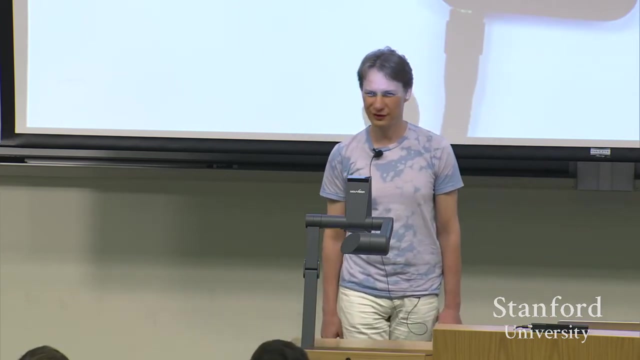 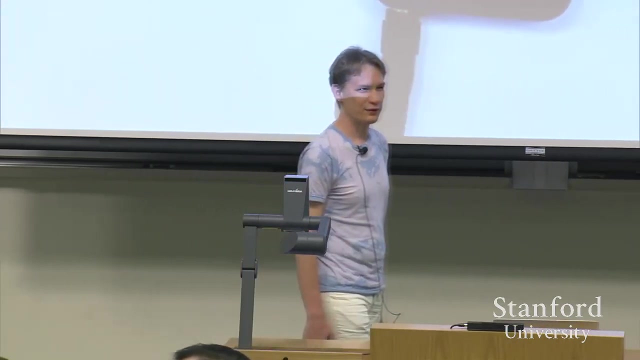 Gesture With The Touch Screen. Where Do You Press Okay, Right, What It Actually Is. It Will Actually Simply Execute That, Just Instead Of Telling. 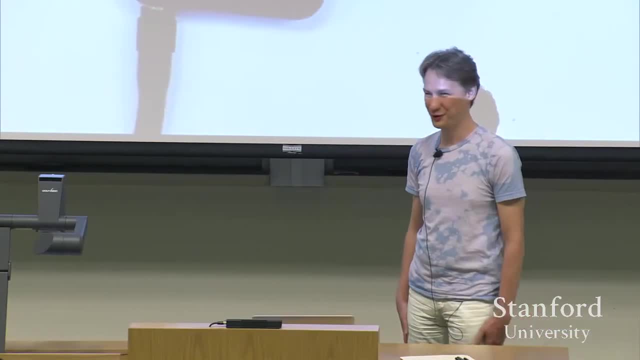 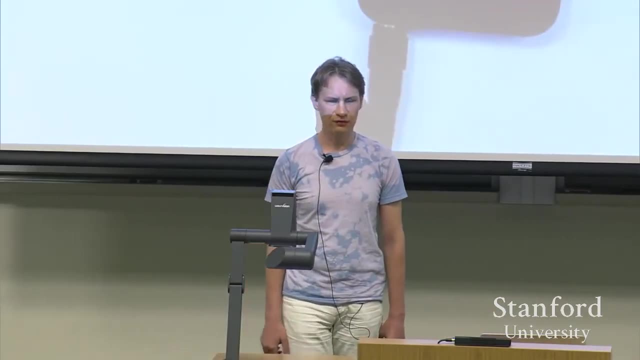 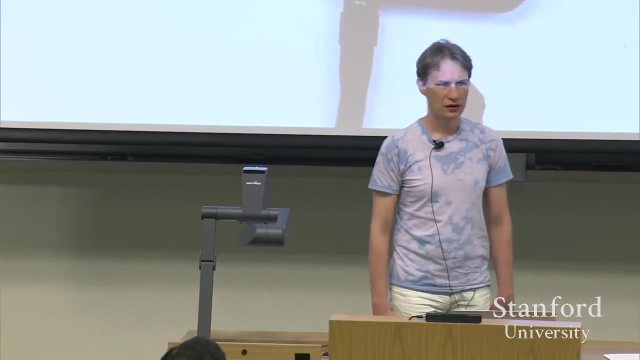 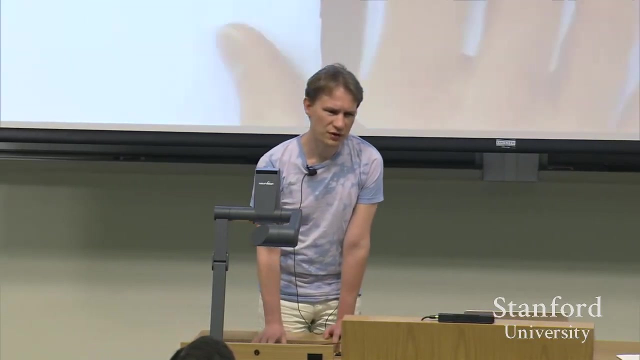 You. What Actually Is There? Did You Guess That? Or You Know That Kind Of You? Who Is That Is? You Know That Is, You Can. 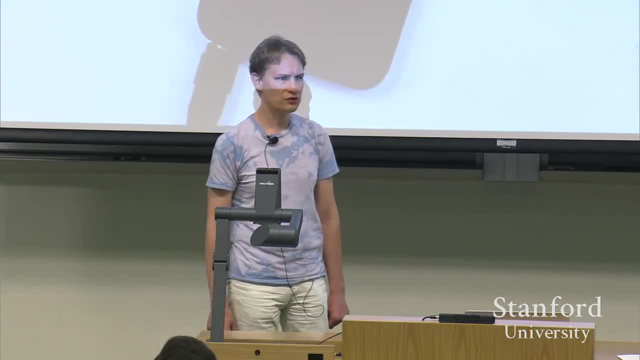 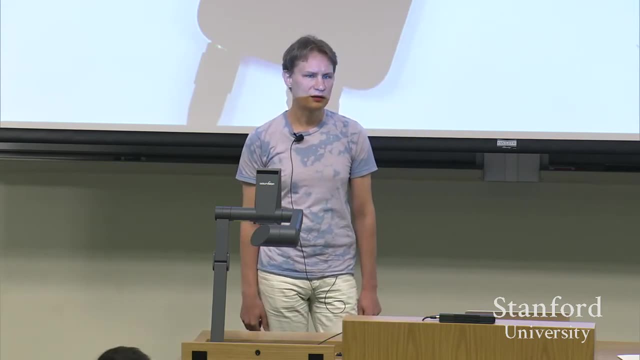 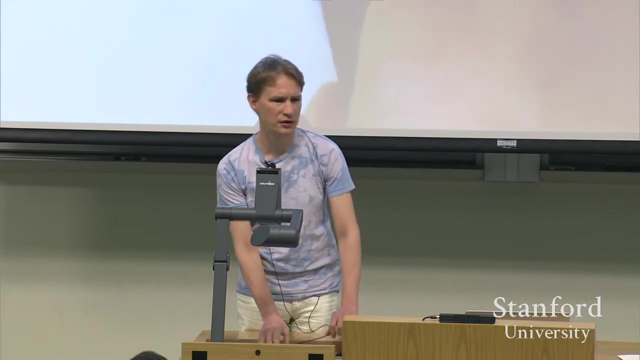 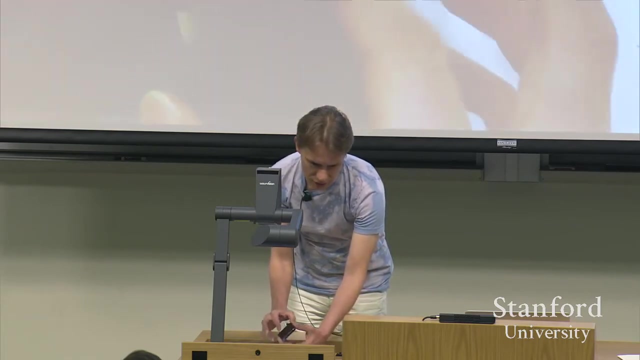 Be. You See, That Is A Thing, Is That Is Something You Can Do, That With You, A twice to execute it. So now I'm going to make it louder, sorry, Okay, is this? Oh wait. 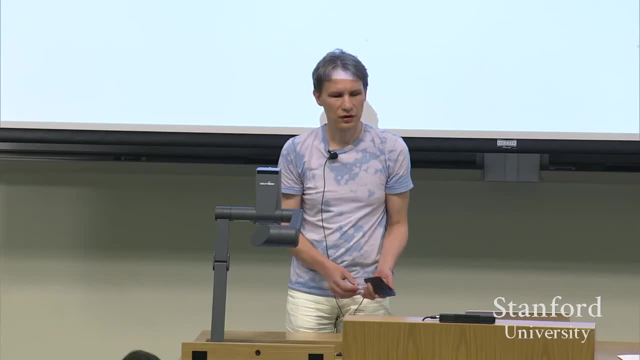 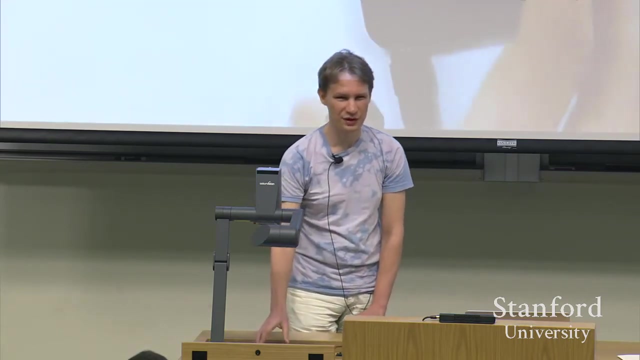 you know what? Give me a second. I forgot I need to. oh, these corporate phones. Actually you'd be surprised, not really, You know why? Because I think the speech takes quite a lot of battery too, because it constantly keeps on talking. That would be great actually. 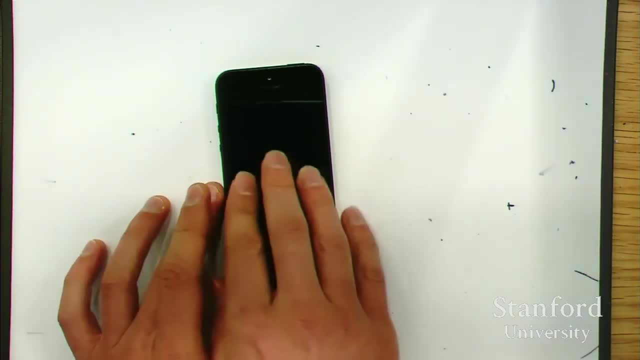 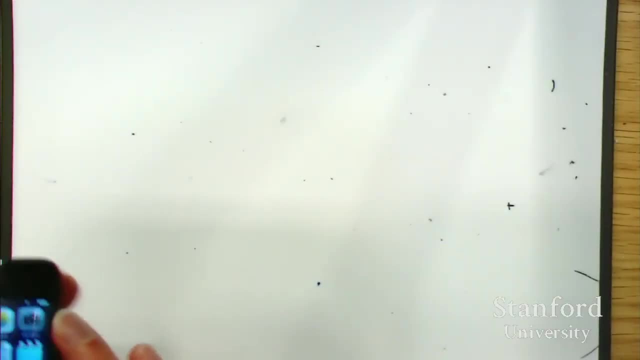 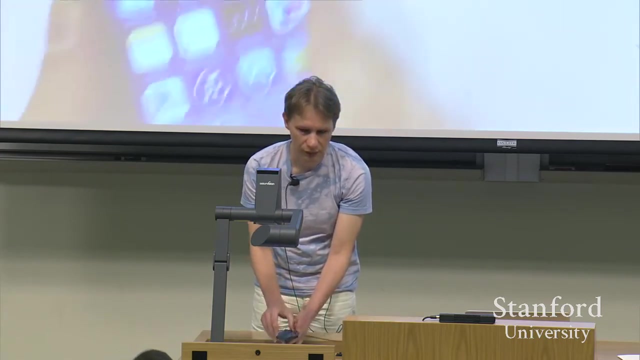 Reminders: Double tap to open Screen curtain off. Okay, let me just Characters, Language Headings, Containers, Hints, Sounds, Volume, Speech rate: 80%, 50%, 45%, 40%. Okay, cool. 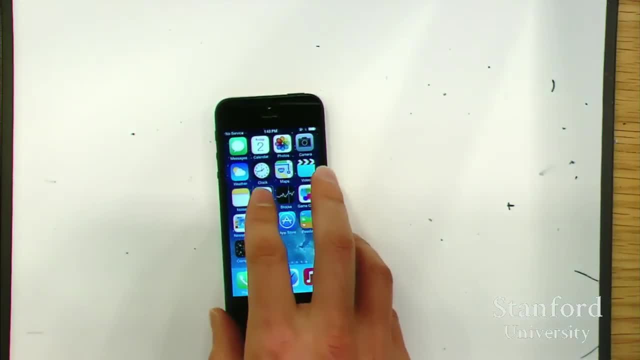 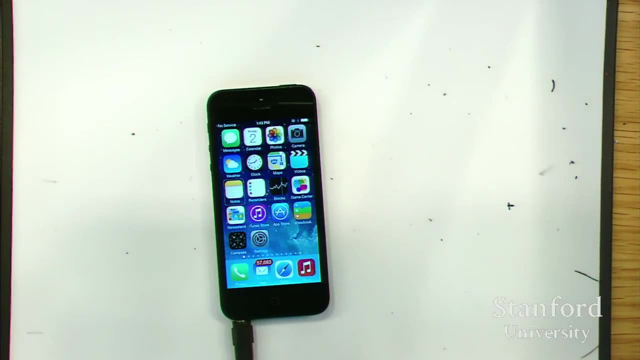 Okay, now, hopefully you guys can see. So I single touch something: Reminders, Double tap to open, Notes, Double tap to open, And then it gives me a hint to double tap to open. So if I wanted to see, I don't know, let's say reminders, App store. Actually, let's do app store Double. 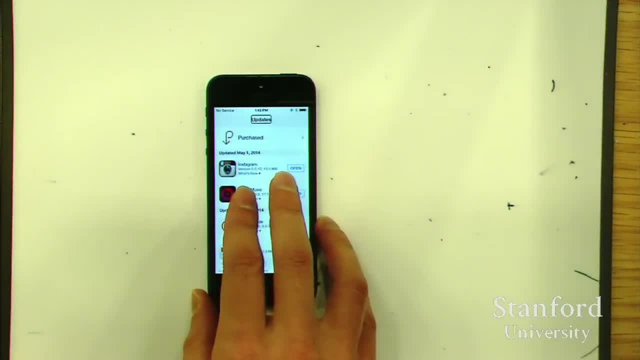 tap to open App store Updates Heading. You double tap right. From here on, you have two ways of exploring the touchscreen. Now, remember, VoiceOver controls my gestures, So there is a way to ask VoiceOver to bypass a gesture means: don't you know? let me. 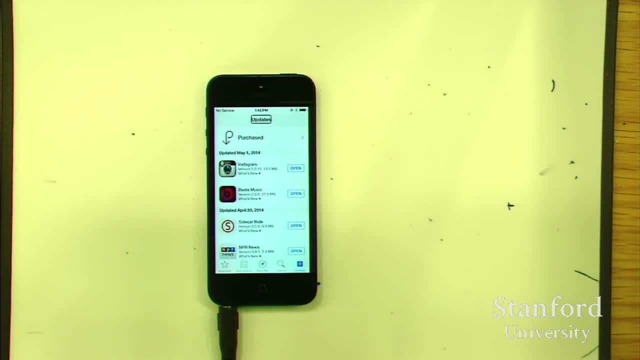 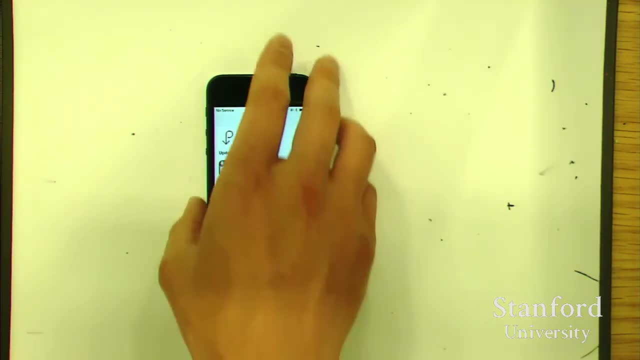 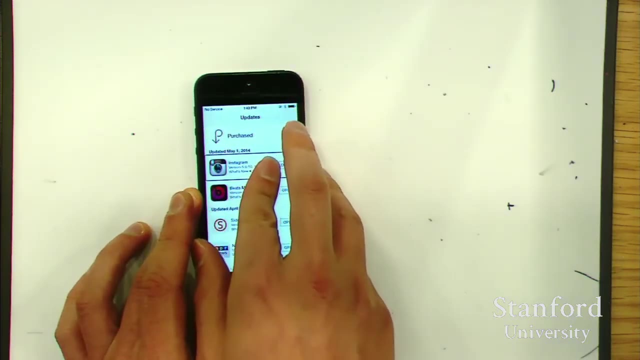 the next gesture, pass it through directly to the app, But by default most users wouldn't want to do that because it's pretty dangerous unless you know what you're doing. So I can just start exploring the screen. Updates Heading: Purchased Updates: Instagram Version Beats: Music Version 2. Up Side. 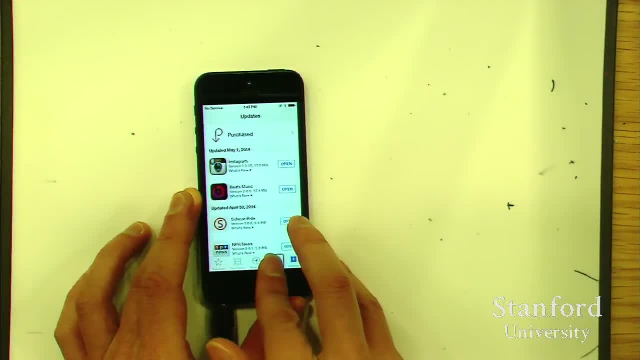 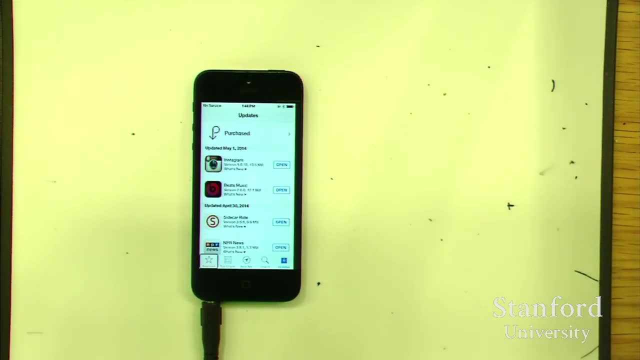 core End- Featured Tab 1 of 5.. Near me Search- Selected Update Search. Near me Top chart: Featured Tab 1 of 5.. Okay, you notice right away what happens there. right Is that I can suddenly start getting. 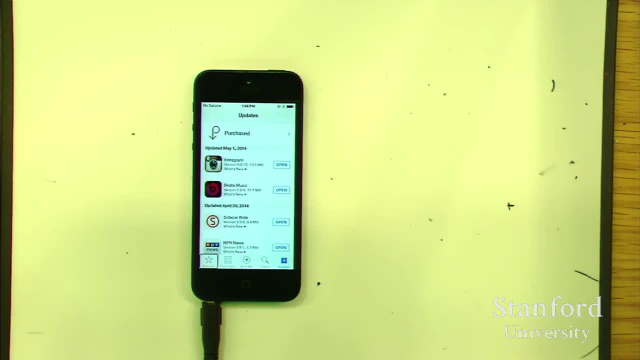 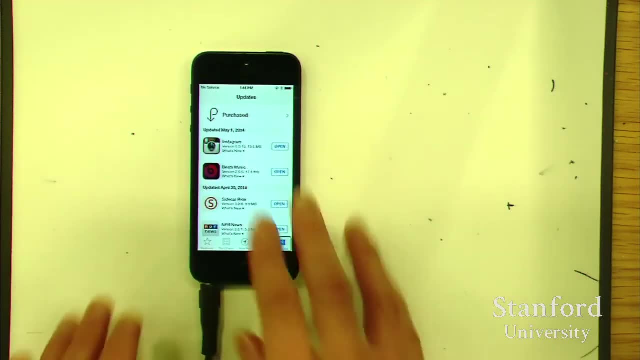 a spatial imagination of the layout of the screen right. So I've got a tab bar at the bottom which consists of five tabs: Selected Updates Tab. Not only that, notice how VoiceOver tells me which of them is currently active, right When it says selected NPR News Version. 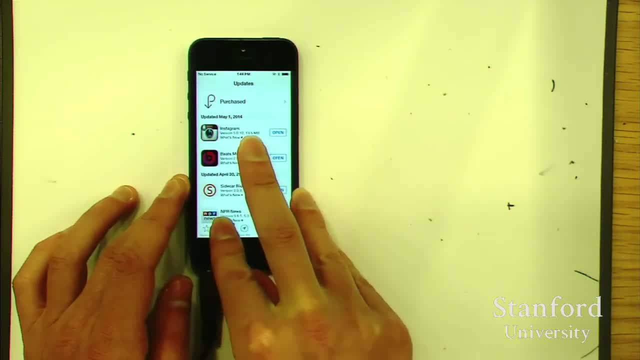 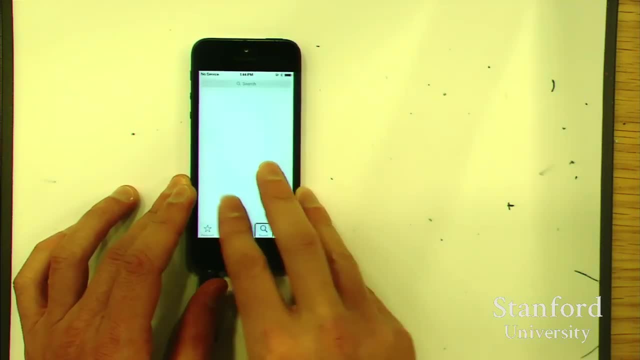 3. Featured- Tab 1 of 5.. Top charts- Tab 2 of 5.. Near me- Tab 3 of 5.. So if I tap one of those, let's say search, Selected Search Tab, Now search becomes a selected tab. So 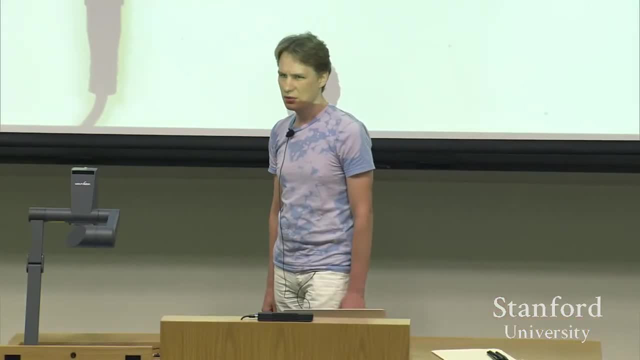 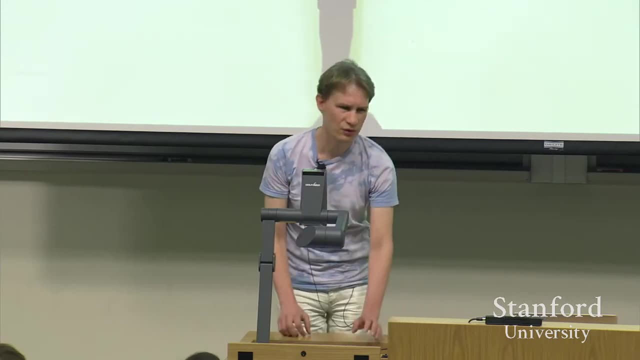 now I talked about one-dimensional navigation on the desktop. Well, finally, with tablets and touchscreens, with the screen reader, we can actually start getting a little bit more into. so I can start if I go to a website and I learn that something is on the left. 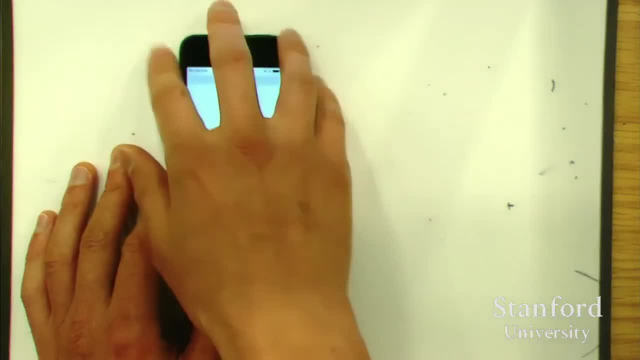 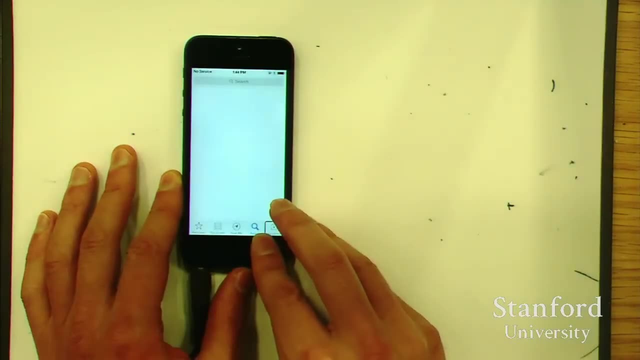 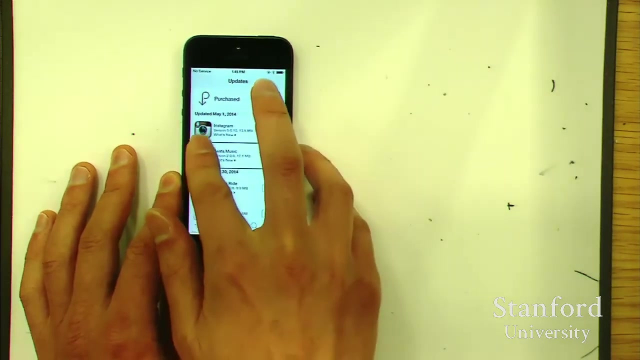 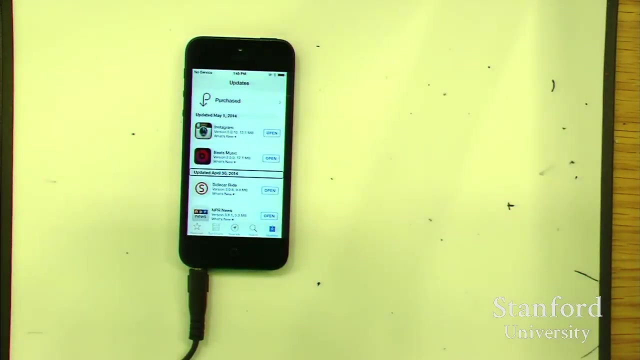 side. I don't have to go, like you know, one by one, I can just scroll my finger. Top charts: Tab Selected: Search Update. Tab Selected: Update Beats News, Instagram, Right, So that's one way So you can drag your finger, learn you know. layout of the. 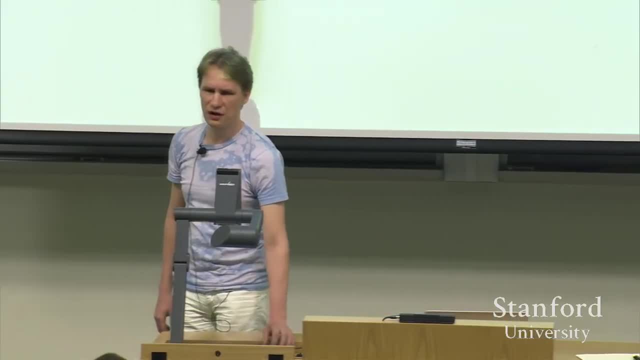 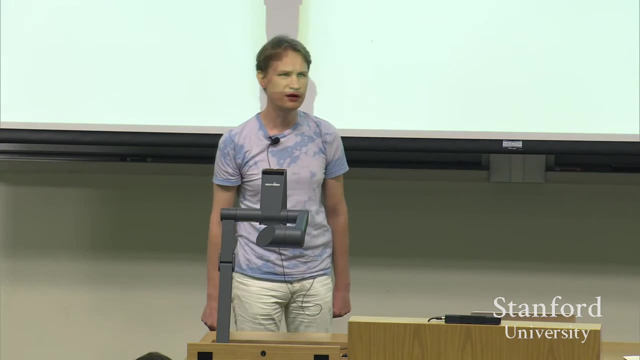 screen You can also. one of the things they've done is that they say: well, you know it's going to be hard for some blind people to immediately readjust to touchscreens, so we're going to give them a feeling as if they were using a tab key, So you can move through the. 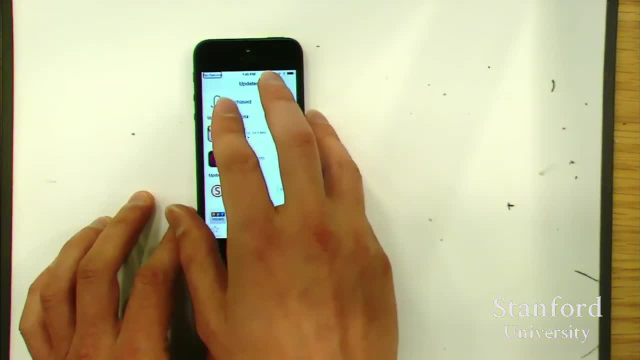 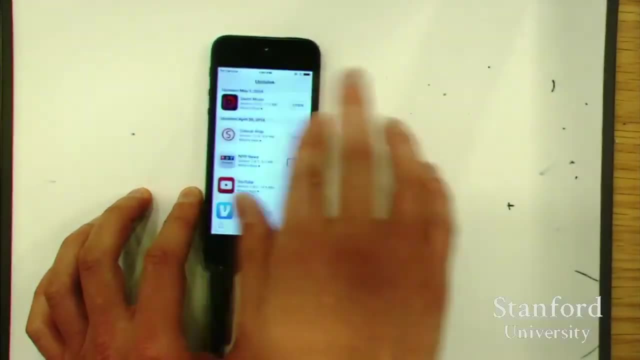 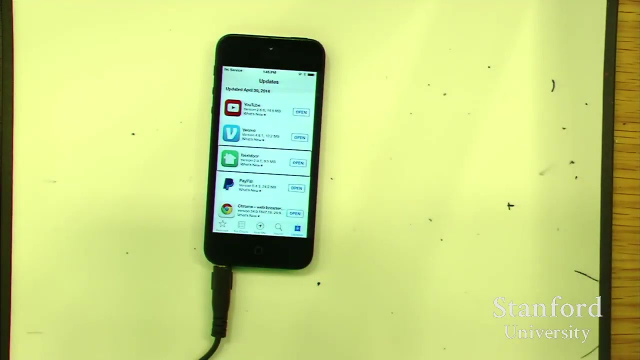 hierarchy on the screen by starting anywhere on the screen And just swiping: Open Beats News. Open Updated Sidecar. Open NPR. Open U2.. Open Venmo. Open Next door. It does take a little longer, but you know if you're in a hurry or if you're just exploring. 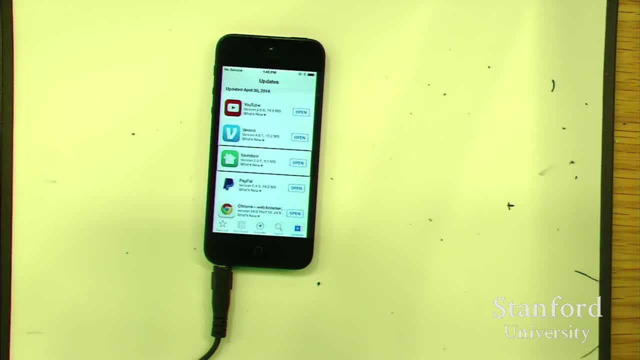 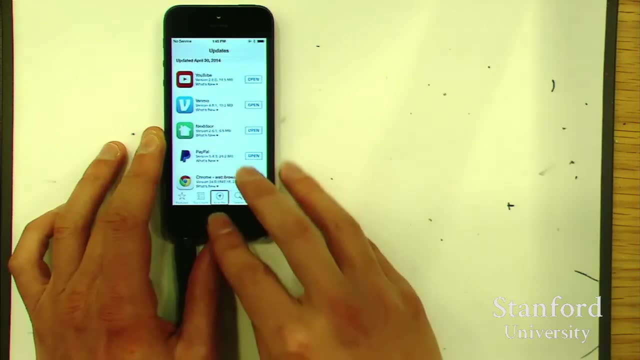 or if, let's say, you know you're not comfortable in using touch exploration, that's another way, So you can swipe right and left, Near me Tab, PayPal. Yeah, so I'm almost done iTunes store, And so the last thing I wanted to show you is that. so, as you can see, I have a little. 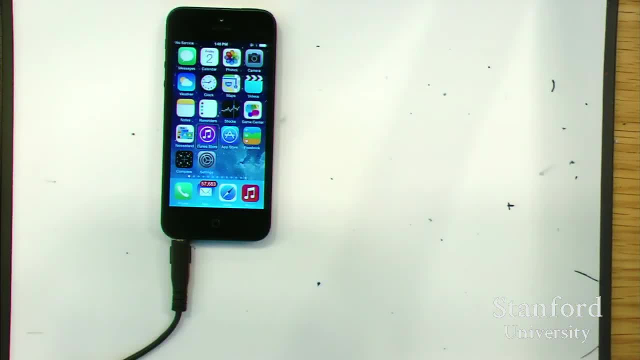 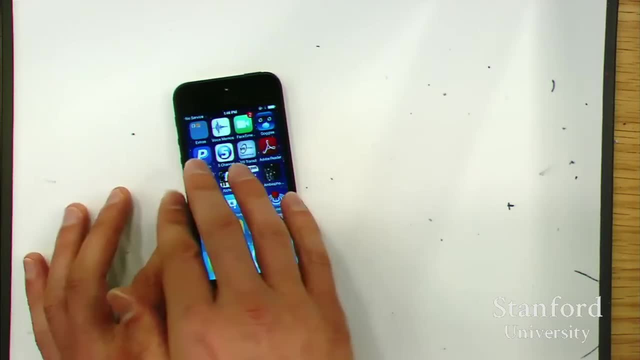 bit of accessibility. You can imagine all of the gestures, like single touch to you know, to hear double touch to activate. There's also, of course, you can swipe left and right, Extras, folder Messages And so on and so forth. 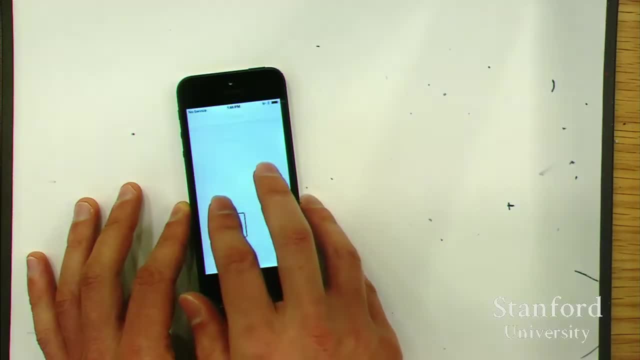 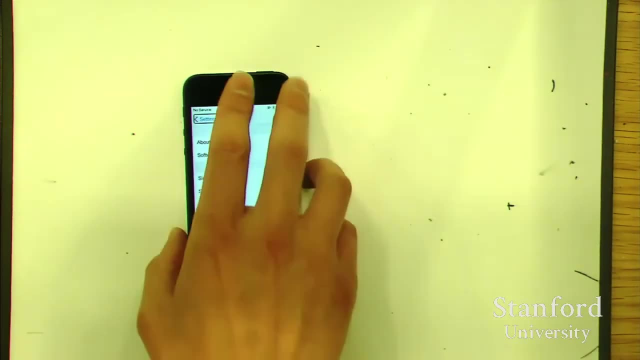 Page 1 of 13.. iTunes store Settings. And so last thing I want to show you guys is where to find this General Button, Because there is no reason why you guys starting HCI should know how to use these cool gadgets. 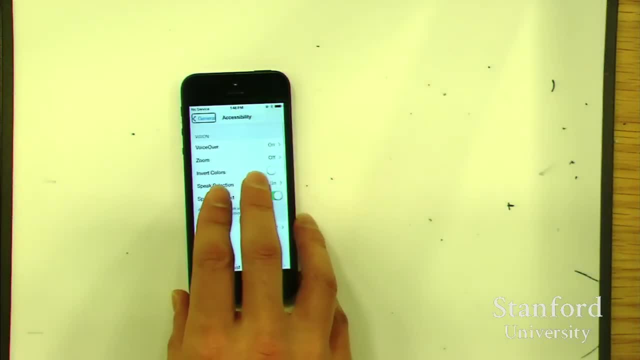 right Text size: Accessibility: If you go to accessibility- And I think I already mentioned 100 times, but I'll just say it 100- first is that it's built into every, every, every, every, every iDevice. Can you imagine Every Apple TV? 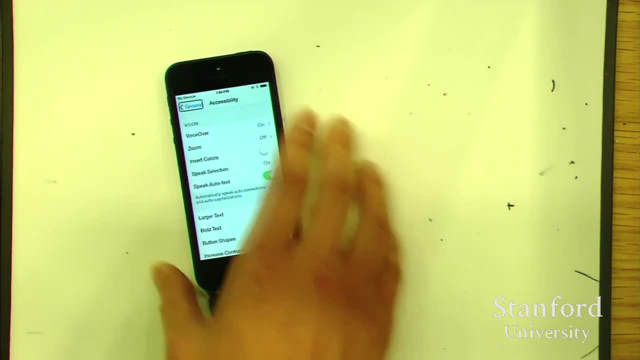 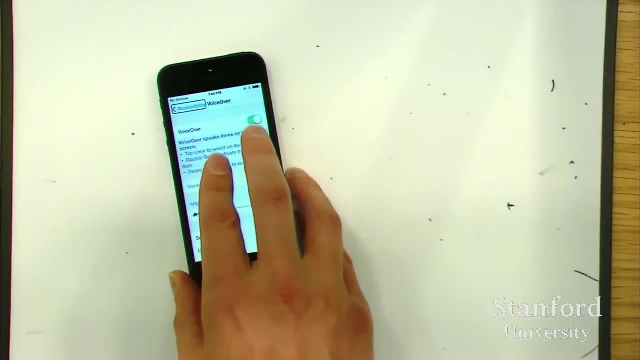 has something some kind of that. you know iPod touch and iPad and iPhone. This is where voiceover is. So if you want to learn how to use voiceover, you go here. That's it. It gives you very basic instructions how to use voiceover. 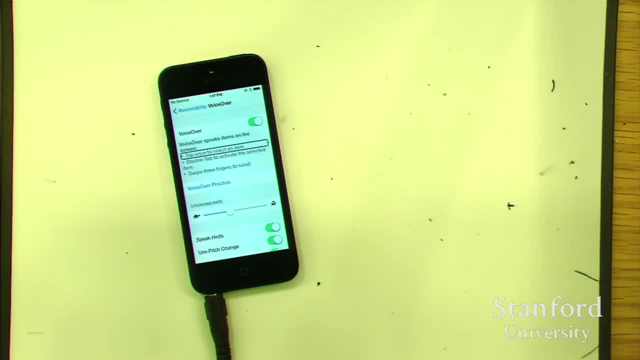 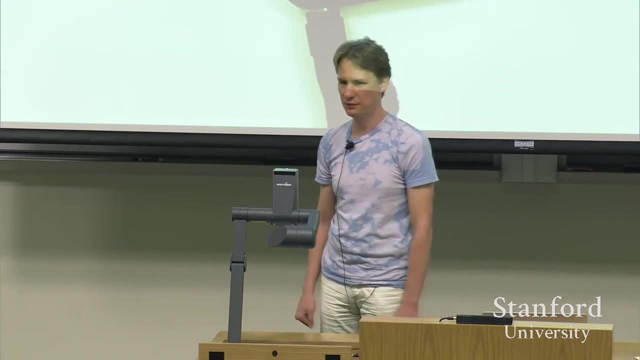 If you, if you're not comfortable getting yourself into trouble, you can always tell Siri: turn voiceover on, or turn voiceover off in iOS 7.1,, I think, or no, iOS 7.. And that always going to get you out of trouble. 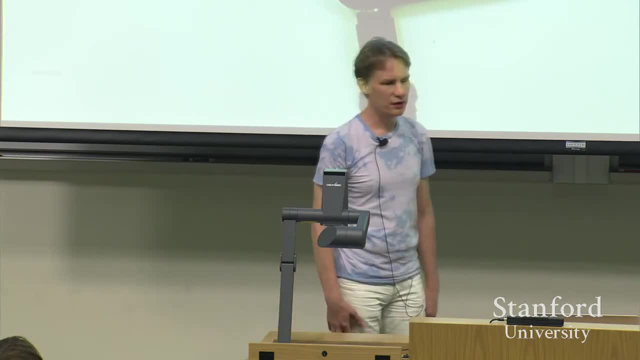 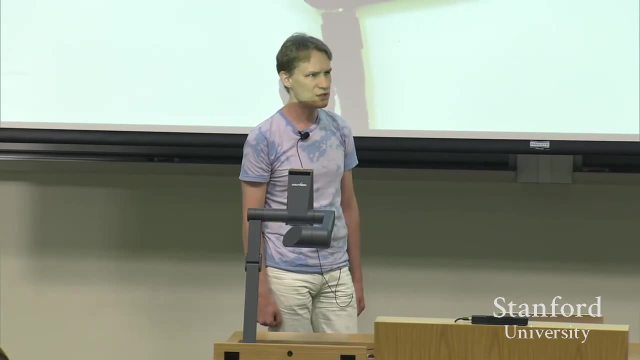 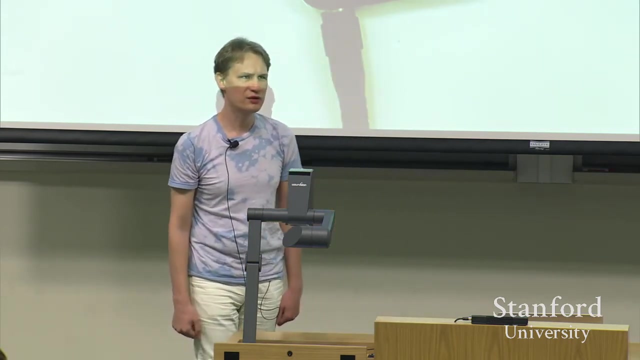 So, since you know, we talked about desktop, we talked about mobile phones, I want Ramya to come up and talk a little about the web, And the reason why we spend so much time talking about the web, Companies like Facebook and Twitter and PayPal- is because web is really our desktop of the future. 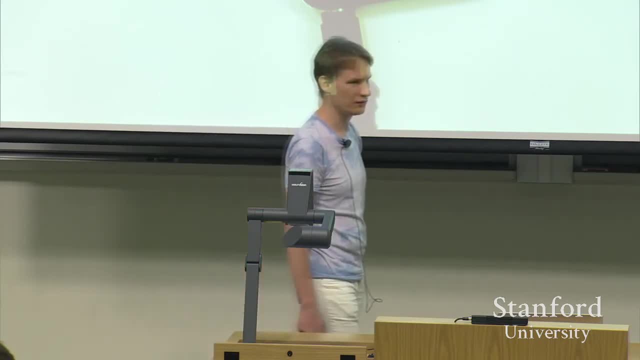 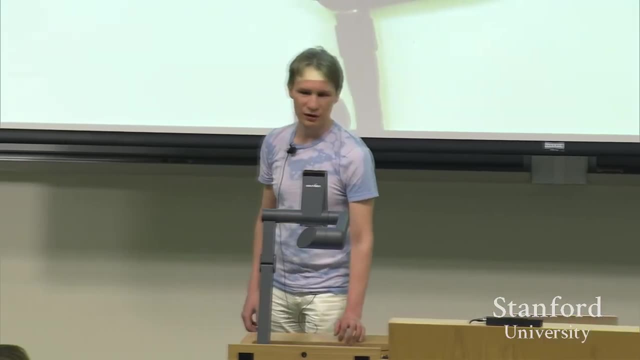 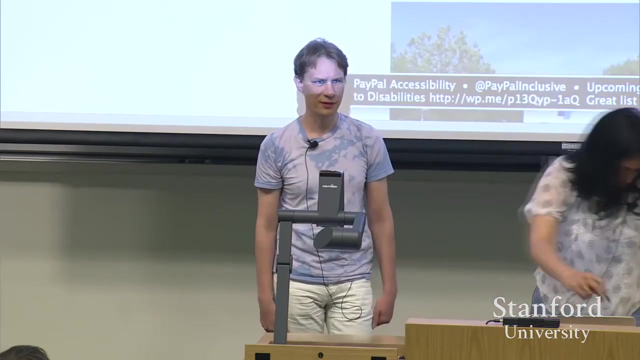 I think every battle that's going to happen- including the one with FCC, is going to happen- about the web right, Make the web accessible, keep the, you know, flow of information going, And the web is so important. So this is why it's so important for all of us to keep web. 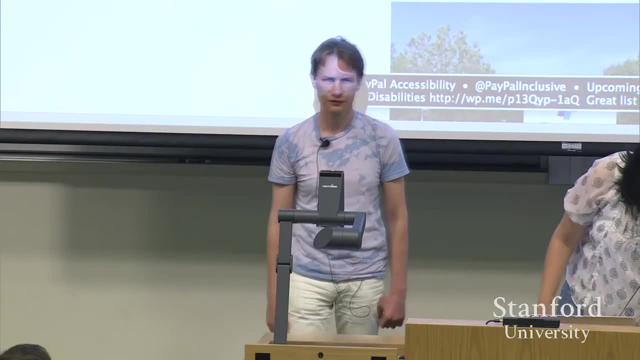 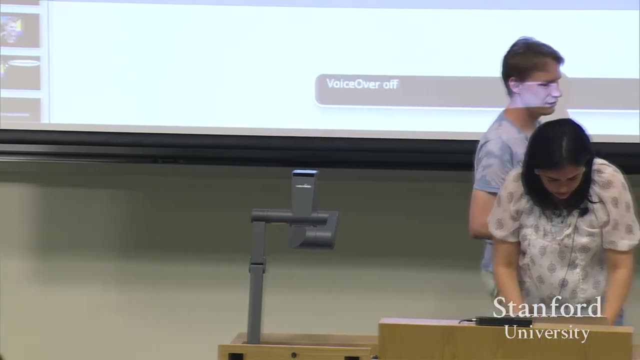 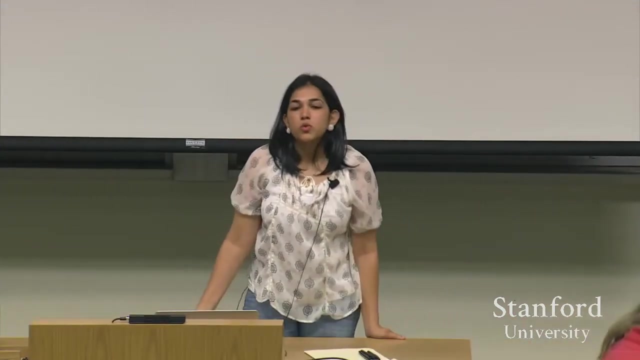 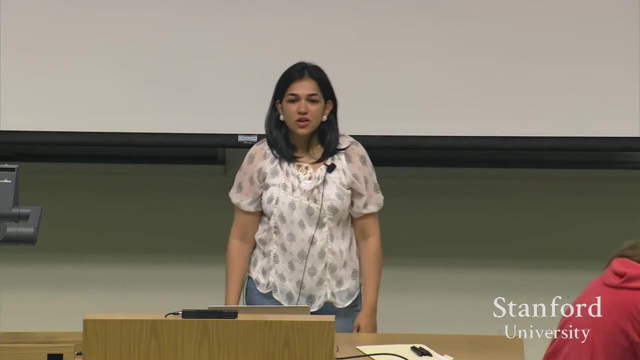 healthy and for you guys as developers, as people who design interfaces, to be doctors of the web. I'm going to begin with a small world story. Prior to working at Facebook, I worked at Stanford University as a web accessibility consultant in Scott Stalker's team. 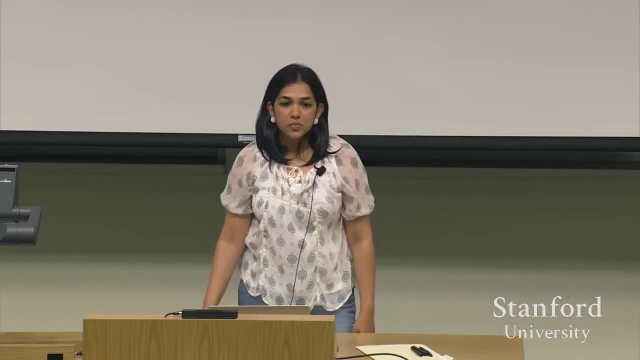 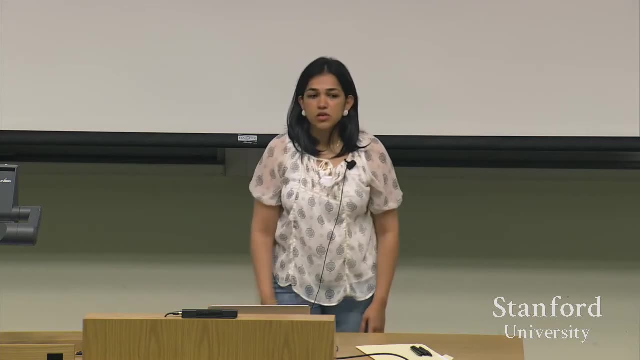 So I want to shout out a thanks to him for connecting us to the right people to make this happen, And I want to thank Michael Bernstein for letting us present here, Although None of us have our PhDs, So I'll try to talk super fast because we're running out of time. 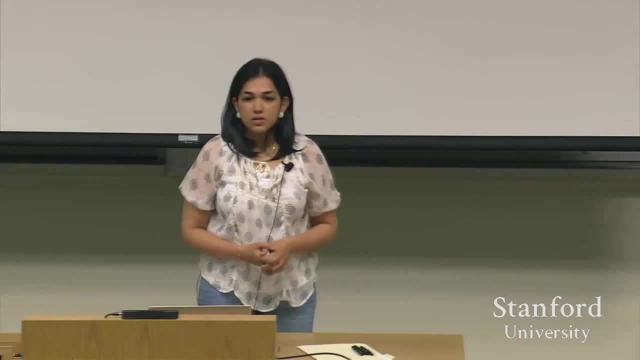 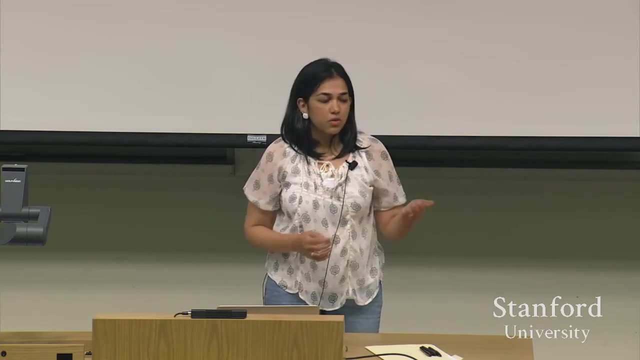 For the next five minutes, I'm going to give you all a crash course on web accessibility. You'll all be web accessibility experts at the end of five minutes. And then, since today is all about acronyms, we saw POUR and SOAP. 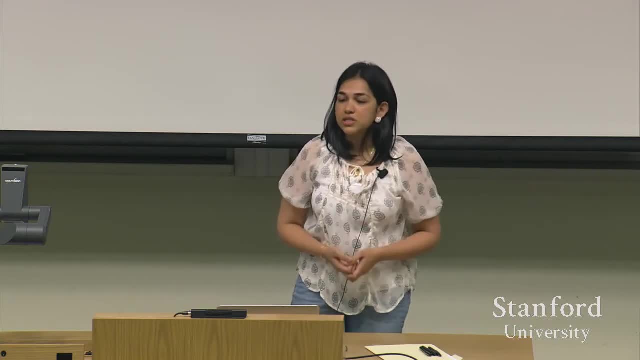 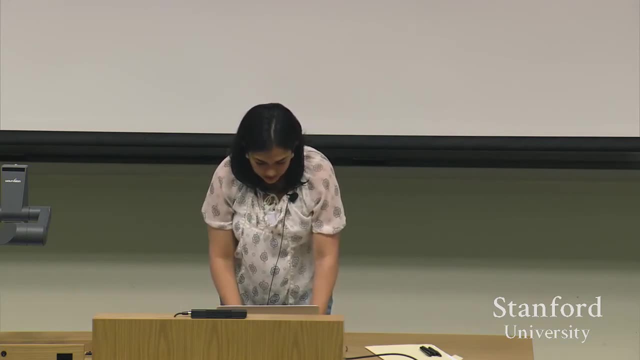 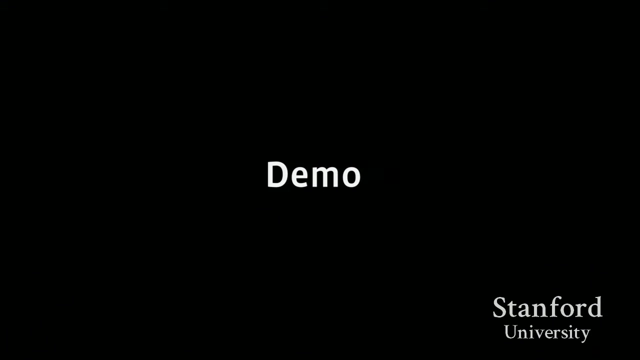 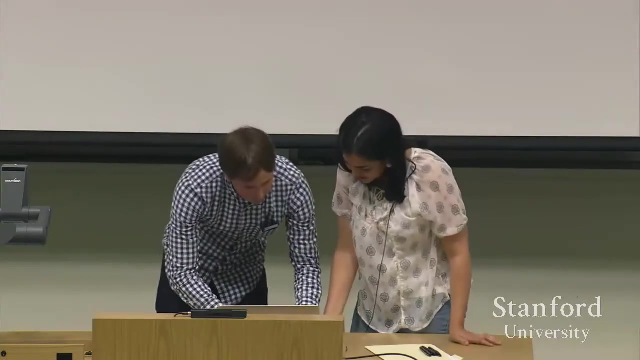 I'm going to leave you with an acronym which will help you recall all the basic principles of web accessibility. I'm going to try to do a live demo with voice, So let's see how this goes. Comment that to get to the, I think, while we're waiting. so you guys know that I remember repeatable, operable, understandable and robust. 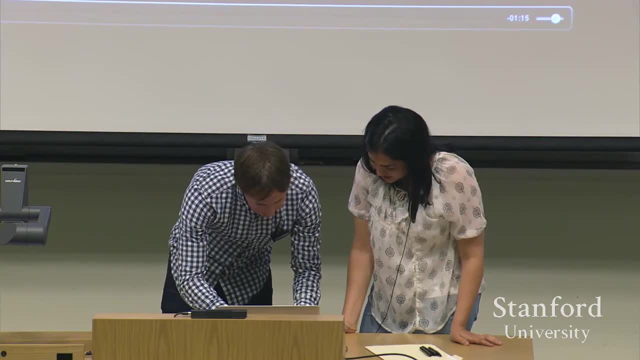 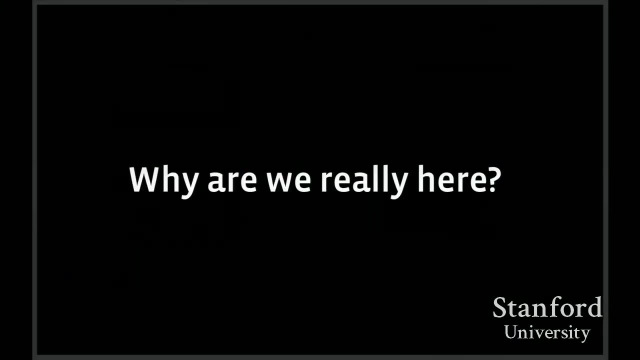 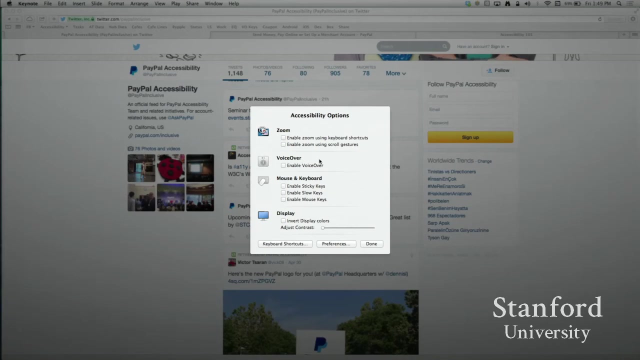 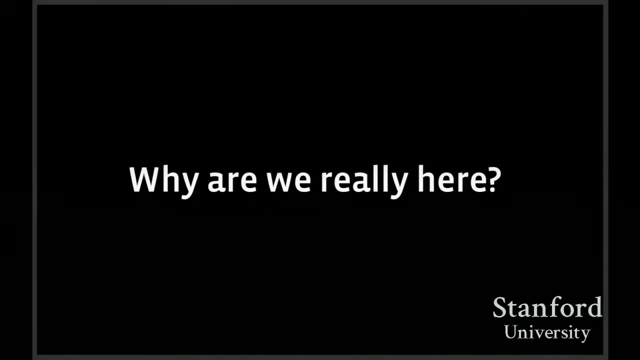 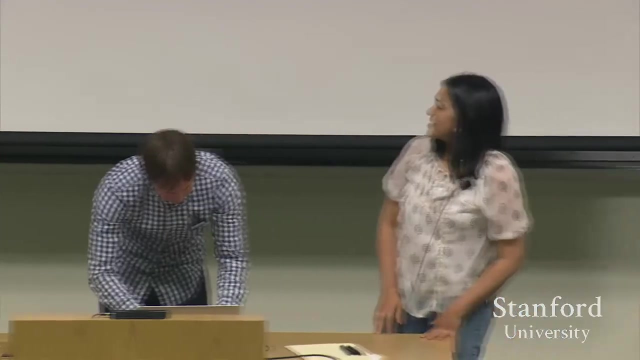 Yeah, as we are fumbling through this, yeah. 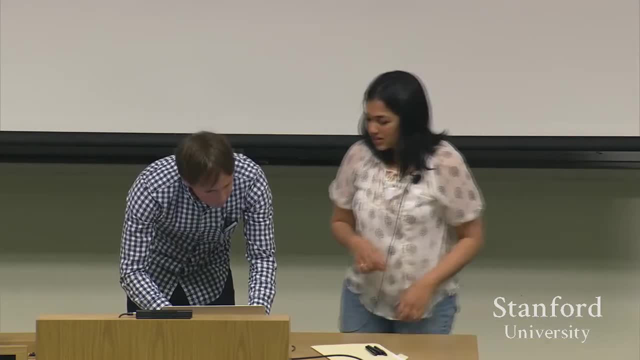 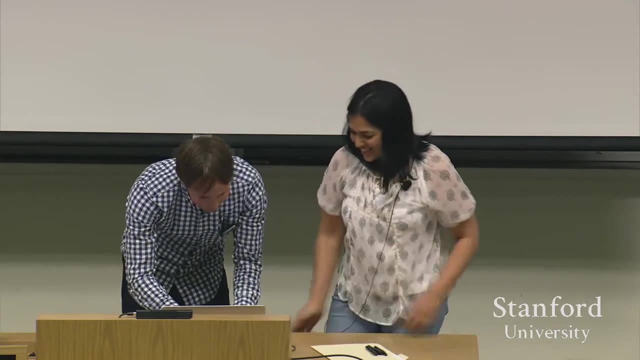 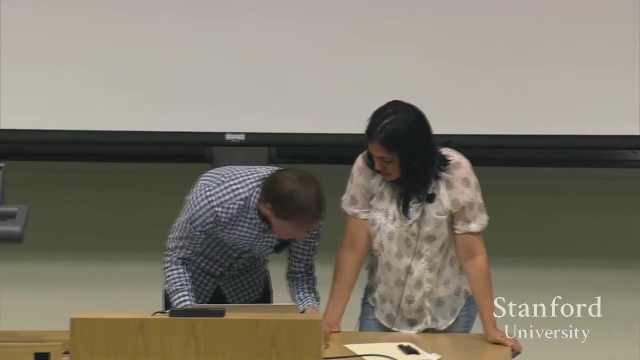 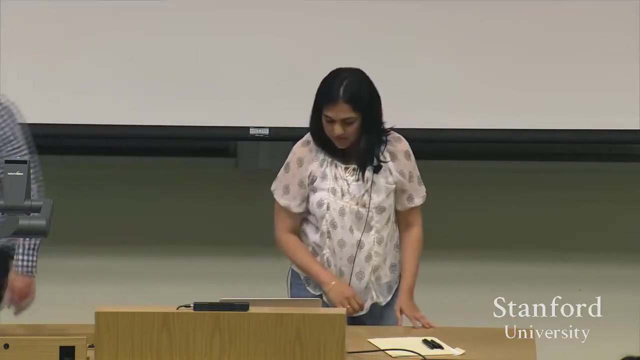 It's. we're just trying to jump out of Keynote and kind of: yeah, Now I'm a bit nervous about turning on voiceover. Okay, Welcome to OS. So far, accessibility 101, accessibility 101.. Okay, let's get started. 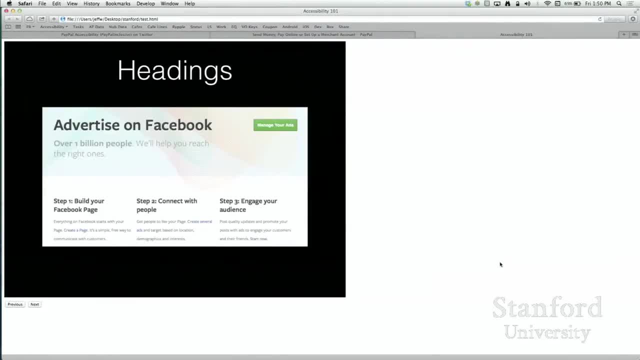 I'm going to walk you through the basic principles of web accessibility and also try to relate them to design. So I'll start with headings. We all understand why headings are important for visual design. They help visually organize the content in the website. 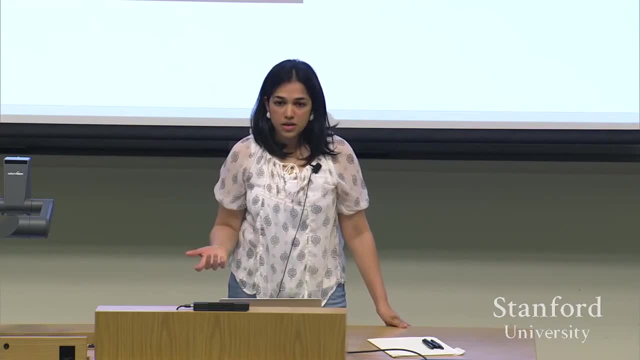 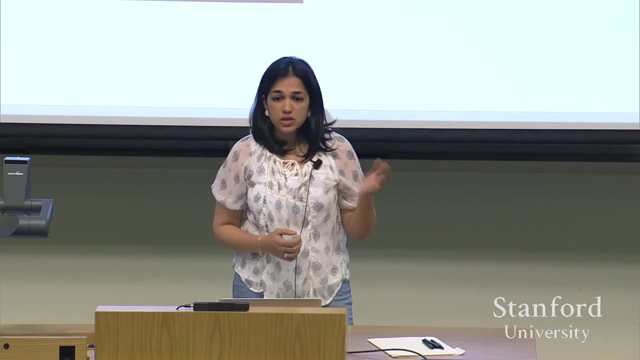 So it's really easy to glance at the headings and know what a website is trying to convey. But headings, as Victor demonstrated, they're crucial for accessibility, Because a person using a screen reader is going to try to get the gist of a website just by jumping through the headings. 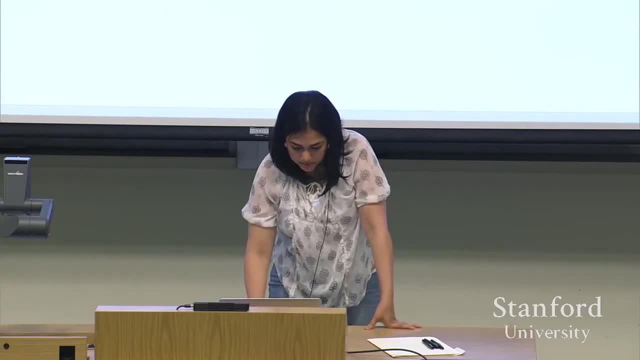 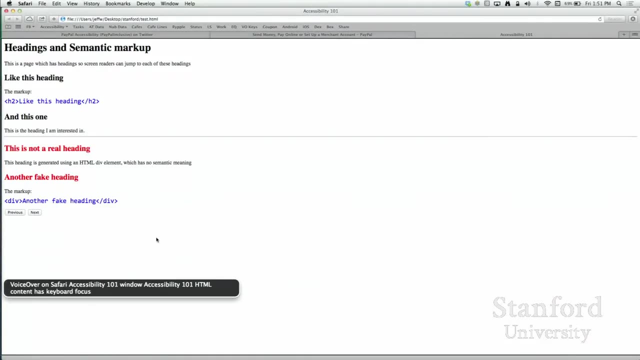 So let's take a look at that with voiceover. I didn't know Victor was going to do this cool demo with cnncom, but I'm going to Voice over on Safari. accessibility 101, window accessibility, Heading level one headings and semantic markup. 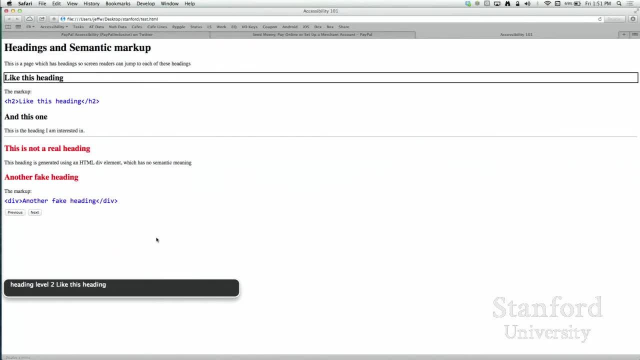 I'm just going to jump through the headings. Heading level two, like this heading. Heading level two and this one. Okay, the next two headings are marked up using divs and not semantic h2 tabs. You are currently on heading level two, inside of HTML commuting. 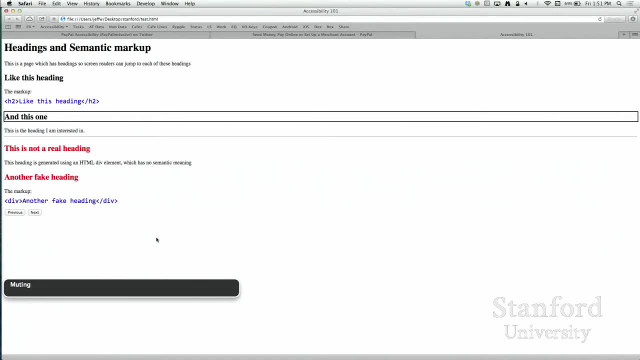 They're marked up with divs and not semantic h2 tabs And you'll notice that voice over skips these two headings: Last heading, heading level two, and this one Voice over off. So that's why it's really important to mark up with your headings with semantic. 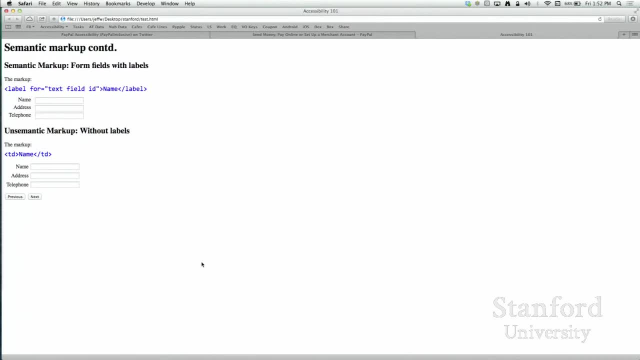 h tags. The next demo I have here is a semantics set of form fields. the first set of form fields: i've associated the labels with the form fields with semantic markup. that's a label with a for attribute pointing to the text field. and the next 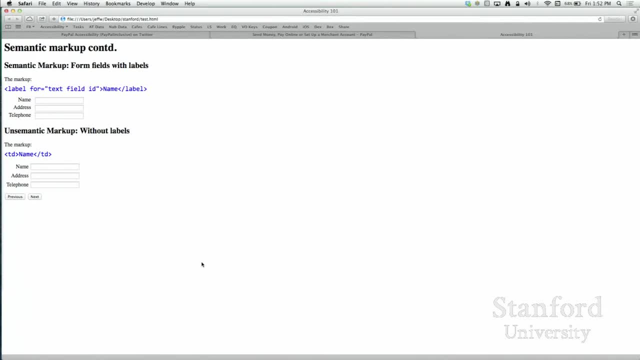 set of form fields. i don't have the labels associated with the text fields. that's unsemantic markup, so let's see what voiceover does with this voiceover on safari. accessibility 101 window. interact with. accessibility 101 html content heading level one semantic markup. interact with. 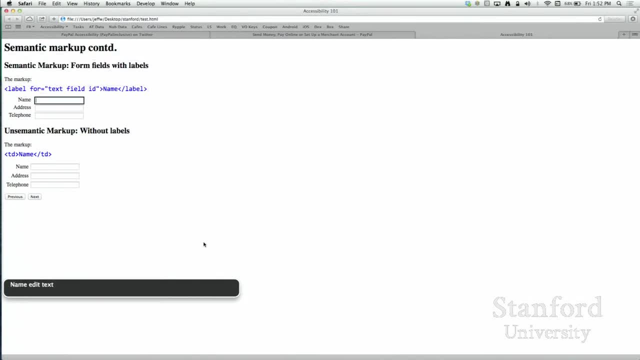 heading level one semantic mark head the name: edit text. okay, it announced the label for the field, which is name. you are currently on a text field inside of voiceover off. um, i'm trying to tap to the next field. so, victor, do i need to do anything to tap to the next text field? it's not tabbing. 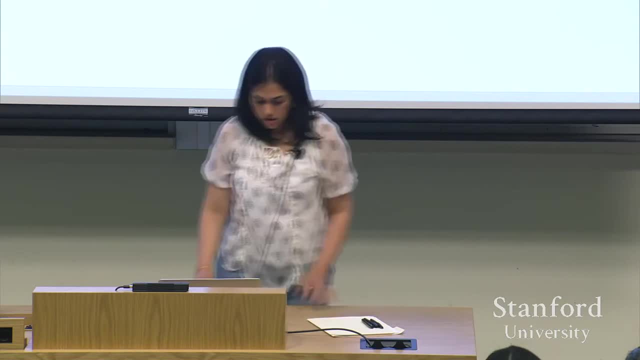 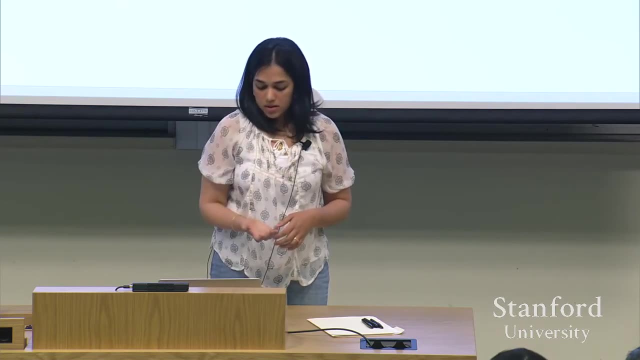 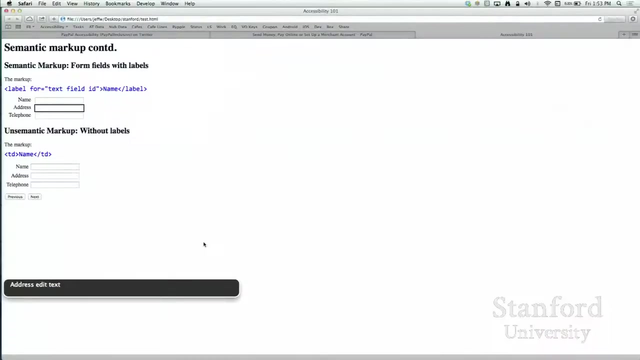 when i tap to it. okay, so the original demo was uh lot more obvious, because when you tap to the fields, voiceover will announce the name of the field. but i'm just going to try to move through each element now. um, voiceover on address. edit text. 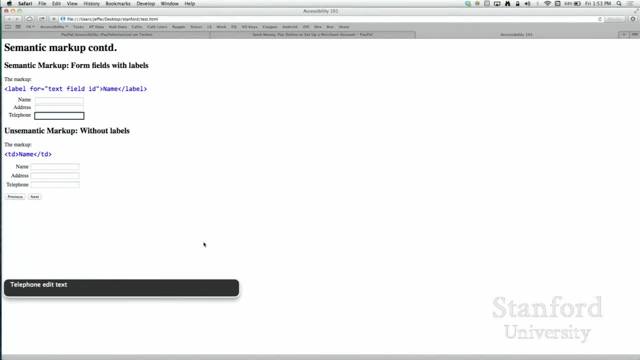 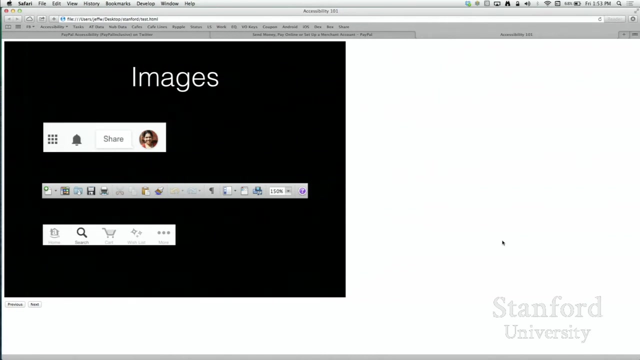 so voiceover announces the label, which is address: telephone edit text. okay, now i'm going to jump to the unsemantic markup. edit text blank. so edit text blank, edit text blank. so that's why semantic markup is important. um, voiceover off. jumping to the next principle, um, it's images and non-text content. i have here a few screenshots from: 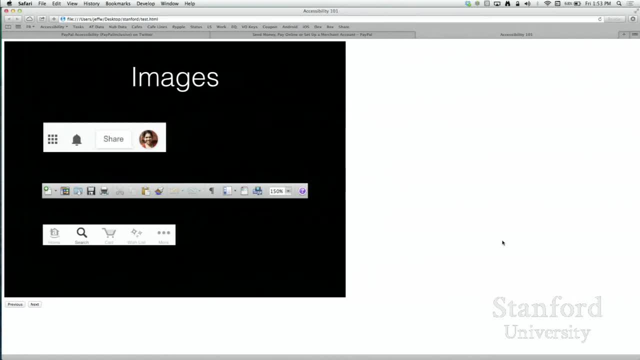 popular web applications like gmail and microsoft word, and the reason i've called them out here is it's not clear to me what these icons indicate until i activate them and look at the options in the menu. the third screenshot here is from the amazon mobile app. the icons are really clear and 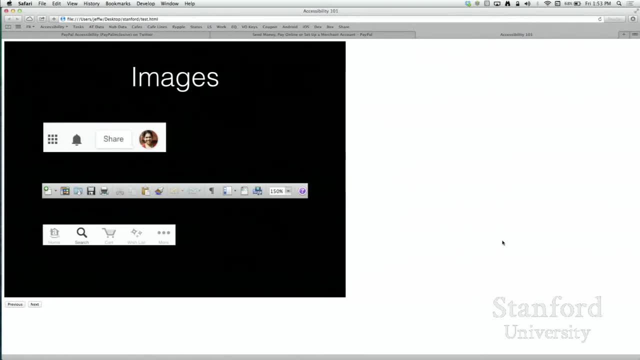 this text right below the icons, which makes it obvious what the icons stand for. now, if vague for a sighted person, it creates a really painful experience for someone using a screen reader, because now they would have to tap to the icon, activate it and then go through the list of. 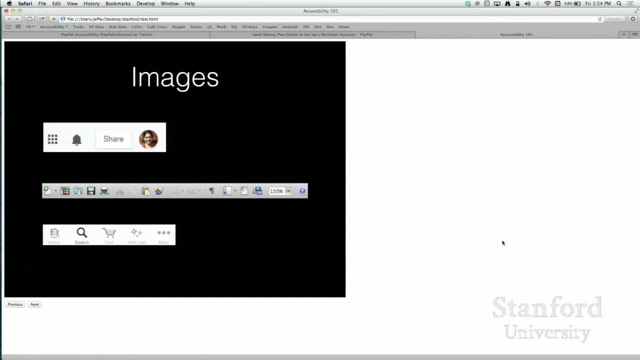 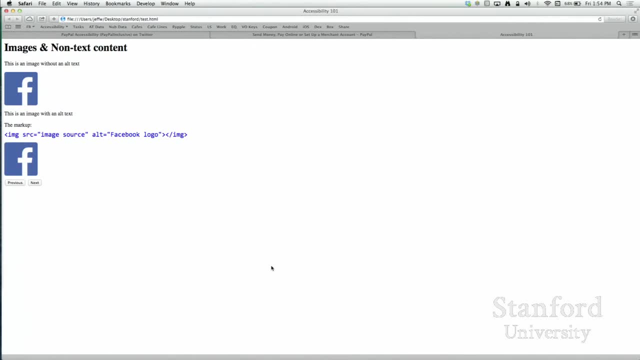 options in the menu to know what the icon is representing. so let's look at a demo. i have two images here. the first image: i've associated it with some textual description and i do this by using the alt attribute in the image tag, and the first image is with us. 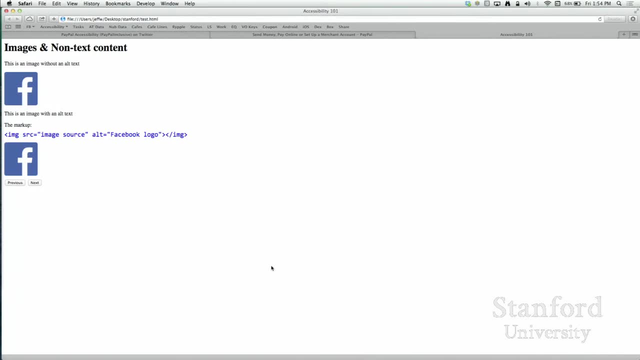 the alt attribute and the second image. i associated with an alt attribute and let's see what voiceover does when i navigate to these two images. voiceover on safari: interact with one, two, seven, one zero eight. four. underline one zero. one five. two, two zero three, one zero eight. 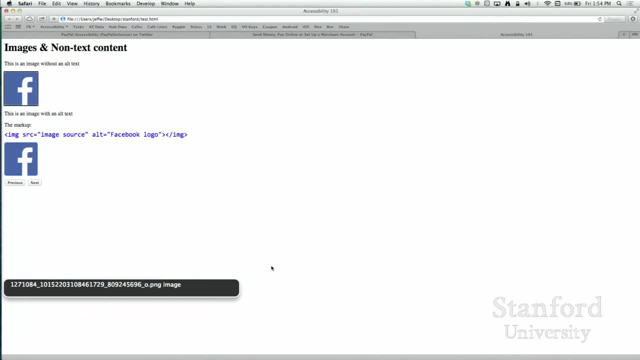 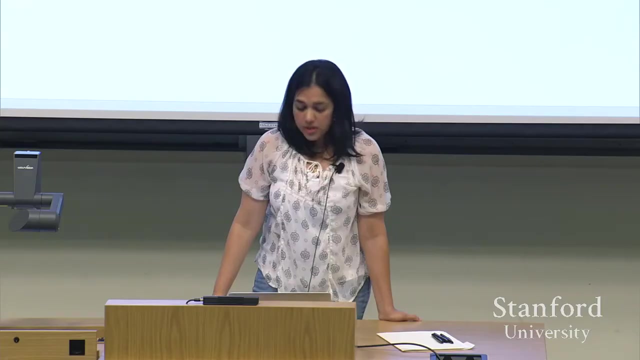 four, six, one, seven, two, nine. underline eight zero, nine. two, four, five, six, nine, six. underline nopng image. so that's an image without an alt text. the facebook logo image. voiceover off. okay, so that's short and sweet and this is an easy problem to fix most times, but this is actually. 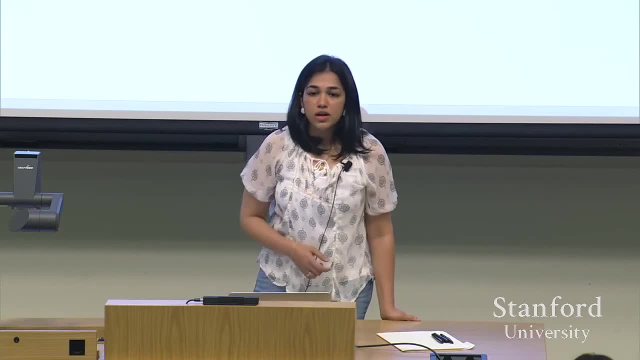 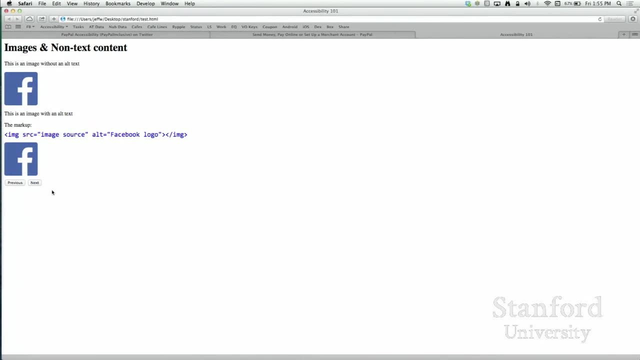 pretty prevalent on the web. there are a bunch of images that don't have all text associated with them and they are inaccessible to screen readers. okay, you hit the nail on the head, so i'm going to. i'm going to cover that towards the end of my talk. 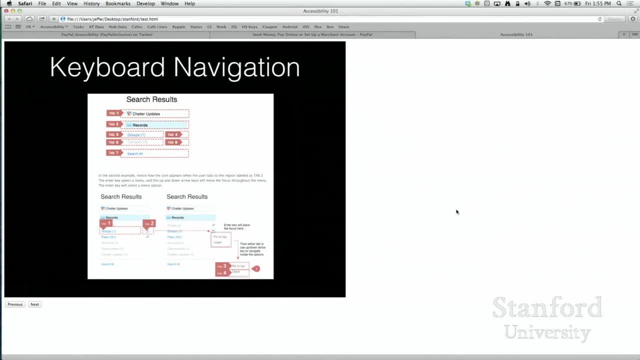 the third basic principle is keyboard navigation. what you see here is actually the screenshot of a design document from the salesforce blog. i thought this was interesting because it was a design document calling out tab stops and keyboard navigation. but keyboard navigation is also crucial to accessibility, because a person using a screen reader as well 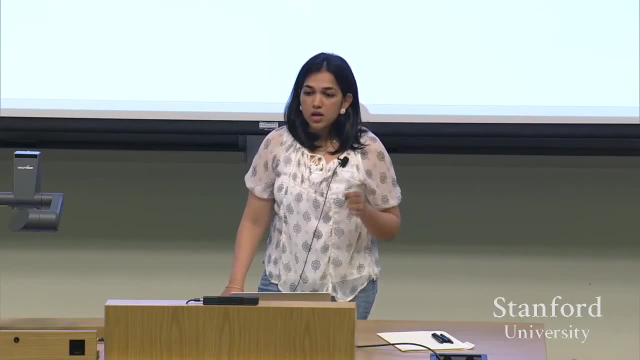 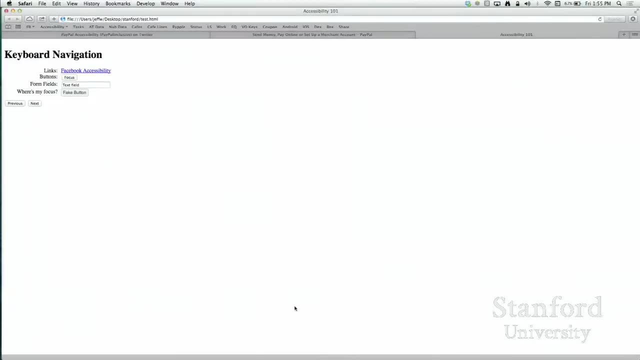 as those with motor disabilities, who cannot use a mouse, use just their keyboard to interact with elements on the page. so let's look at a demo of this. basic elements like links, buttons and form fields which are marked up with semantic markup, get keyboard focus by default when you tap to them. 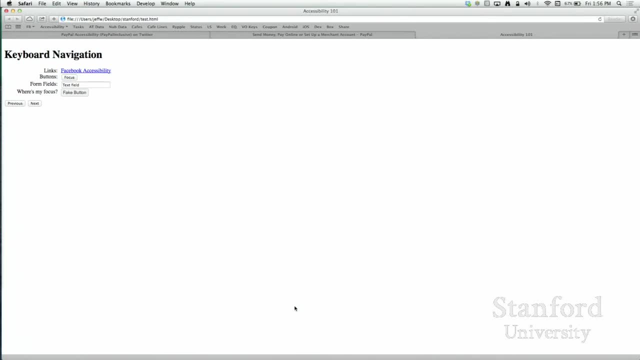 but things get interesting when you build custom widgets and they're built with unsemantic markup, like this fake button i have here. so let's look at this voiceover on safari: interact with accessibility once your link focus buttons, button text field contents, selected form field text: fake button clickable. okay, voiceover off. this demo did not work because i was supposed to tap to the. 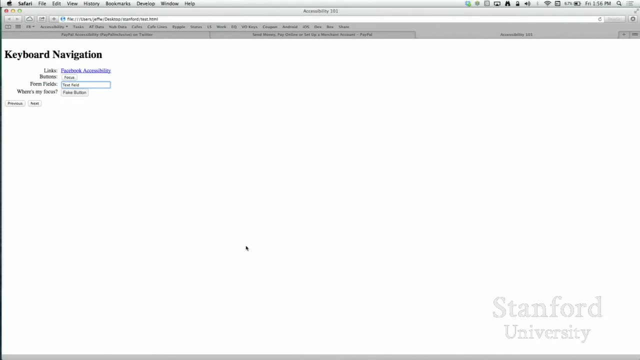 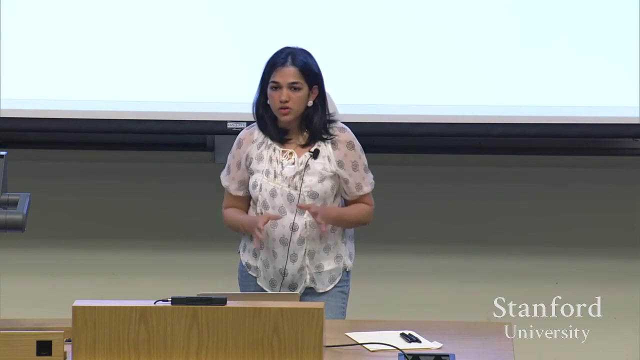 button and voiceover would not have tapped to it. but something is broken with the tab navigation right now, um, and so it did announce the name of the button. but, um, if you actually build buttons with just divs or spans and you try to tap to them, the screen reader is not going to tap to. 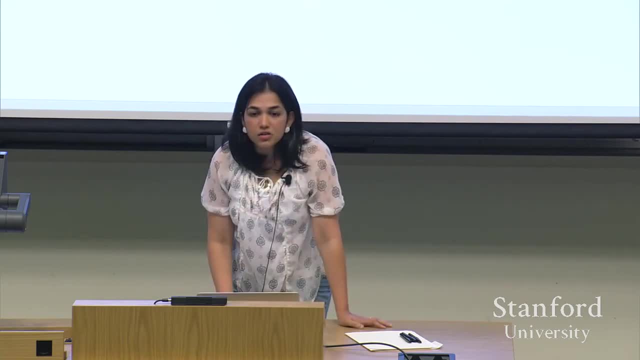 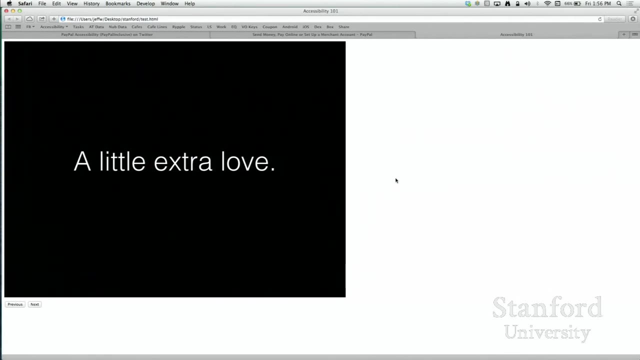 those elements and we'll see in a few minutes how to make this fake button accessible, but before that, my last principle, which is a little bit of love, is that when we want to make a user experience accessible for users, we have to meet the user's expectations, and the same is true for accessibility. in addition to focusing on headings, 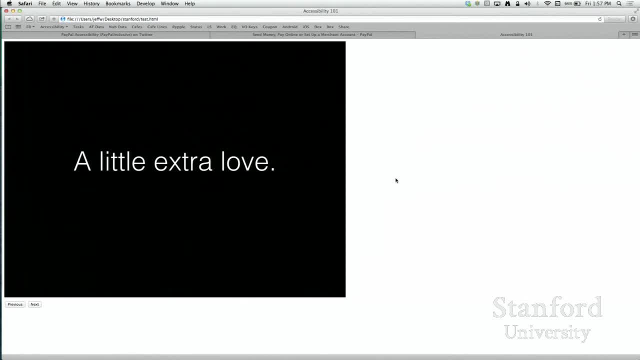 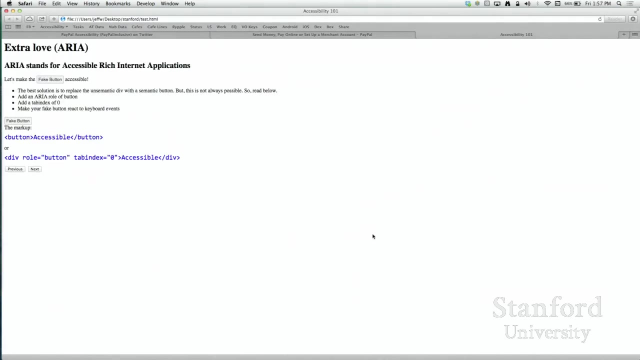 keyboard navigation and non-text content. we also have to augment our html document with some additional attributes that convey this extra information to screen readers, and that is done with aria. aria stands for accessible, rich internet applications, and this is one of the reasons that we want to make this aria accessible for the screen reader, because it is an html document and it's a 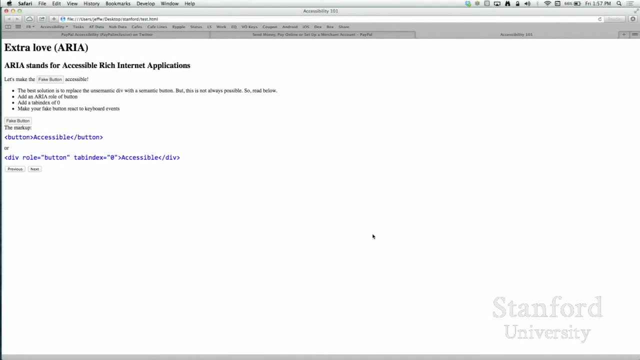 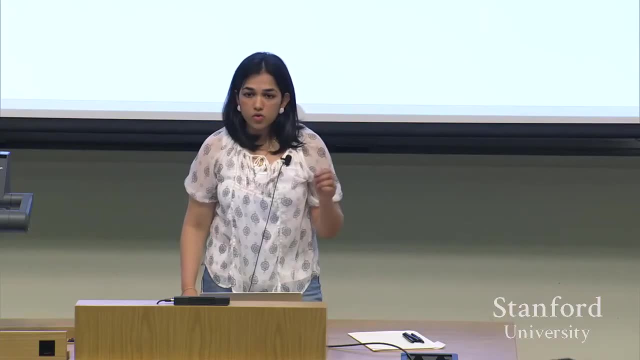 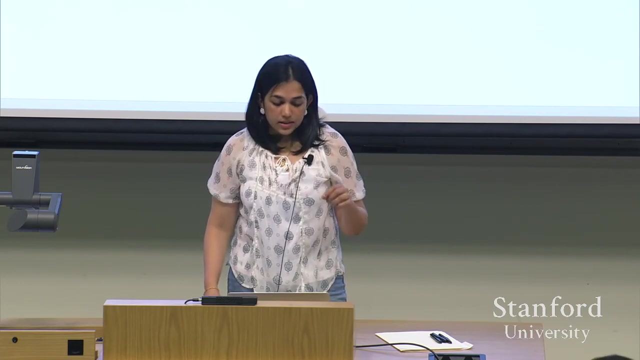 set of role, states and properties that you can associate with an html element to talk to the screen reader. so for, in order to make this fake button accessible, i would actually give it an aria role of button. this tells the screen reader that this element is actually a button to make it. 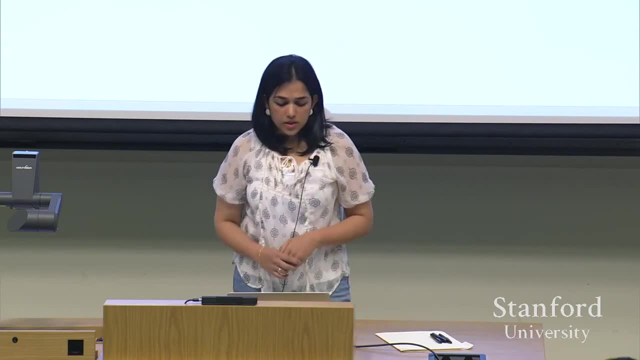 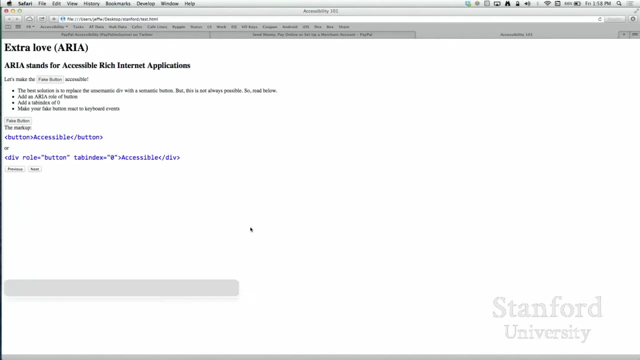 get tab focus when you tap to it, i need to add a tab index of zero to it with keyboard events, just like it does with mouse events. so let's take a look at this over on Safari with interact with accessibility and fake button button. okay, you are currently on a button inside JavaScript. what I only 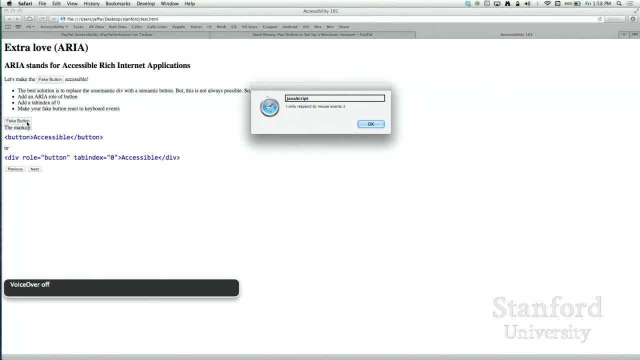 respond to mouse events. frown, I was supposed to show you that when I pressed enter with a keyboard, but something is messed up with the keyboard navigation so I had to use a mouse to click it. so I cheated. but you would have seen this nice dialogue if it had worked with just the keyboard. getting back to 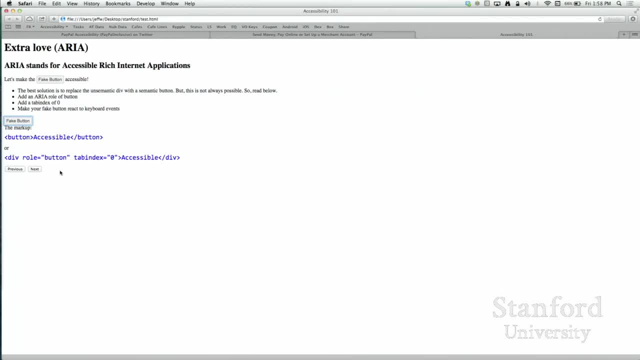 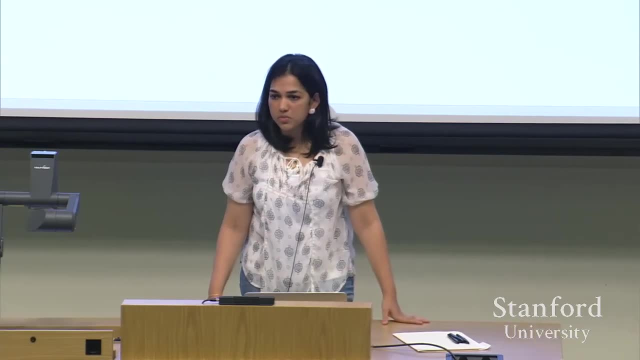 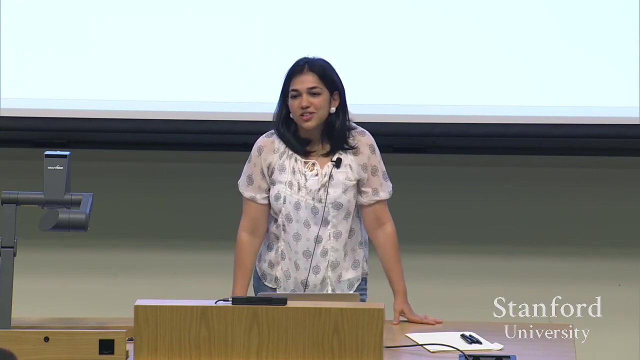 Michael's question. our jobs would be really easy if all accessibility problems were as simple to fix as we saw in these few examples. but we often run into situations where you have to be a bit clever about finding solutions to your problems, and I wanted to show you an example of where 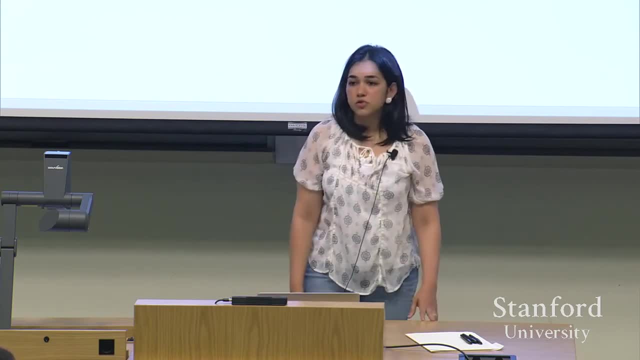 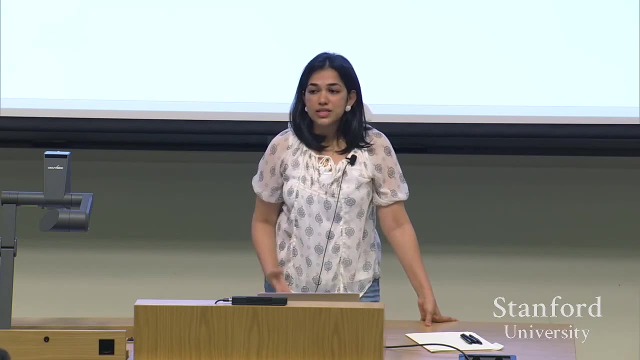 we've done that, and that is with Facebook photos. we have billions of user-generated photos from people all around the world on Facebook and we can't force people all around the world to always enter a caption or an alt text for their photo. so to solve this problem, we built something called the caption. 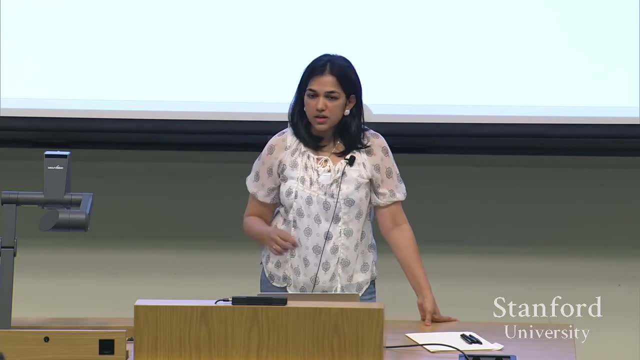 generator. the caption generator takes bits of metadata associated with a photo- who uploaded the photo, where was the photo uploaded, who are the people tagged in the photo- and it generates a caption or an alt text for the image, which we then associate with the image. so when VoiceOver lands on. 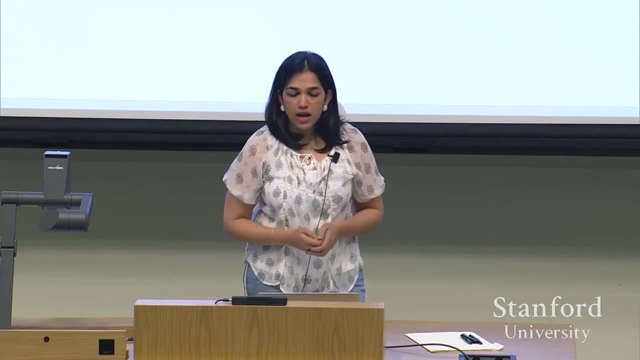 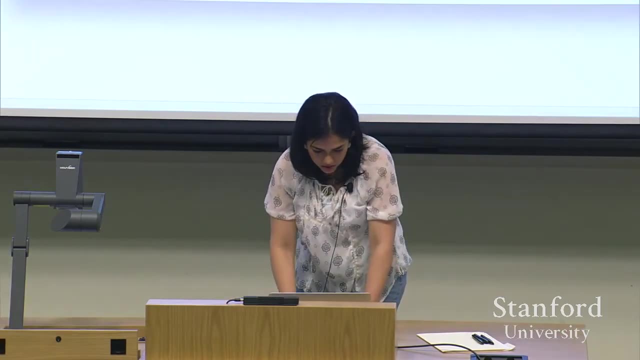 the photo. it announces this nice caption for the photo and I don't know if you have time for the video. okay, so let's take a look at the video showing tampa 況 voiceOver, interacting with our photos. you'll notice that we didn't Оpere. 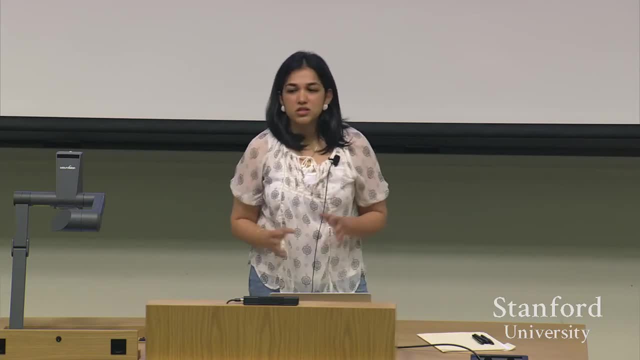 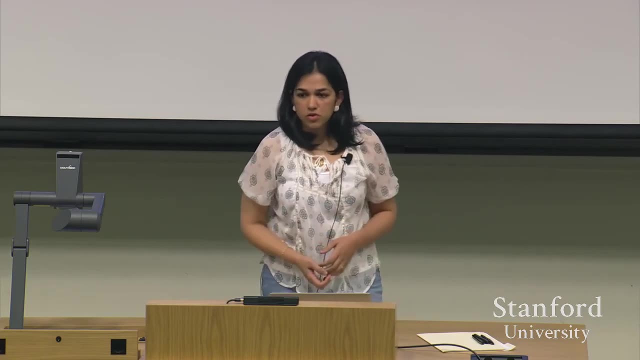 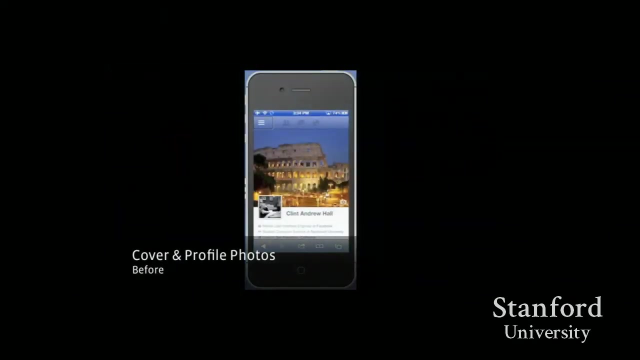 Notice that before we apply the Caption Generator, VoiceOver announces something generic like link image when we tap to a photo, And after we apply the Caption Generator, it announces a much richer description for the photos: Link image, Link, Link, Link. 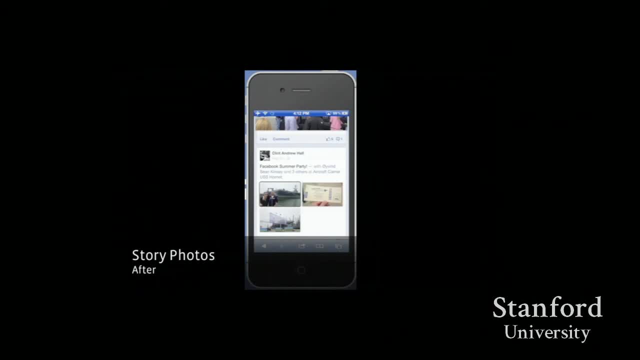 Clint Andrew Hall's photo of Clint Andrew Hall and Arjun Wurtsler taken at aircraft carrier USS Hornet, entitled On the Dock Outside the USS Hornet- Such an Amazing Place. Link image: Clint Andrew Hall's photo taken at aircraft carrier USS Hornet, entitled On the Dock Outside. 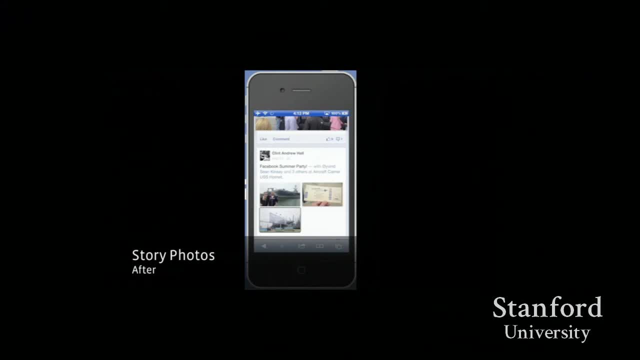 the USS Hornet entitled Outside the Party. Link image. Clint Andrew Hall's photo taken at aircraft carrier USS Hornet entitled A Passenger Receipt was a Nice Touch. Everyone kept asking if the barcode was real. Link image. Okay, that's all I had. 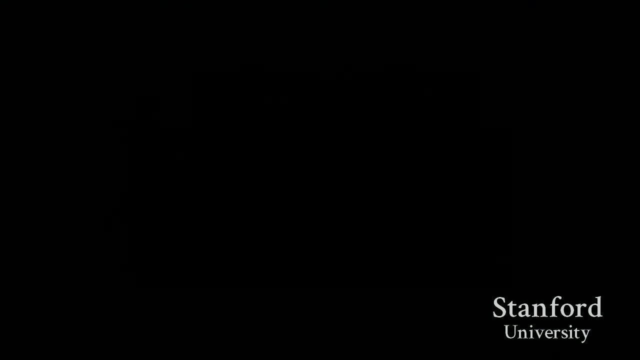 I'm now going to hand it over to Jeff, who's going to talk about making accessibility mainstream. Okay, Thanks, This is your call If you want to do five minutes of questions, or people can stay after. Do you guys have questions? 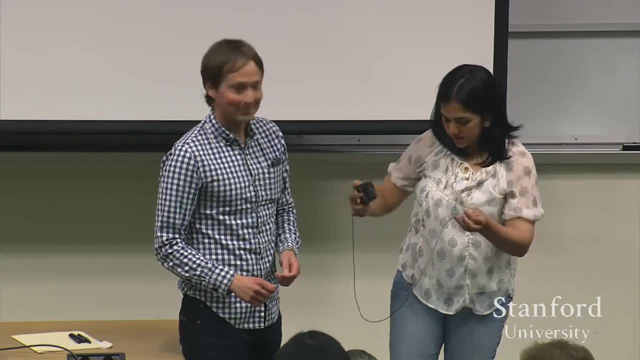 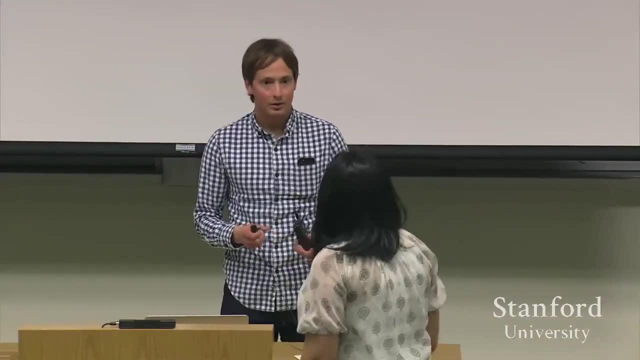 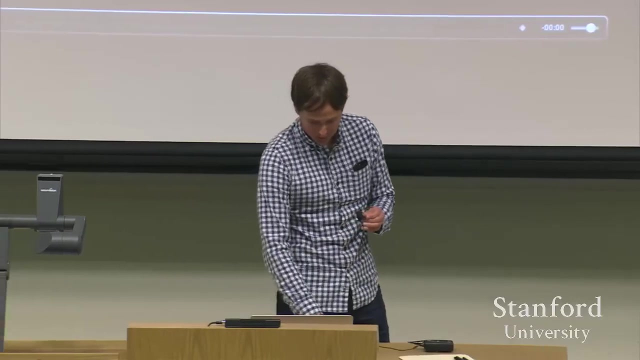 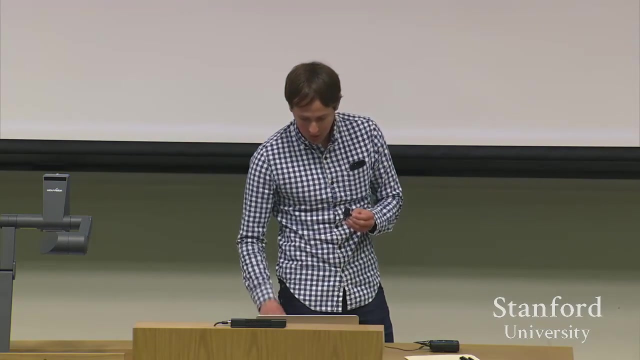 Yeah, I'm happy to field some now. Sure, Okay, So the presentation is supposed to end with a couple quick stories, and let me just give you one quick story. then I want to try to answer this question, which is: why are we really here? 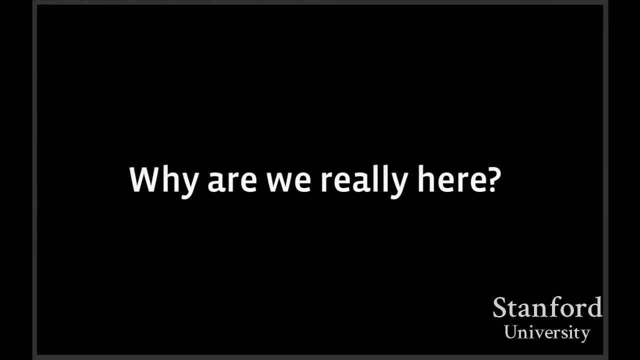 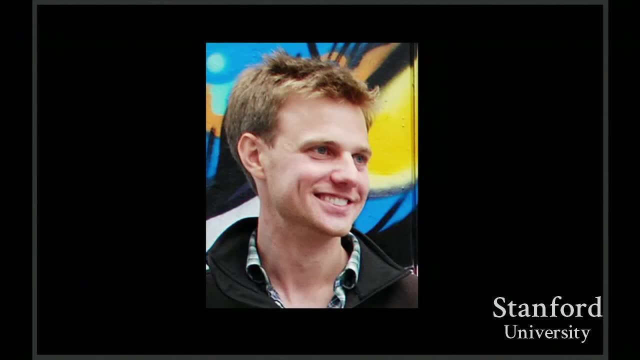 Why was Facebook and PayPal excited to come to Stanford and talk about accessibility? And the story that I think captures that best is a story that starts at Facebook. So I want to introduce you to a front-end engineer named Jason. He is in his late 20s. 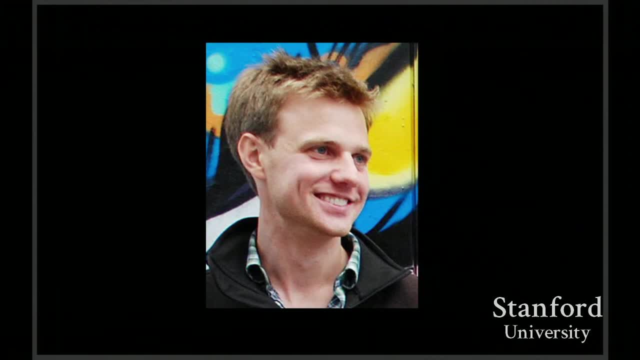 He graduated from Carnegie Mellon University. He's about to get married in two weeks. He's a very nice guy. He was working on a product called Web Messenger- Web Messenger- if you use Facebook in a desktop browser and you send messages. that's Jason's. 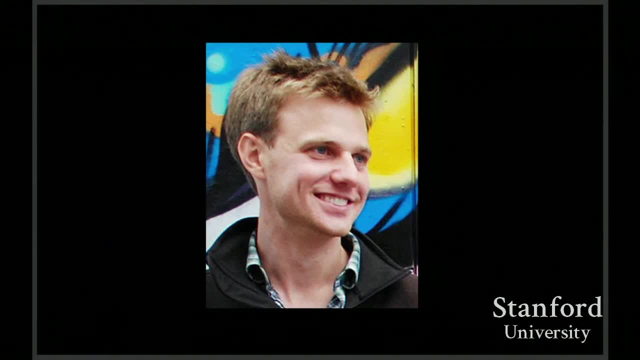 product. So when he was working on Web Messenger about a year ago, we were doing a large refresh to this product, I noticed that there were going to be some challenges with it in regards to accessibility and compatibility in a screen reader. So I reached out to Jason and I asked him had he tested his product for accessibility. 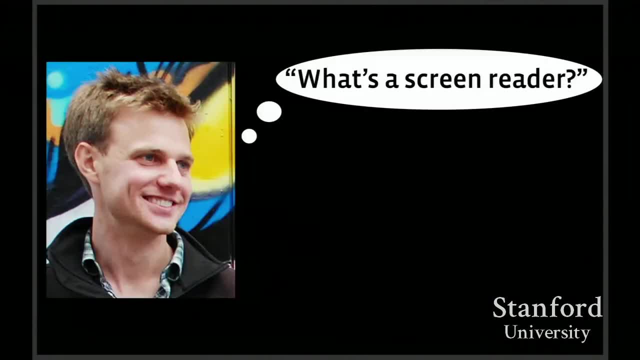 Had he tested it in a screen reader? Jason's response was: what's a screen reader? This is sort of the dreaded response that you get as somebody who's working in accessibility. When you reach out to an engineer and you ask them, you know, are they working on accessibility? 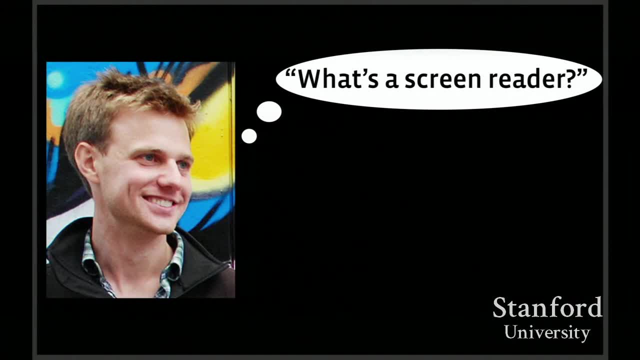 for their product And their response is: I really don't know anything about accessibility or what a screen reader is. So, despite the fact that Jason had graduated from, you know, an outstanding engineering program, had passed the technical bar to work on Frontend at Facebook, he had no exposure. 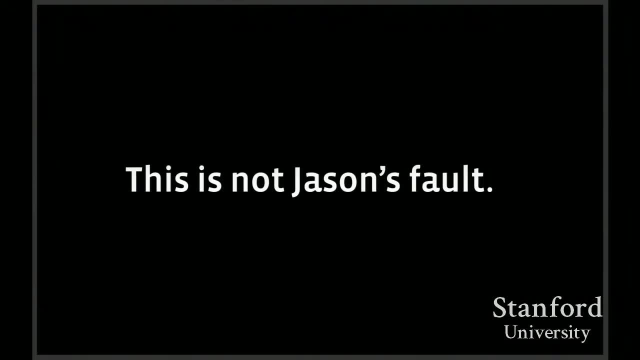 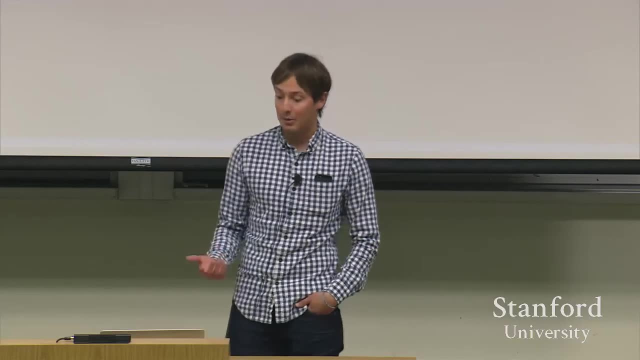 to accessibility And I'm not here to push Jason under the bus. I really don't think this is Jason's fault. In fact, there are most of the engineers that we work with at Facebook have a similar experience as Jason: They've not been exposed to accessibility. 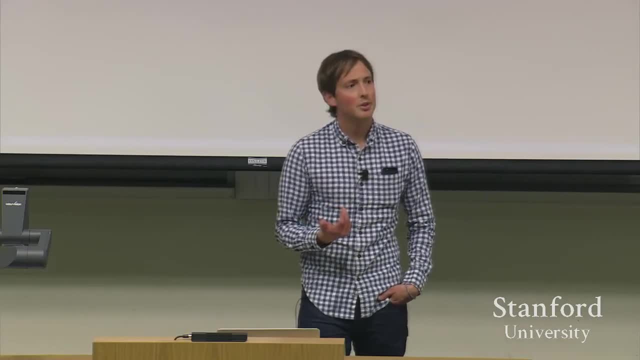 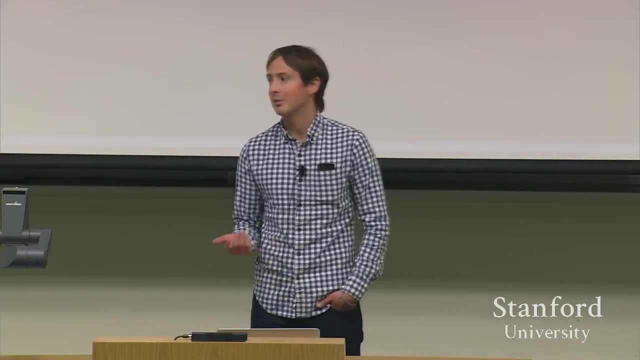 They've not been exposed to accessibility in their training, And so I think it's a little bit difficult for us to expect that the web is going to be accessible if the people who are building the web don't have much understanding about accessibility. So one of the reasons why we were really excited to come here was just to connect with students. 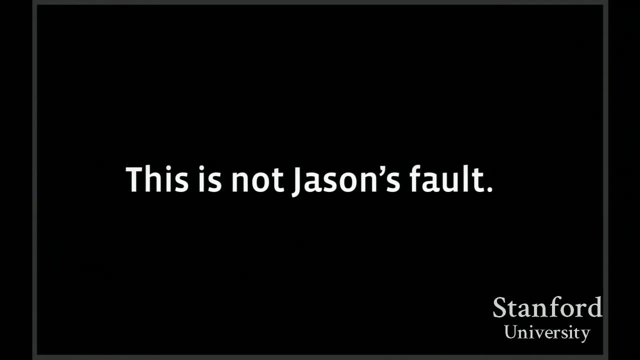 like you guys working in design and HCI and computer science who are ultimately going to build the future web and build future products. We want you guys to know earlier in the process, you know in your life cycles as developers and as creators, about accessibility so that you can demand it from the products that you're 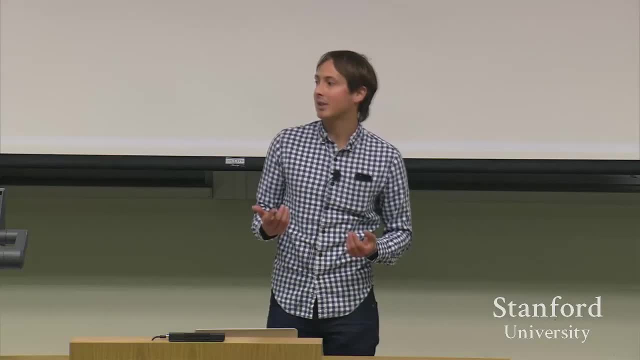 building and you know what to do. You have some best practices. I know that Ramya moved pretty quickly through some of the HTML demonstrations, But I forgot the word. The acronym for the code is HIGH, H for heading, H for images, K for keyboard navigation and E is extra low. 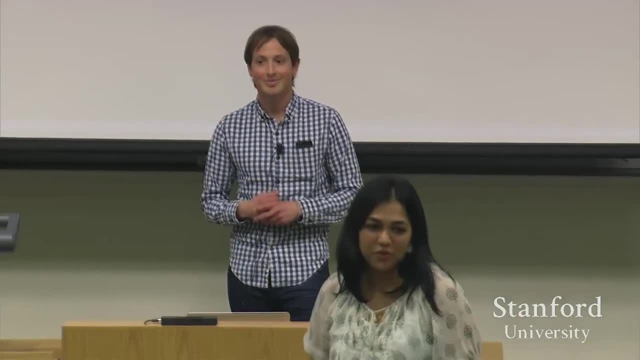 So that's the acronym. But Yes, and just remember HIGH Next time you are, you know, working with a web team or building a web product. That's like I don't know, I don't know, I don't know. 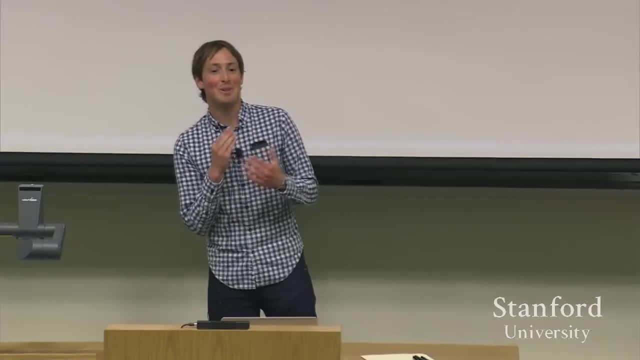 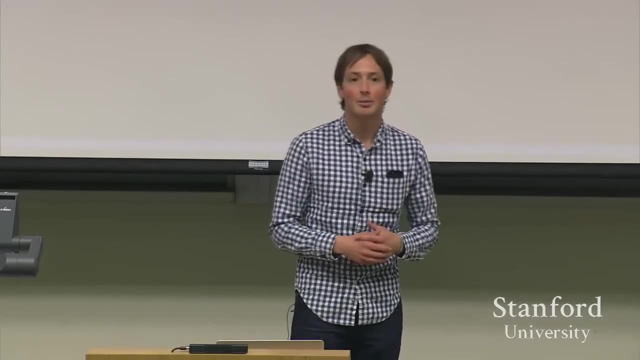